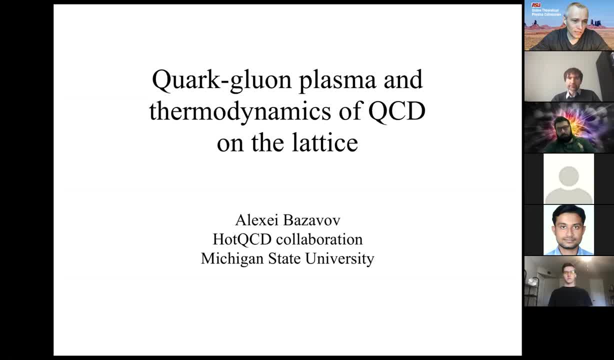 Since 2016,, he is a faculty member at Michigan State University. He has diverse research interests in finite-temperature field theory, lattice-gauge theory with applications to particle and nuclear physics, parallel algorithms, molecular dynamics algorithms, inverse problems, Bayesian inference, ultra-cold atomic systems, quantum simulation, effective field theory. 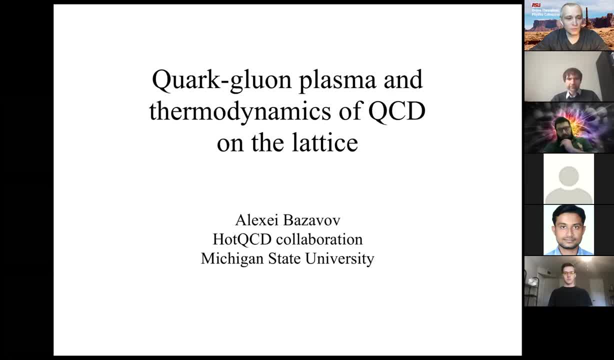 wide research experience, and today he will be giving a talk about cool-gluon plasma and thermodynamics of QCD on the lattice. So with that I'll give the microphone to Alexei. Okay, thank you very much for the invitation and the nice introduction. So it looks like you had a look at my web page. That's a nice letter. 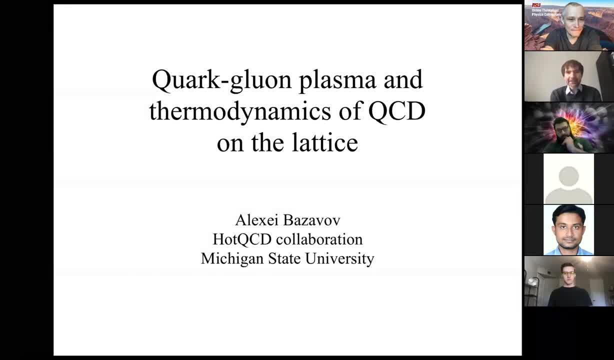 So I will discuss certain aspects of the work which spent roughly the last 10 years- and there have been, of course, many things, but I'll focus on things which I consider the most important and interesting. I can cover everything, obviously, and I will try to keep the level of technical details to a minimum, except for a couple of places. 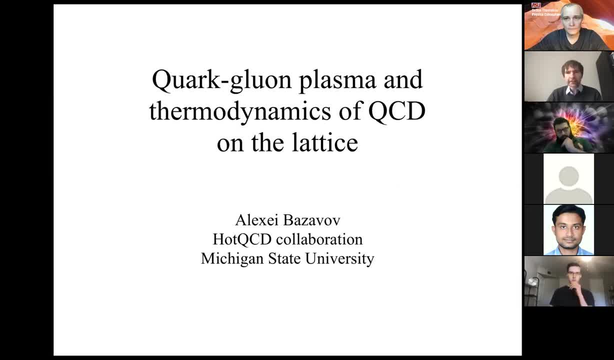 and this is mostly the work done. I'm participating in the what is called hot QCD collaboration. It started as a collaboration of collaborations in the early 2000s, then evolved. I will show you the current state of it, plus some other work which 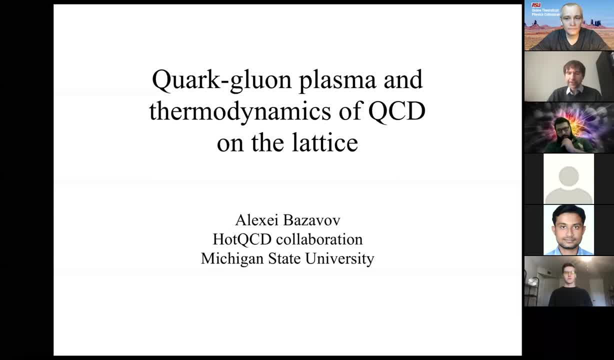 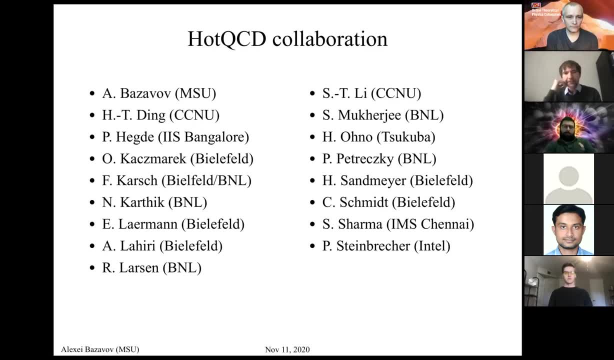 I have done with my colleagues beyond that. So first I start with some acknowledgements. That's the roughly current state of the HOT QCD collaboration. It's a group which mostly, initially, was centered around the Bielefeld University in Germany and Brookhaven National Lab, but then over time, with, you know, junior. 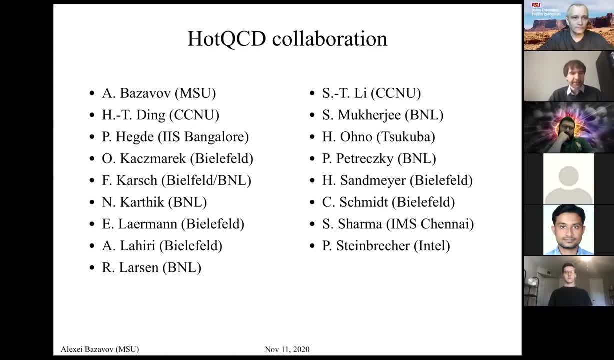 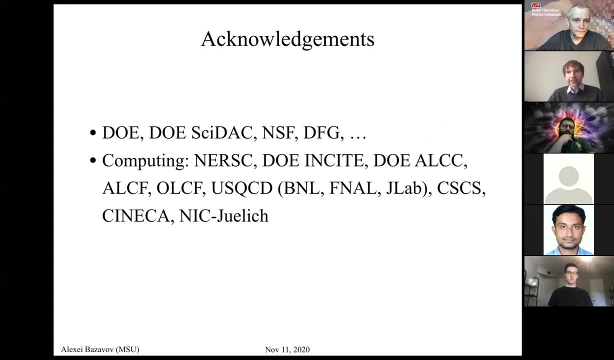 members finding faculty positions at various places. it became more international and most of the work I'm reporting is on behalf of HOT, QCD plus, as I mentioned, some other work. So this work relies on first of all, of course, on funding, as any work, but also on 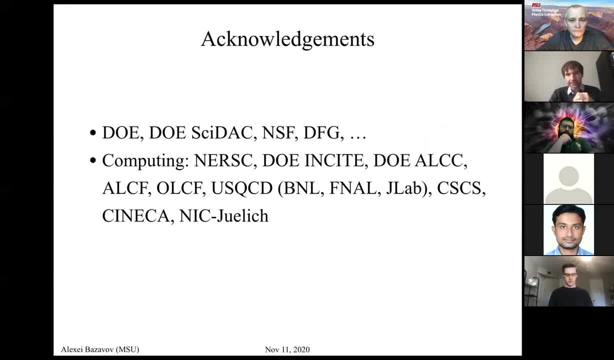 massive amounts of computation. So it wouldn't be possible, obviously, without funding from the Department of Energy, in particular from the Scientific Discovery through Advanced Computing Program, National Science Foundation, German National Science Foundation, Analog and other funding agencies, And the computing came from what we call. 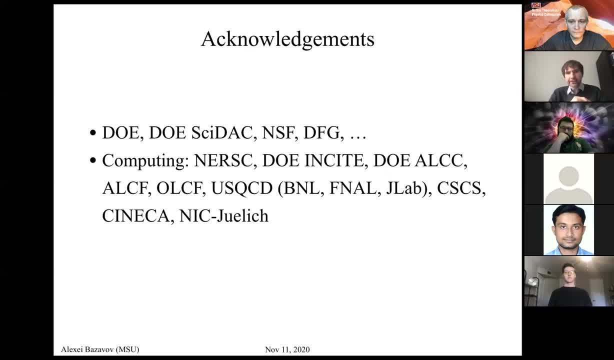 leadership class computing resources which are typically stationed at national labs in the US, large computer centers in Europe, in Switzerland, Germany, Italy. So it's a coordinated effort which which spent many years, and I will discuss at some point what makes these calculations expensive and what we can do about that. 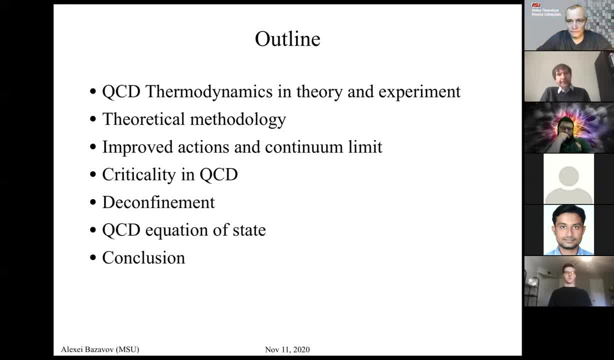 So with this I will discuss a little bit the outline. So first I would like to introduce what is the main physics we're interested in and what can be done in theory and experiment. and this would be very brief, sort of bird's eye view of things, of course. 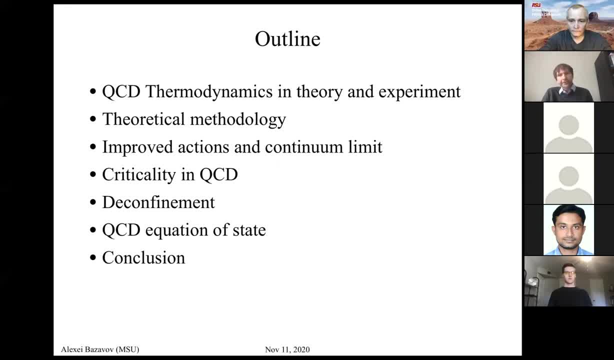 And then I discuss some theoretical methodologies that we build upon and, in particular, what technical things we needed to do to be able to proceed with the calculations, results of which I will discuss. And then I go into the physics part, the way we we can see and calculate on the 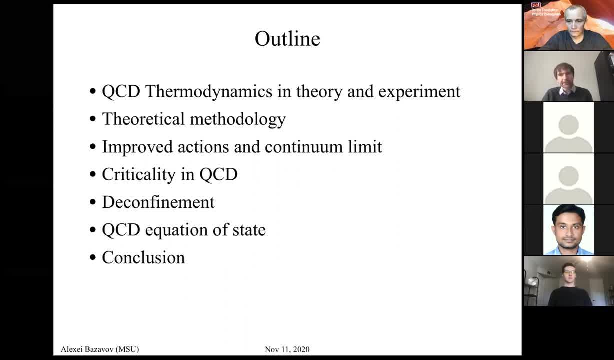 lattice. and what are the interesting features of QCD in particular, such as chiral symmetry, breaking and confinement. and what happens in the high temperature phase of the theory? what is the equation of state? and then I conclude. So, but before going into that, since this 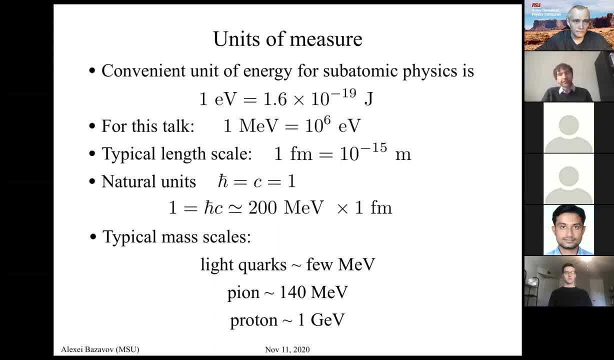 is a colloquium. let's get some feel of what we're going to discuss, And the first starting point could be: what are the typical scales that we have in the problem? And so, for basic physics, we typically deal with electron volts, which of course are: 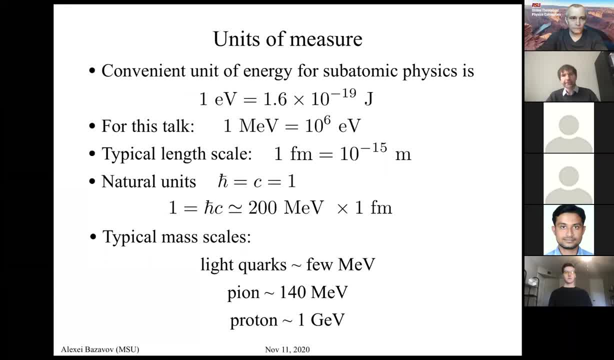 connected to system international units, but those are not very convenient in this case And for the QCD scales that we're after here we're on the scales of millions of electron volts, so basically MeV for the energy and typical length scales of 10 to minus 15 meter or one centimeter, And it is convenient to 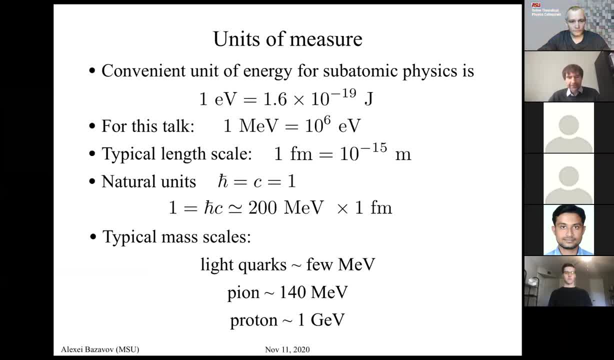 work in natural units, so one unit of quantum and one unit of relativity are set to one, which roughly gives us this relation between the energy and length scale that 200 MeV times one Fermi is roughly one in this unit, And so you. 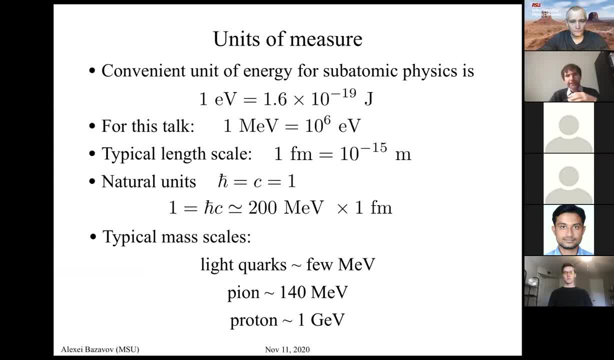 could immediately see that the length scales are related to inverse energy scales, and so that matches our intuition that to access smaller and smaller scales, we typically need colliders with higher and higher energy, And the typical mass scales that we have now for the dynamics that we're going to discuss are the 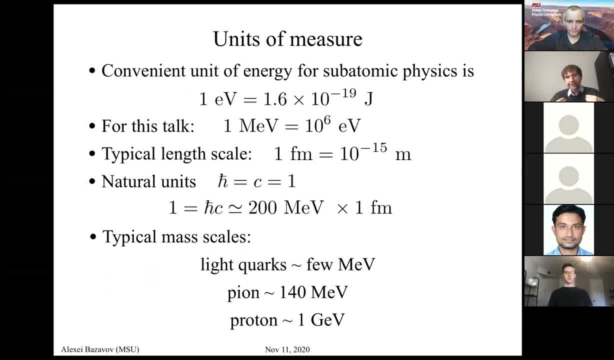 following: So we have the constituents of the theory, like works that determine most of the dynamics, and their masses are on the scale of few MeV. Then, as we'll see later, they're not observable in nature as isolated object. rather we observe some composites, And then the lightest state in the spectrum of QCD is 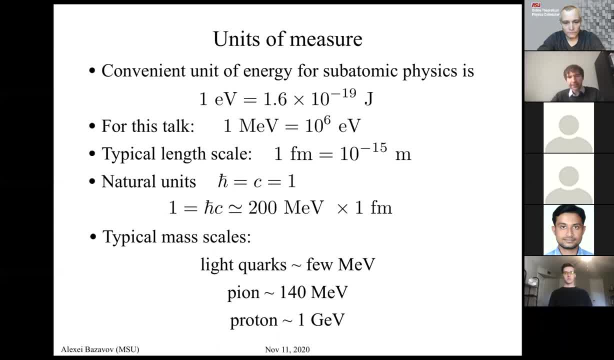 pion. so it's a quark-antiquark pair bound together and its mass is on the scale of 140 MeV and, as you'll see later, that's roughly the scale where most interesting things happen, And then most of the observable matter is in nuclei, protons and neutrons. so those are. 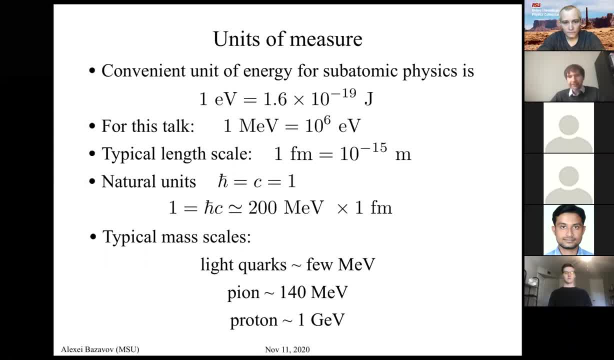 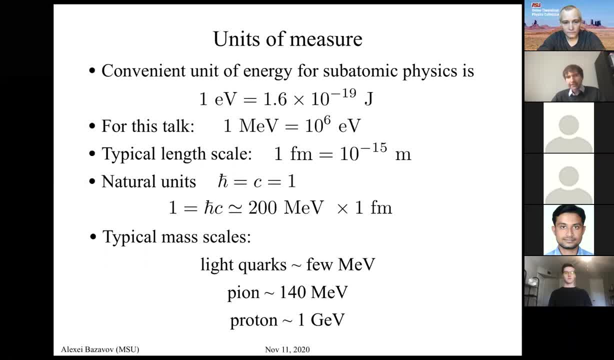 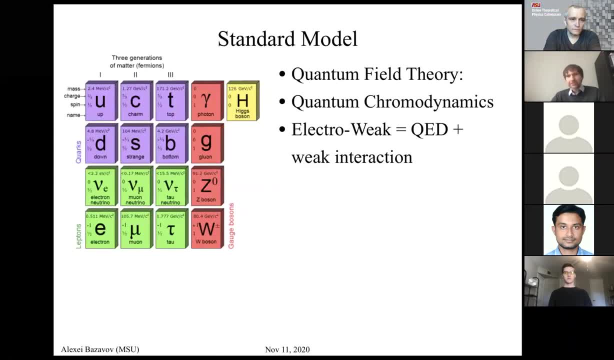 1000 MeV or 1 GV, And those are the typical scales that will play a role. Before narrowing down to the problem that I'll discuss, for the rest of the talk it would still be nice to pause and look at the whole picture in general. So 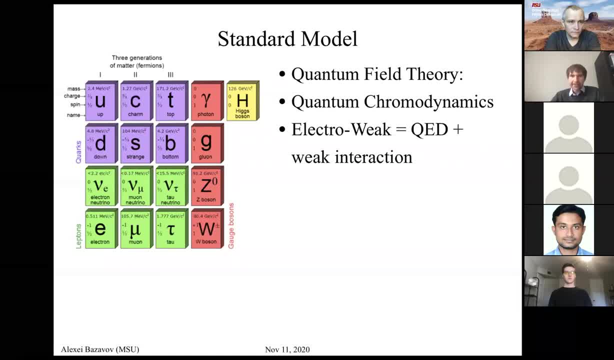 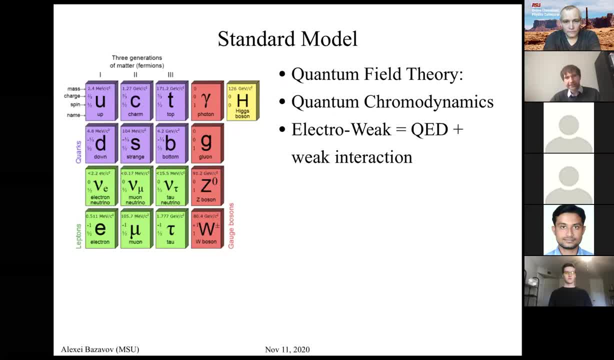 and the other four are significant. and the other four are significant and the other were us conveniently described by quantum field theories for the oncologicaliße特 across the standard model of particle physics over the last five or six decades. It's, of course, amazing to note again and again that a lot of observable phenomena gets down. 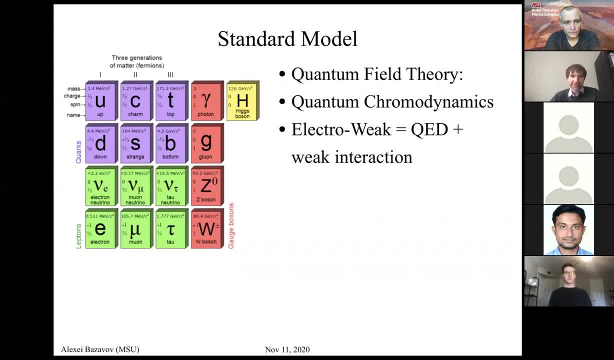 to a very small number of fundamental constituents. We have seeding genetics with, in trainings, fermions and leptons which form matter, and we have carriers of the force such as photon glue and weak bosons, and the latest experimental discovery of 2012 is the addition of the Higgs boson, which plays a special 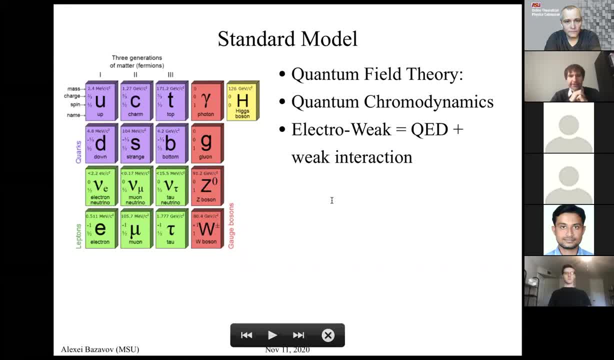 role- I will not go into details- important for electroweak physics and giving masses to the observable particles and so on. so, um, in a way, uh, as we know, it is very successful in describing the observable phenomena in multiple collider experiments. uh, but many puzzles, of course. 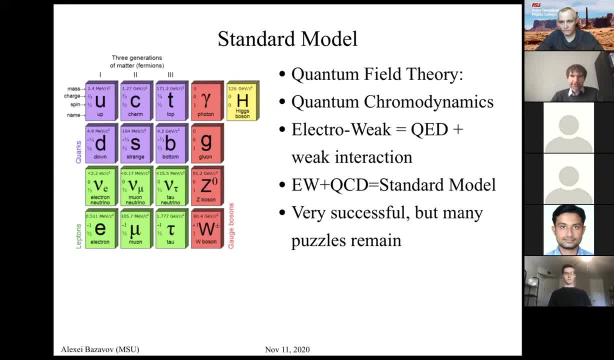 remain, such as dark matter or baryon, anti-baryon asymmetry and many things alike. plus, does not include gravity, so big open problem to to eventually include quantum theory of gravity into the picture if possible and uh, to get a feel of how successful things are. one of often. 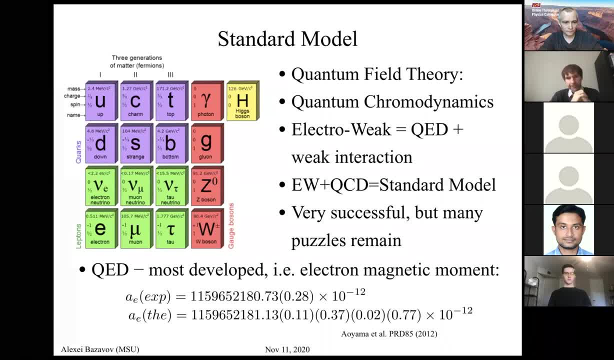 cited examples is the anomalous magnetic moment of electron. so again, I'm not discussing the technical details, but just by looking at that we can admire that. it's a quantity which is known to amazing precision both in experiment and theory, and uh, as we of course know, the most developed and tested part. 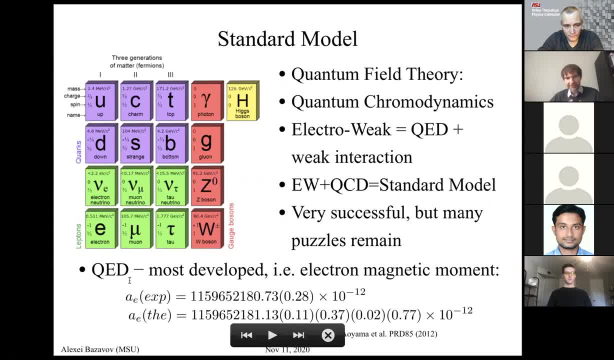 of the standard model is electrodynamics, which was successfully developed classically for over 150 years, uh on on quantum level in the 40s and 50s, with the work of Feynman, Schwinger and many others, and uh, what's interesting to note here is that this is, uh, this is a what we call perturbative. 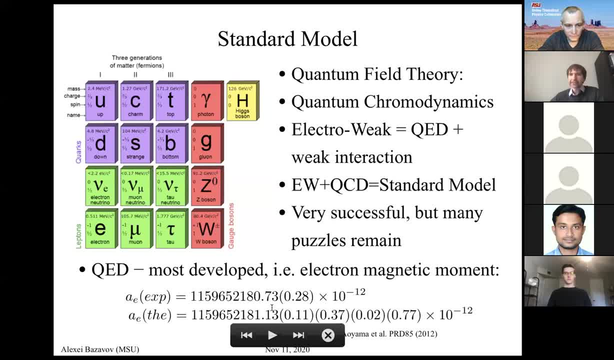 calculation where the uh, the answer, is achieved by Taylor expanding the quantities that we want in some small parameter, in the theory and at very high order of this Taylor expansion. eventually, all of the data that we have is actually taken from the quantum level. so that means that all interactions contribute and the largest uncertainty 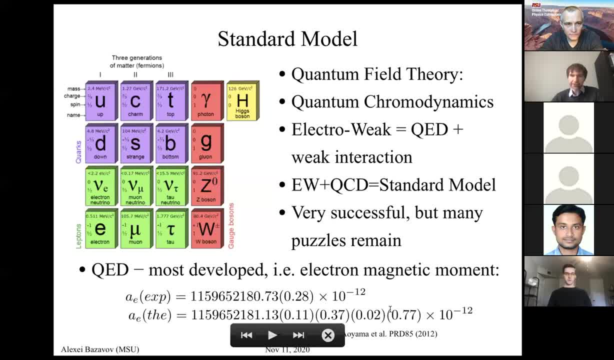 in this quantity actually comes from the strong interactions and QCD, the quantum chromodynamics. the theory of strong interaction is, uh, less developed. there are technical challenges, and that eventually what leads us to the lattice QCD formalisms that this talk builds upon. so we're pretty sure this works. 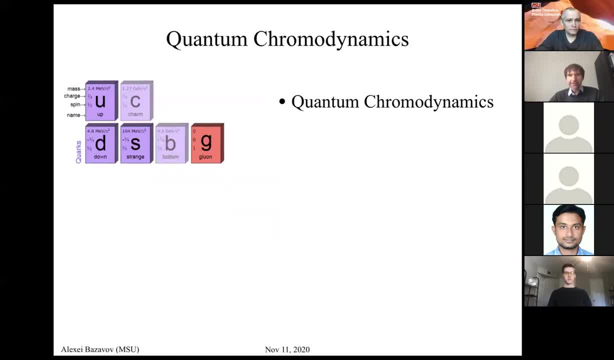 uh. however, for the phenomena I want to discuss as thermodynamics of QCD, we narrow down to strong interactions only. we are at the scales. we can safely switch everything else off. we can neglect the top quark because the mass is so high plays no role on the scales we're interested in and 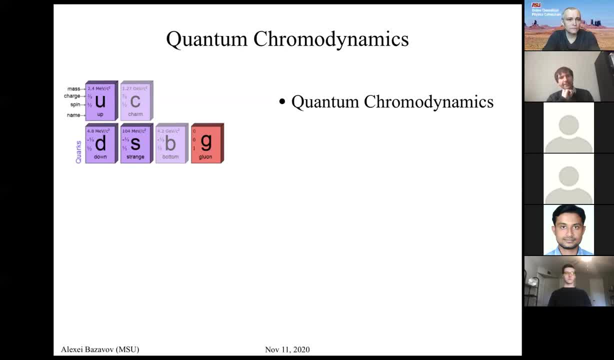 most of the dynamics is determined by the light and strange quarks. so those are the main degrees of freedom plus the gluon to carry the interaction. however, behavior quarks. they also play some role later in the talk and they could serve as a probe of the dynamics dominated in the environment by the light works, and we'll discuss this a little. 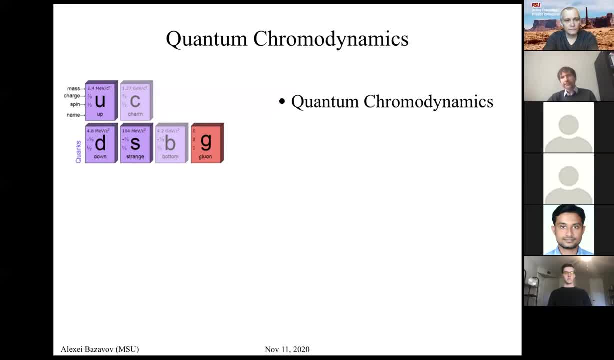 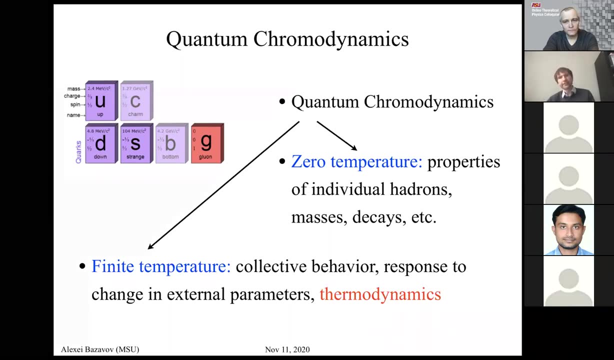 bit later on. so at this point I could roughly classify the type of calculations we can do in in two domains that we have something that we can classify zero temperature calculations, where, when, we're interested in what are the properties of individual hadrons, composites of forks. 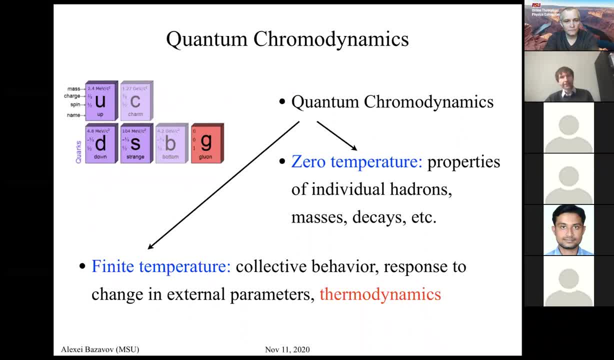 their masses decays. various form factors- And those are typically many of those types of calculations- are precision calculations on the lattice. They could be done with high degree of control, small statistical and systematic errors. Some quantities get precision of sub percent level. now 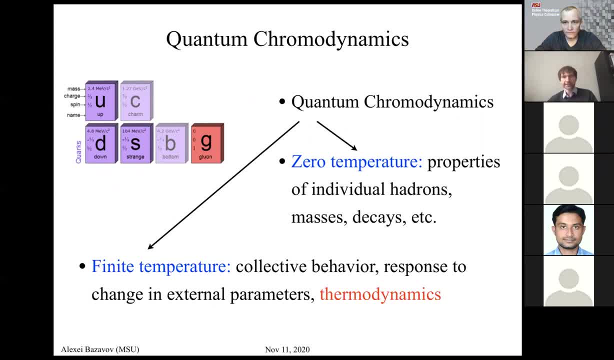 and they play a role in combination with other calculations and they compliment the various experimental programs and they are required in many cases to extract things like, for instance, C-kind matrix elements which are responsible for the weak sector. but all the QCD background is encoded in various quantities. 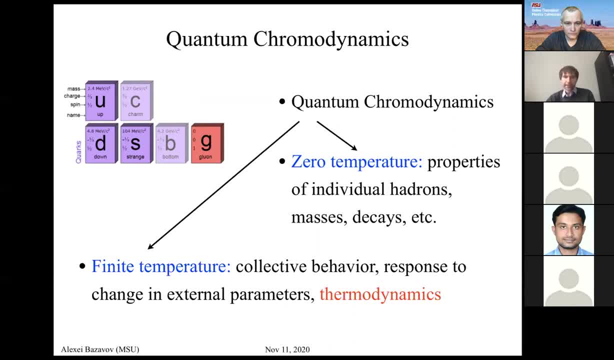 which have to be calculated in lattice QCD, And then another domain is finite temperature field theory, where we're interested in some collective behavior. So we can see there's some macroscopic amount on the scales of QCD of strongly interacting matter And this is basically a thermodynamic description. 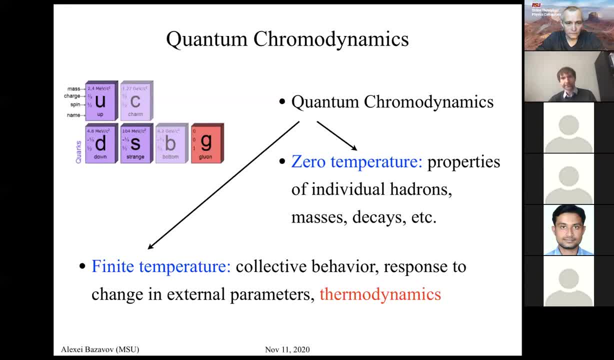 which means we're normally looking at systems in equilibrium. that would play a role as some disclaimer later on. So in other words, we're looking at systems in equilibrium. in other words, we want to know how some macroscopic amount of strongly interacting matter responds to change. 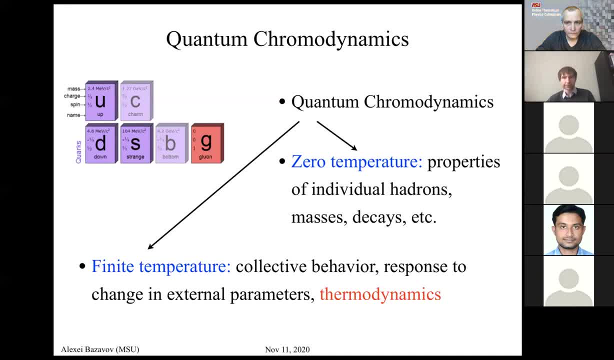 in some external control parameters such as temperature or density or other things. So- and this is the focus of today's talk- So we look at thermodynamics of QCD and we need lattice as a tool to study So we can quickly contrast. 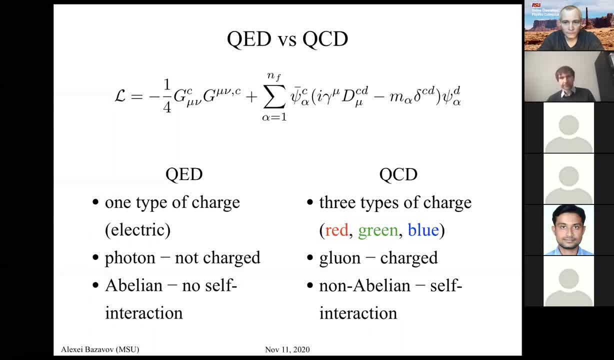 electrodynamics and quantum chromodynamics and build a little bit upon the past developments. So when I refer to first principle calculation later on, what I typically mean by that is that we have the fundamental Lagrangian. it encodes all the degrees of freedom, all the interactions. 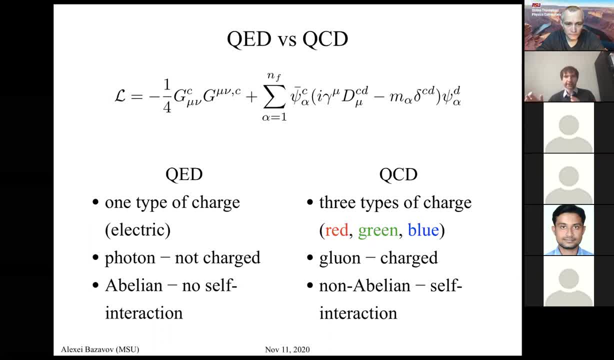 And ideally we would like to extract all the observable, measurable quantities From that somehow. And so, as I mentioned, in electrodynamics the perturbative calculations are very well developed. There is a small parameter which is a fine structure: constant alpha, one over 137,. 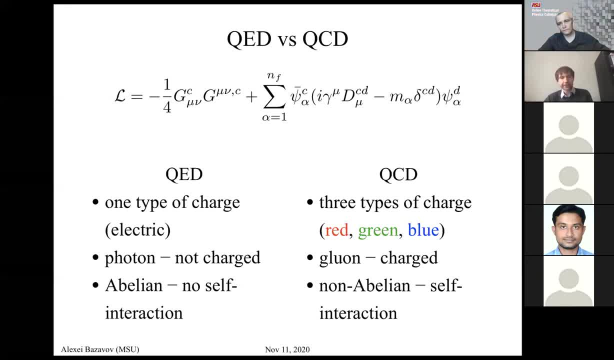 that typical scales of everyday world, And this is a parametrically small parameter which allows for building this- perturbative expansions. And so from that perspective we could say we have one type of chart, the electrodynamics, and one type of charge in QED. 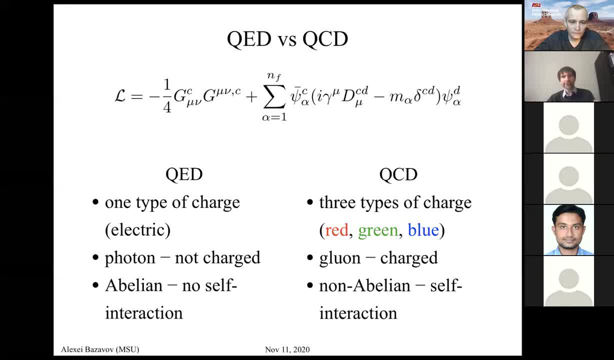 The carrier of interactions, the photon itself, is not charged, meaning there is no self-interaction. And in our technical description we say it's a billion gauge theory which describes electromagnetism. In contrast, in QCD we have the Lagrangian. 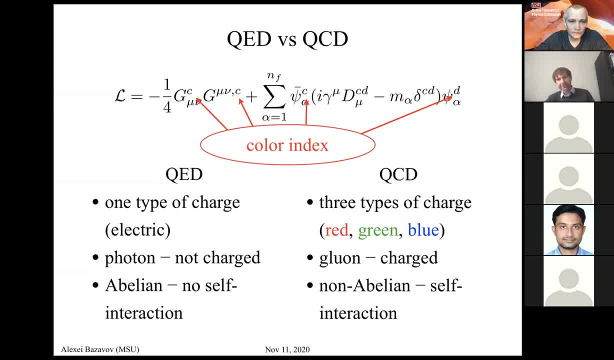 which looks more or less the same way, but we have this extra degree of freedom, the color charge And the carrier of interactions. the gluon is itself charged, Which leads to self-interaction and non-trivial dynamics of the theory. 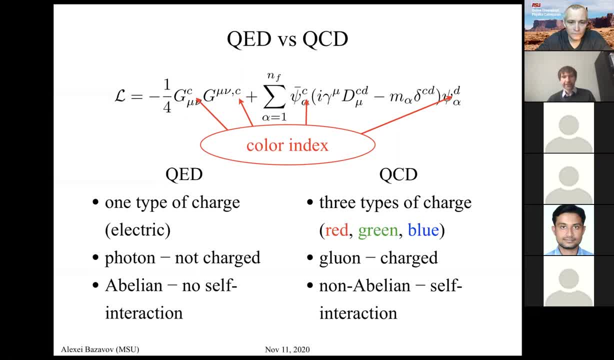 even if we just look at the gluons only. So if we look at the photons only, then we have just black body radiation. but in QCD, even without thermions, we have a non-trivial, non-ambient gauge theory dynamics. 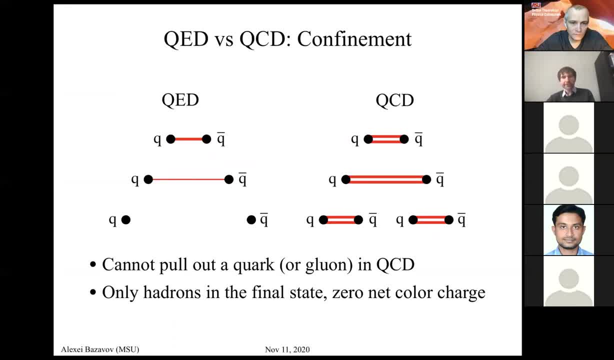 So here is a cartoon which is not completely correct but still represents some things that I want to communicate. So if we look at, ask ourselves the simplest question: how we can approach studying some force in nature And in electrodynamics on the classical level. 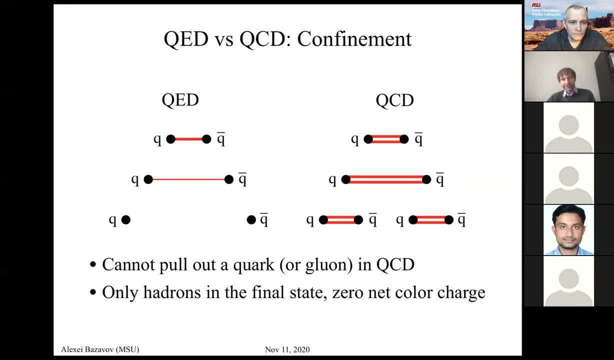 one of the starting points was the discovery of the Coulomb's law that if we have a static charge and anti-charge, we can study what is a force that we have between them. So it falls off as one over R squared. So if you recall from Jackson, 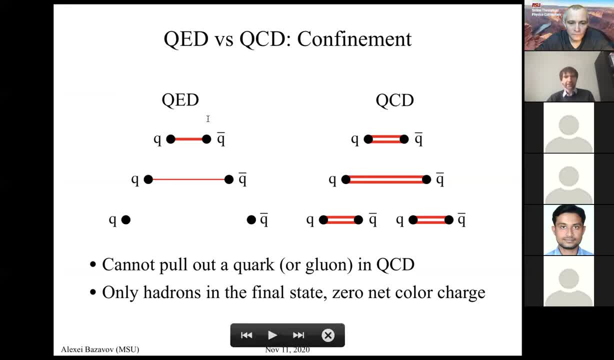 if I were to draw the field lines, then they occupy the whole space between charge and anti-charge. But what I'm trying to represent here is rather the fact that the force dies off with distance And if we separate things far enough apart. 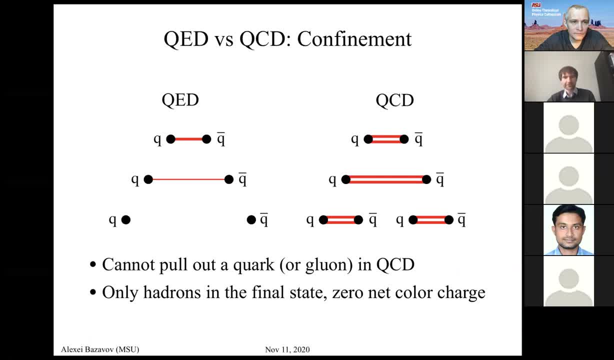 we could effectively have this force set to zero And eventually we can pull the constituents macroscopic distance apart, So we could deal with isolated electrons, measure them and things like that, In contrast in QCD. And so this is. this cartoon is closer to reality. 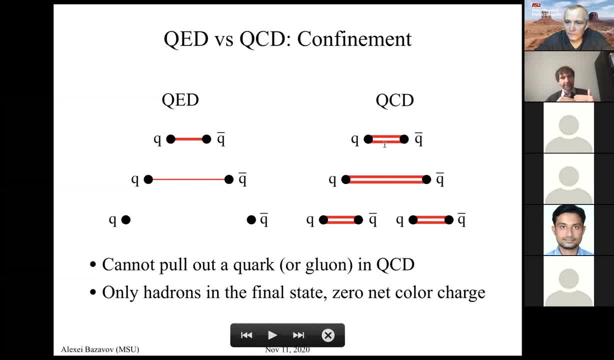 The field lines are squeezed into a flux tube and the force is constant, And so when I'm trying to pull the system of quark and anti-quark apart, I have to invest more and more energy into the system, So at some point it becomes. 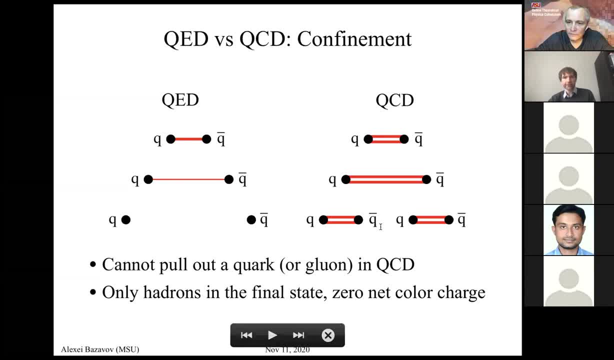 it becomes energetically more favorable to pull out a pair of quark and anti-quark from the vacuum and break that connecting stream. And so if I started with a meson and I'm trying to break it, eventually I end up with more mesons. 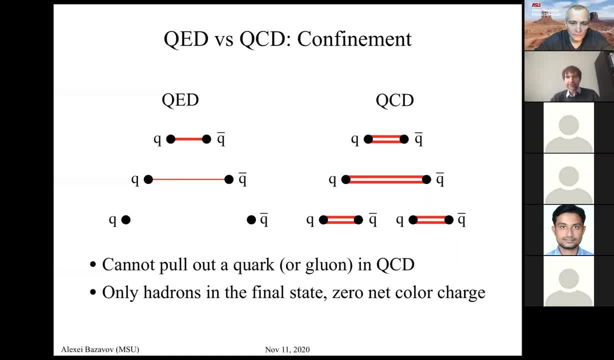 or other composite objects. So the main point out of it is that we only observe the composites, the hadrons, at macroscopic distances in the detectors as a particles of the final state. So this is a confinement phenomena and it's not something you could really precisely define. 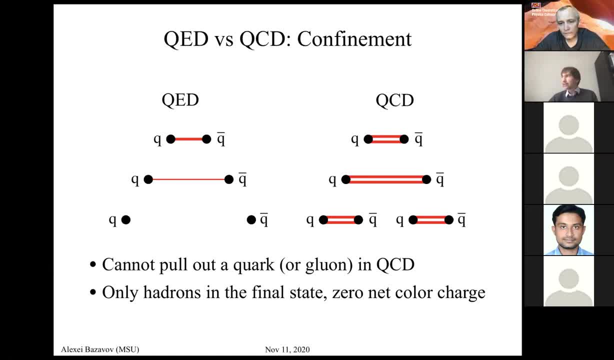 but that's a loose cartoon telling us that unfortunately, we cannot have the constituents as asymptotic states. However, we could still study the spectrum of QCD in the same way as we can learn about electrodynamics by studying the spectrum of the hydrogen atom. 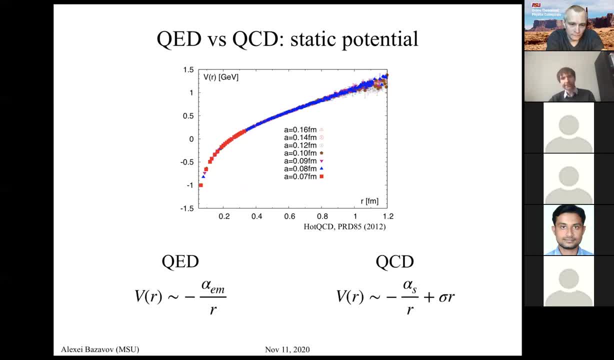 And that's in a way what we do in lattice QCD. So if I sort of extend this to more realistic, measurable things, on the lattice, then we can look at the static quark-anti-quark potential, and this confinement is manifested in linear rise. 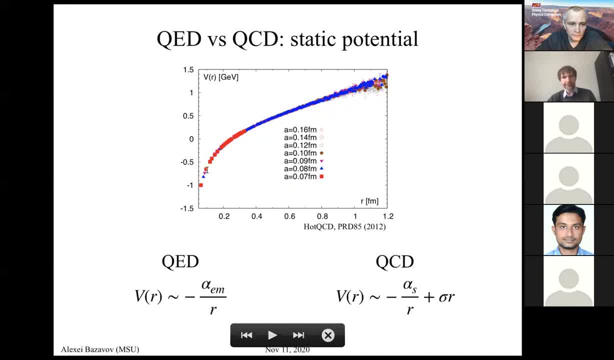 at long distance. So the short distance behavior matches the one in QED, so Coulomb's law. but the long distance phenomena shows up as confinement. Realistically it eventually has to level off due to the string breaking formation of these extra mesons and stuff. 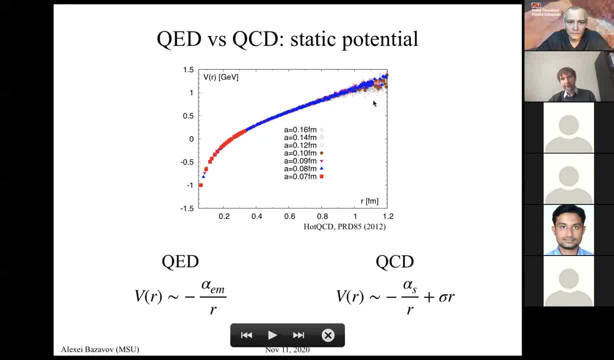 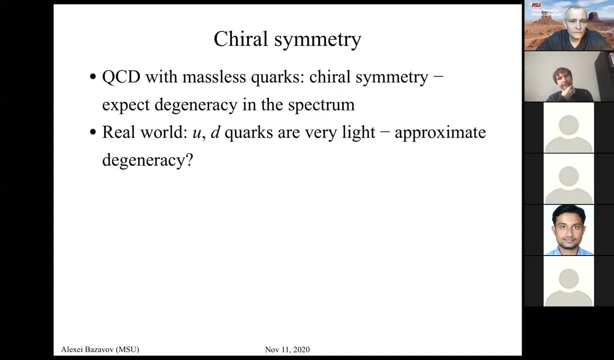 This is not reflected here, but let's just to give you some feel of one of the ways to look at confinement from this perspective. Another phenomena which is manifested in QCD is the following idea: So when we have massless quarks, we have massless quarks. 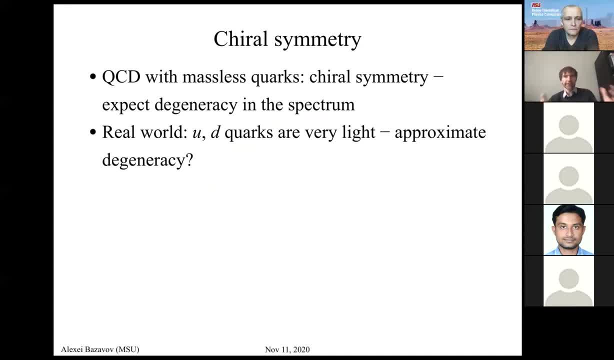 there are transformations, which leaves the action of the theory invariant, And in these cases we can expect that there is some degeneracy in the spectrum, because there is some symmetry relating different states, And so based on that, one could argue. well, in the real world. 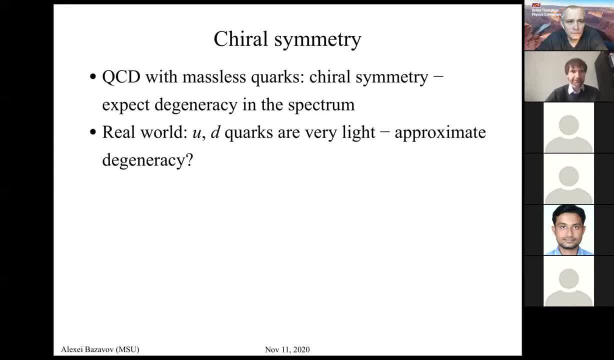 all the quarks are massive, but the masses of light UND quarks up and down are so small that maybe we can expect at least some approximate degeneracy because, remember, the masses of these quarks are on the scale of few MEV. 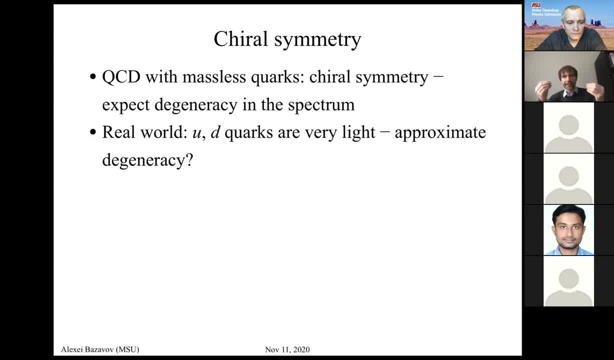 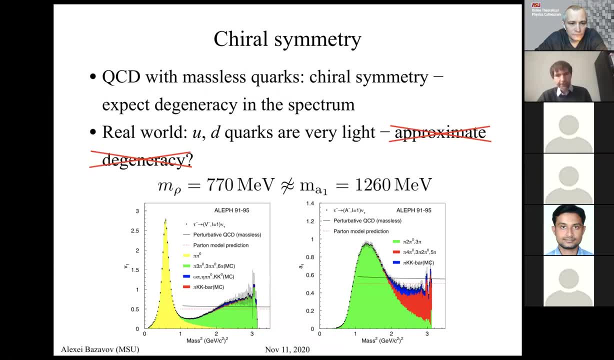 So maybe we can expect that some partners in the spectrum would sort of be within several MEV apart. However, this is absolutely not what we observe, And some states, which would be degenerate if the chiral symmetry was manifest, are actually very far apart. 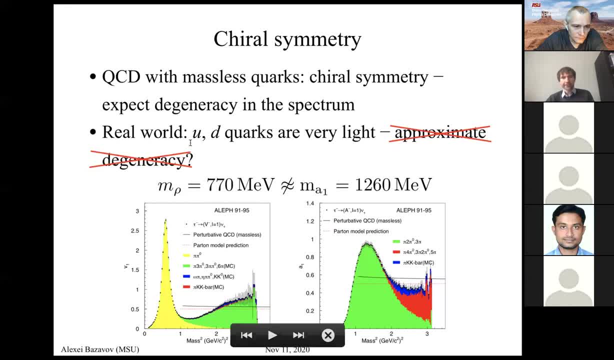 And again, I'm not going into the details, but just by the look of it it's very clear that you know, if you look at these two pictures, which are in a way some sort of spectral functions here or invariant mass kind of plot, 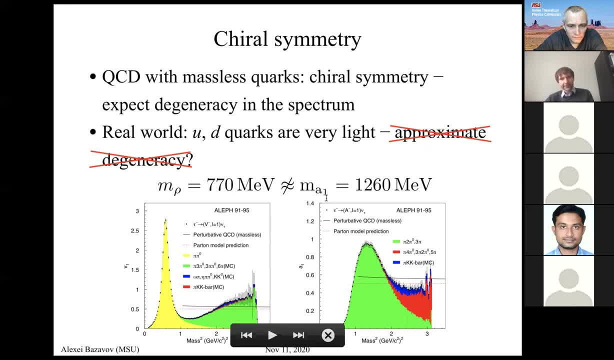 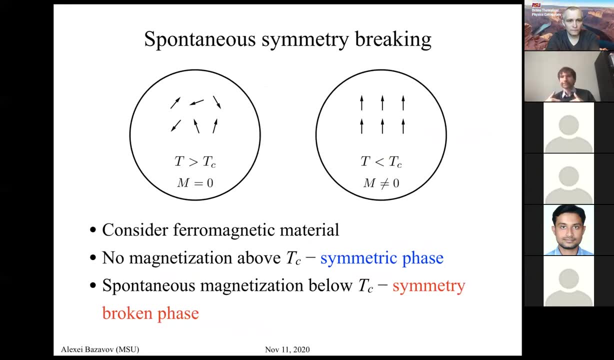 they look very, very different, The states see that very different masses, and they're not degenerate within a few MEV, as one could maybe expect, And so this is what we call spontaneous symmetry breaking. In other words, there is some symmetry respected by the Hamiltonian. 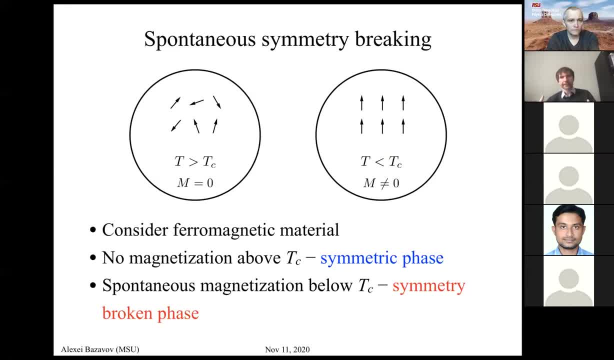 or the system, but it's not respected by the ground state. the system chooses And that can be related to simpler models where very similar phenomena is manifest and sort of easier to comprehend. If we look at ferromagnetic type of material, where we represent these atoms with little arrows, pins, 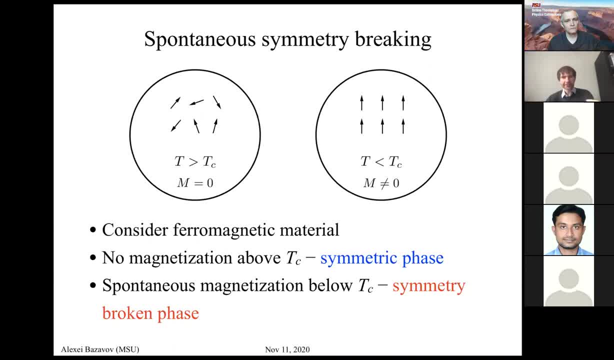 and then there is a variety of models to describe these interactions. Typically what we have in those models that we have some Hamiltonian describing some sort of nearest neighbor interaction. and then we want to know how the system behaves on macroscopic scales And so in the high temperature symmetric phase. 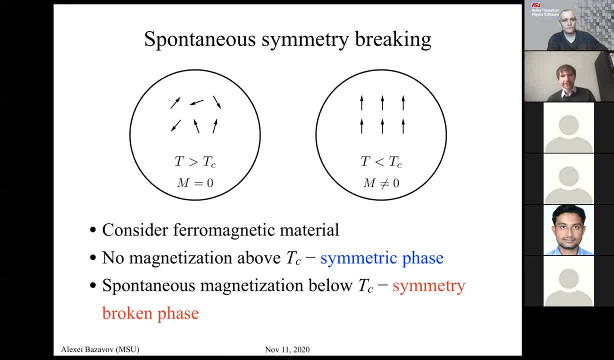 typically the system is not aligned. all the spins face random directions And then when we add their total contribution and ask what is the magnetization of the piece of this material? and it adds up to zero. However, at low temperatures, although the Hamiltonian describing 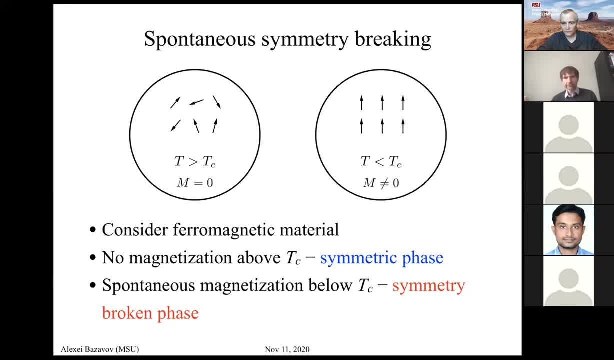 this nearest neighbor interaction doesn't have a preferred direction, so all directions are equally possible. spontaneously, system is magnetized and it breaks the symmetry by having non-zero magnetization and choosing some preferred direction. So this is a phenomenal, spontaneous symmetry breaking, and something similar happens to chiral symmetry in QCD. 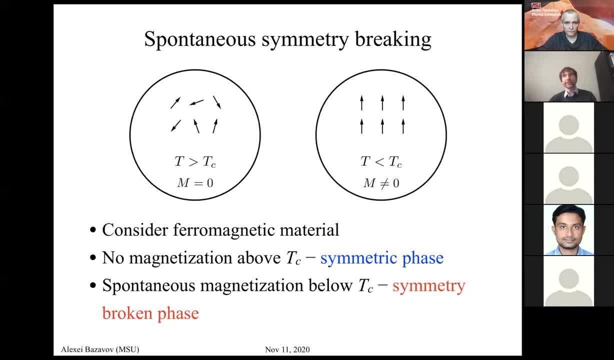 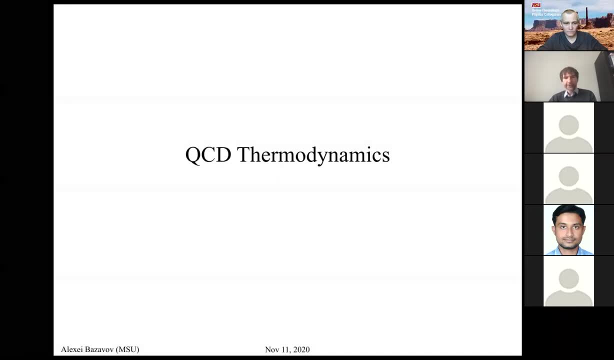 So the ground state of QCD is actually very complicated. So in fact it's in a way easier to deal with high temperatures than with the ground state. So now let me go into the QCD thermodynamics and I'll try to go through this fast. 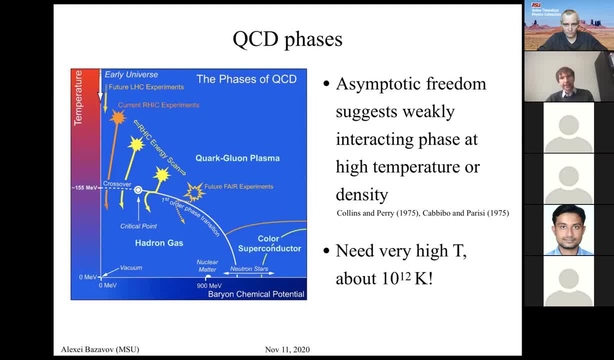 So this is something that you'll probably seen many times in various colloquia, and this is approached from various directions. We're interested in thermodynamics of QCD and basically in its phase diagram, where we typically plot it in this way: as a function of two variables. 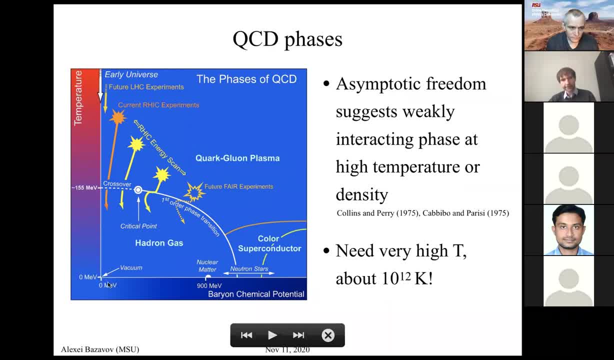 two external parameters, such as temperature vertically and the chemical potential on the X-axis, And so it's a crowded plot. The main point I would like to focus is that the expectation- so I would call it a conjectured phase diagram because there is not yet full- 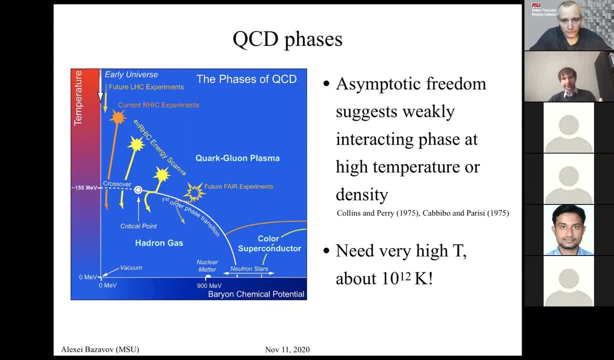 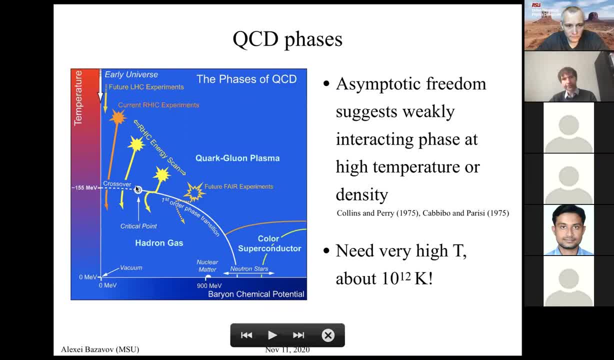 of first order phase transitions, which ends at a critical point, And then, if we continue this line, it ends up as a crossover, And so the most studied region of this diagram is basically the vertical axis. That's where all the direct simulations in lattice QCD are possible. 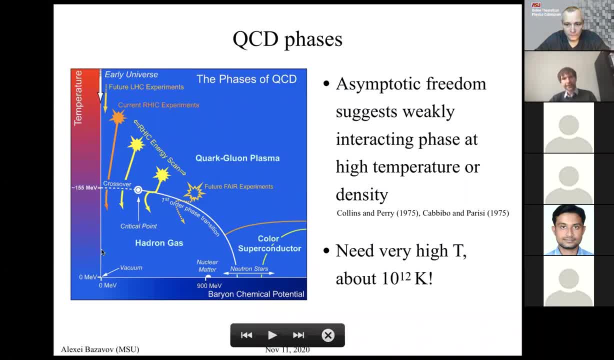 And a lot is known. a lot is known now And a little bit is known about the strip close to the Y-axis. So this phase diagram is a subject of theoretic investigations and very lively experimental program And we need very high temperatures. 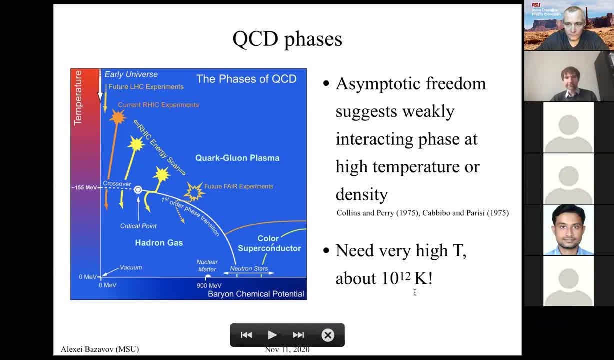 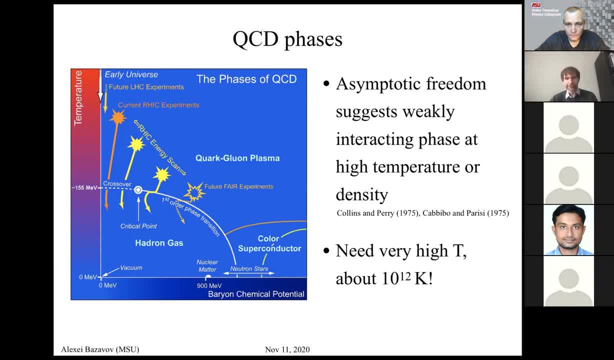 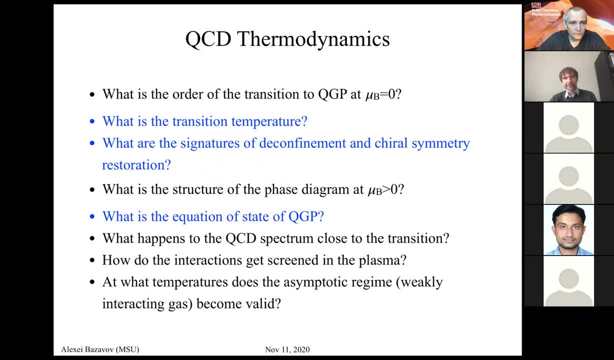 Something on the scale of large nucleus would do And what questions we can address. So I can quickly summarize that. So we're interested in what is the order of this transition, how we can define the transition temperature, how we can study deconfinement. 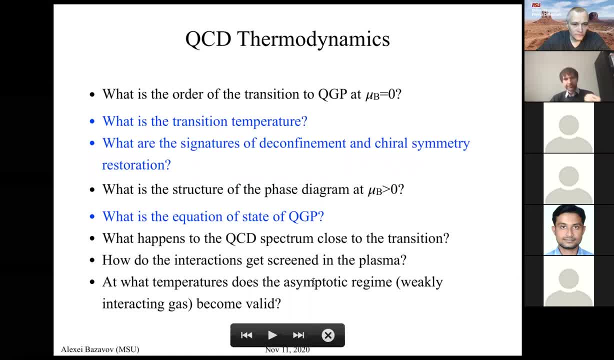 and restoration of chiral symmetry A very big, open question. what really happens at non-zero chemical potential? It's very hard to access Theoretically from the QCD Lagrangian but a lot is known from effective models. So there are various phases predicted. 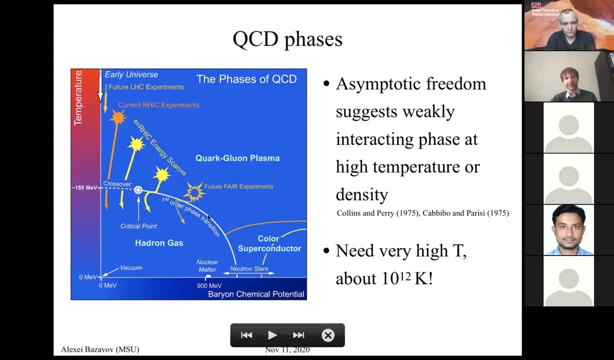 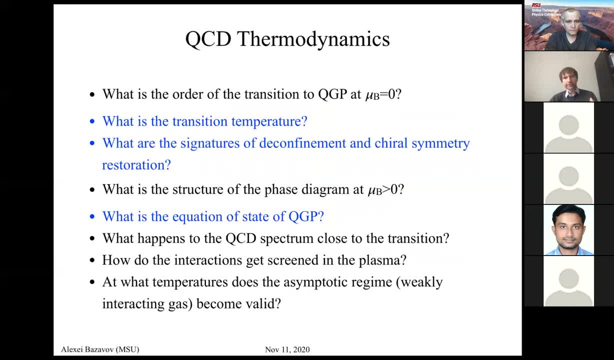 that low temperature and high density and that's the region which is extremely hard to access in lattice QCD for technical reasons. So we would like to know what is the equation of state for quark-blown plasma and what happens to the spectrum screening and things alike. 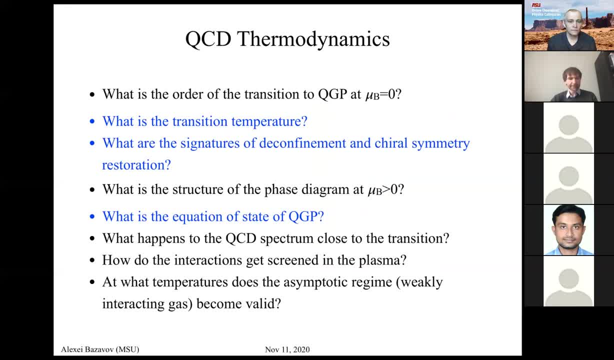 So it's not possible to cover all of these, but some of those features I would like to know And I will discuss in this talk. So, from the experimental side, the two largest Hadron colliders in the world are relativistic heavy ion collider at Brookhaven. 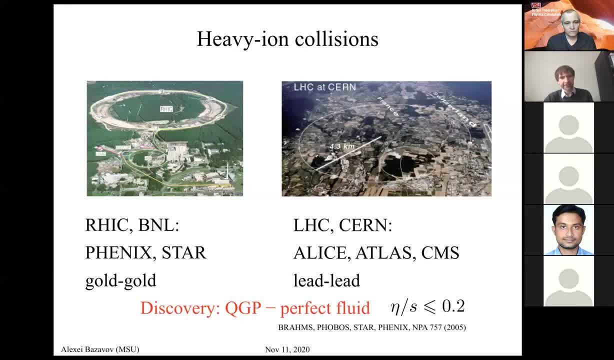 and obviously the largest one is a large Hadron collider at CERN And the Brookhaven one is focused on gold-gold collision, colliding heavy nuclei, and invest so much energy in the collision so it could, and invest so much energy in the collision so it could. 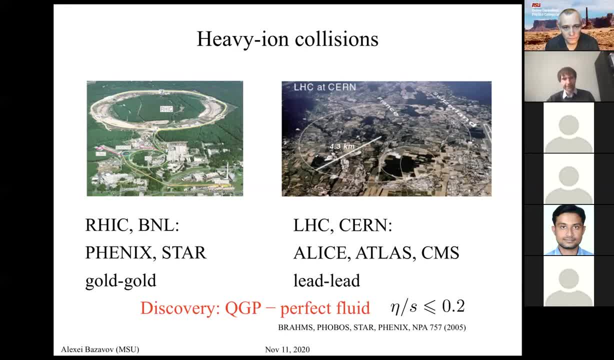 and invest so much energy in the collision so it could turn the system into the core-gluon plasma phase And the. as you know, of course, the main physics goal of the Large Hadron Collider is the energy frontier. investigations in proton-proton collisions. 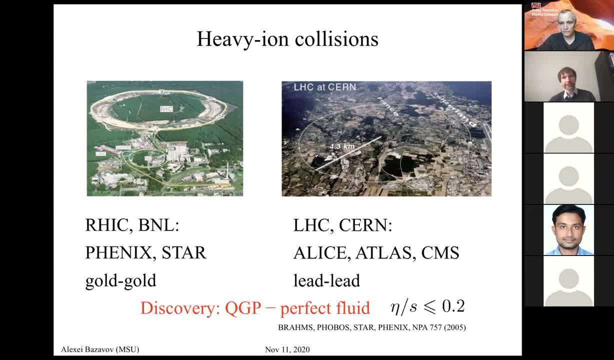 So trying to create new types of particles by colliding protons at very high energy. But part of the program is also dedicated to heavy ion collisions with lead And various experiments. ELISE is primarily focused on heavy ion collisions, ATLAS and CMS, of course. 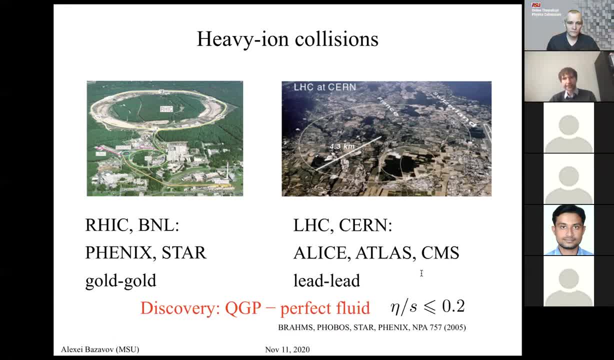 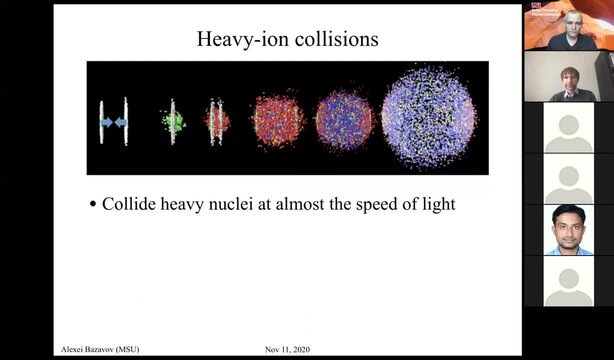 mainly dedicated to proton-proton collision, but they also gather data from the heavy ion program. So, without going into too much detail, a quick cartoon of a collision would be the following: So if we look at photographs of the system, so artistic. 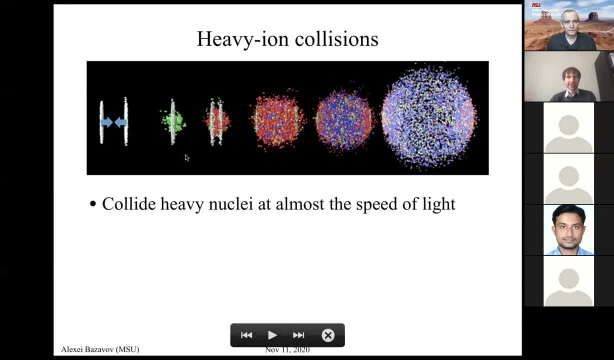 This is a depiction of that As it progresses in time. then we have a collision of two nuclei which are moving at almost speed of light and we're sticking it in the center of mass frame. They collide and the deposit of energy is so high. 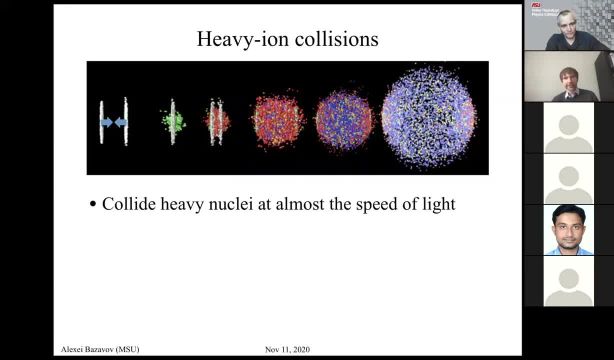 that we expect that the system turns from the hadronic phase into core-gluon plasma phase, And then it's essentially an explosion. The system starts to expand, cool down and, due to confinement, the system starts to expand And due to confinement, as we discussed, 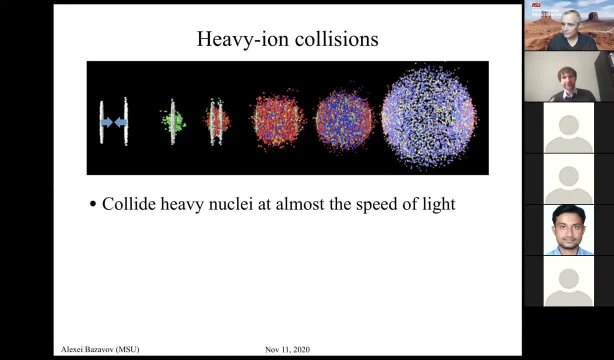 all we can detect as particles of the final state are hadrons again, or they're decay products. So the formalism of lattice QCD is of course unable to address this full real world collision dynamical problem, And so what I'll discuss in later. 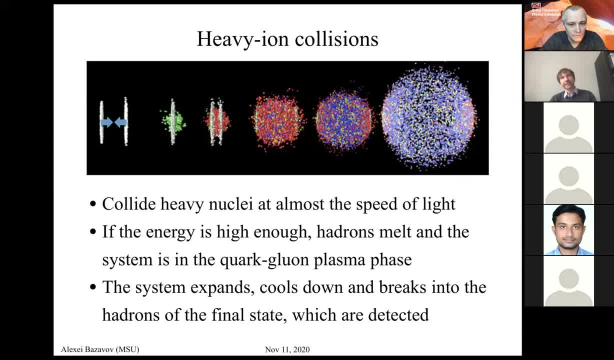 is that we consider an infinite amount of strongly interacting matter in equilibrium. So we're taking thermodynamic limits sort of implicitly and so on, and it's up to experiments to some degree to understand how much of this applies to the real collision problem. So this process is typically modeled with hydrodynamics. 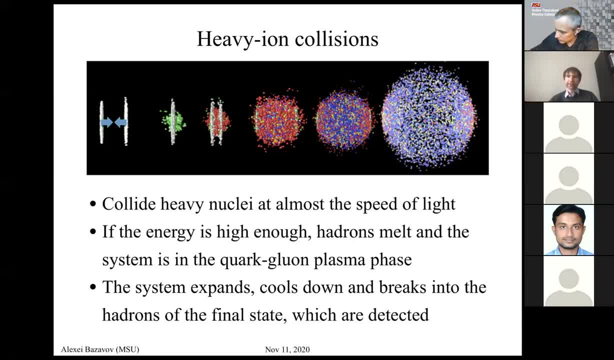 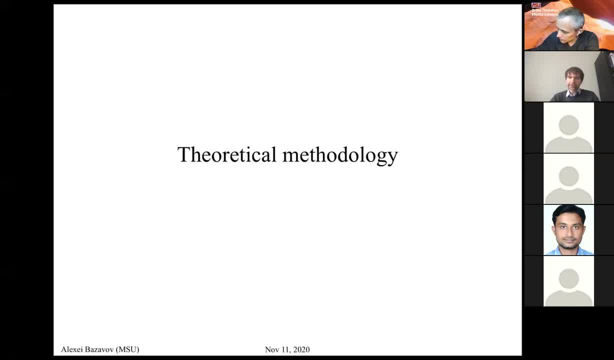 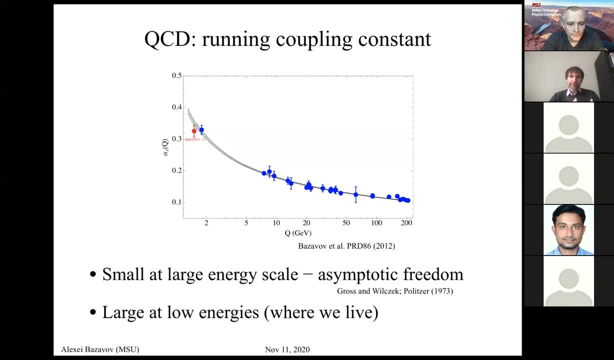 but things like equation of state. they serve as input to that model. So with that, a little bit of disclaimer, let me go into the theoretical methodology that we need. So we have this confinement chiral symmetry breaking. So the low temperature phase of QCD is very complicated. 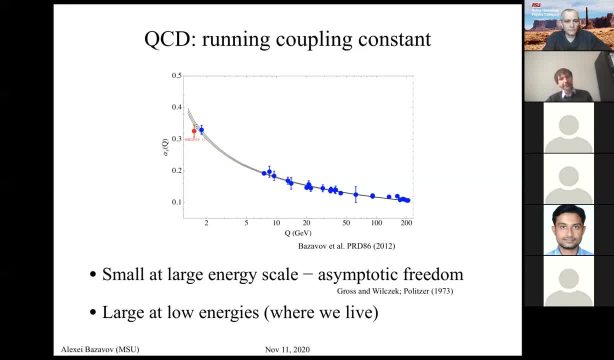 And another manifestation of that is the fact that the coupling constant right, the parameter which determines the strength of interaction, we call it running coupling because it changes with the energy scale And while in electrodynamics it's slightly growing with energy, but let's say approximately constant, 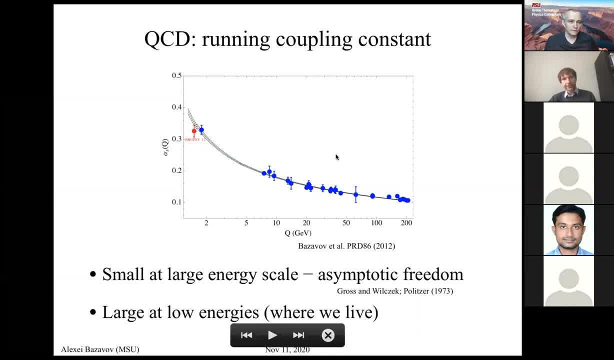 and it's parametrically small. in QCD it changes very fast over sort of short region of the energy scales And it goes to zero at infinite energy, which manifests this phenomenon of asymptotic freedom. And this of early 70s led to discovery of QCD. 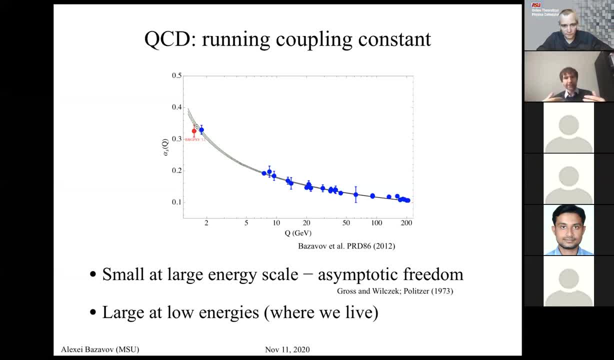 when people were looking for quantum field theories which have this property, which was sort of hinted at experimentally first, that at very short distances a constituents of hadrons behave as almost free, And the big discovery was that non-abelian gauge theory. 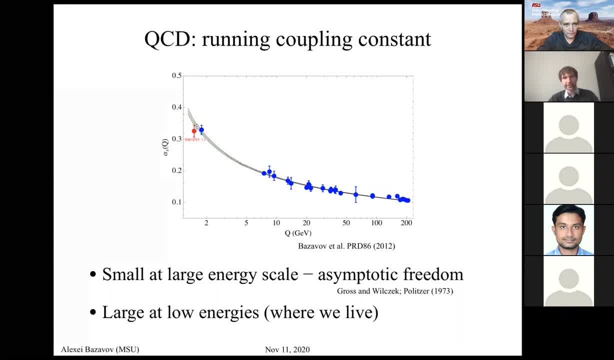 actually possesses property- they're renormalizable- that they could be valid candidates for describing strong interactions, And that's what led to discovering development of quantum chronodynamics. However, decoupling is parametrically large at low energies, where hadrons exist and where we live. 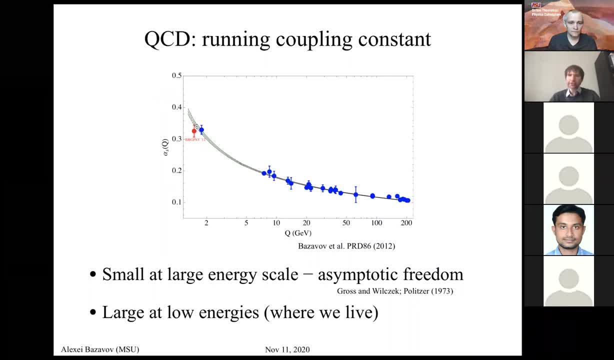 So we need something else which does not rely on small parameter or weak coupling expansions to address problems related to strong interactions at energy scales of order of hundreds ME. When we are in the regime of collider experiments at high energies, then perturbative QCD perfectly works. 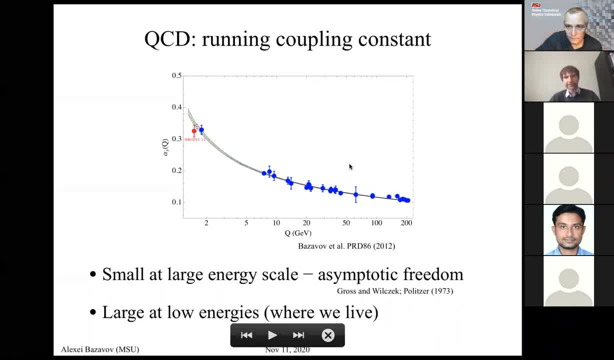 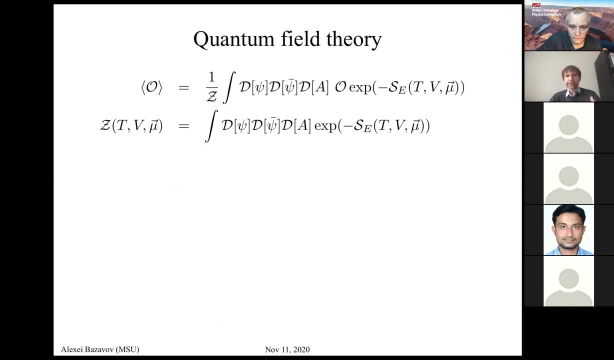 You still need some input for form factors and so on. but at least in this regime you can rely on perturbation theory, but it's not the case on the thermodynamic scales that we're interested in here. So formally, in field theory we can write: 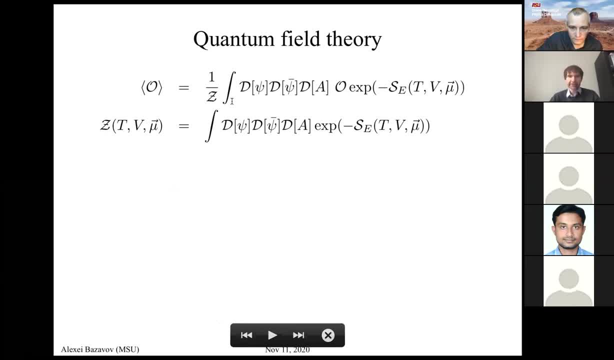 you know, quantum mechanical average of an observable that we're interested in as a in a path integral formalism, where it's basically saying that we integrate over all possible configurations of fundamental fields, which different subspace time domain and these configurations of the fields are weighted. 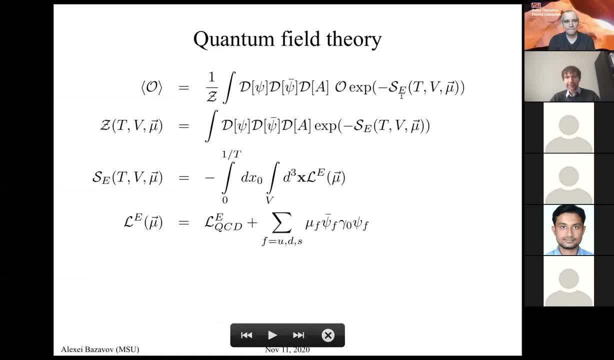 by the action of the theory. So here I'm gearing towards finite temperature calculation. So it's basically written as a partition function. So once again the Lagrangian of QCD, where we have the usual gauge part: Electromagnetic field strength tensor in electrodynamics. 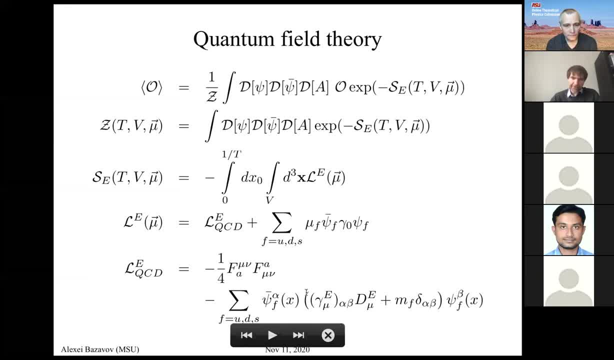 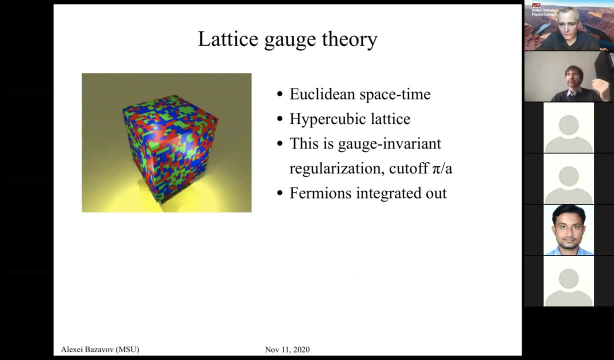 plus the fermion part which couples and tells us how fermions interact with the gauge field and through the gauge field with each other. So this is relatively standard up to this point. Now, how we can deal with the fact that we cannot rely. 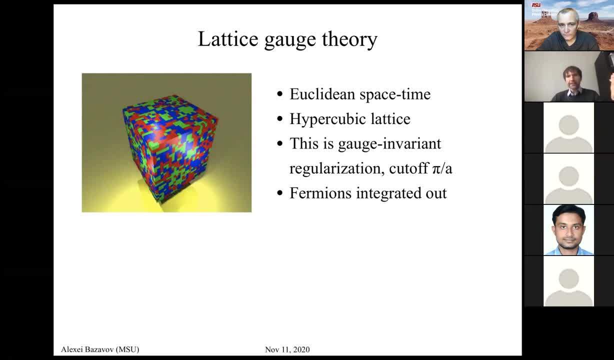 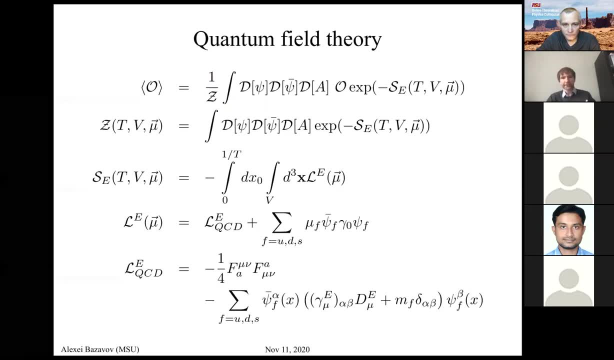 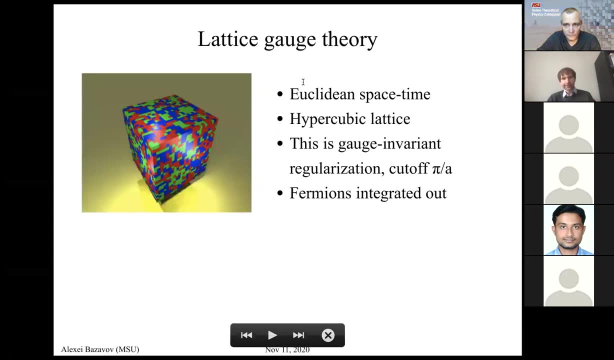 on expansions anymore. Well, the idea of numerical part of lattice QCDs is basically to brute force evaluate those path integrals by basically integrating over possible values of the fundamental fields. So for this we need several prerequisites which are non-trivial and were figured out mainly. 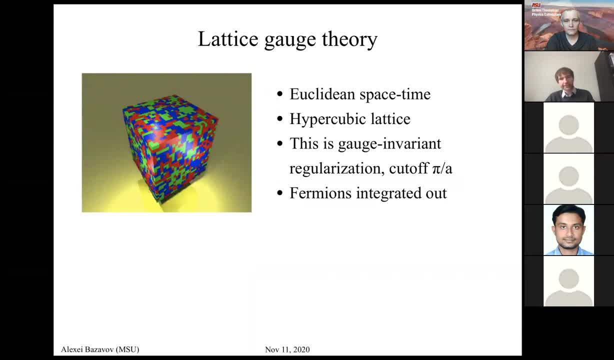 in the seventies through the work of Kenneth Wilson. So for technical reasons we prefer to switch to Euclidean space time. So we do rotation from real to imaginary time, then we discretize space time. And what it does? it makes the highest momentum of the system bound. 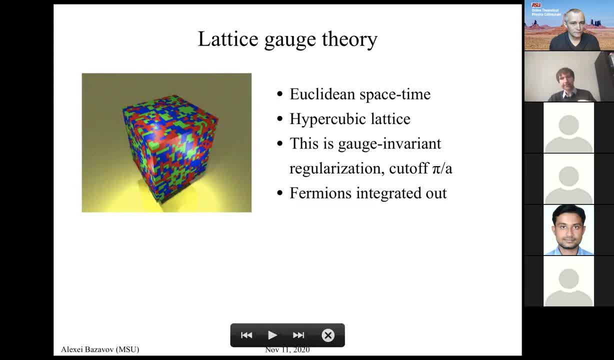 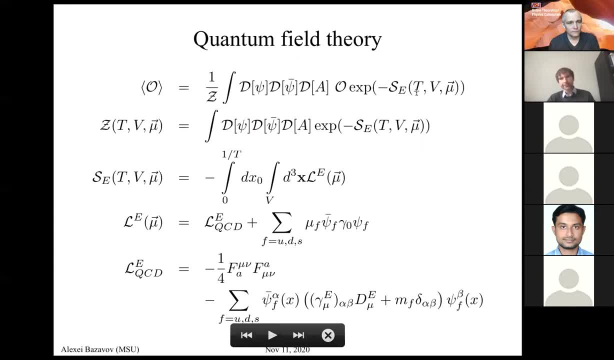 to pi over a, where a is a lattice spacing, And it basically serves as a regularization scheme for these path integrals. So in any case, perturbative expansion of lattice. this is symbolic. One still has to provide the prescription how to regularize those integrals. 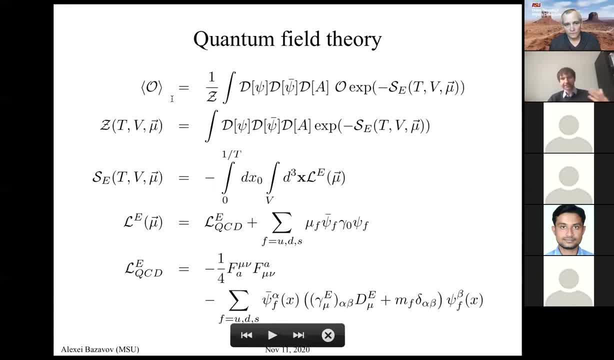 So one wouldn't end up with with infinities And that what took some time to understand, from thirties to forties and fifties, how to deal with those divergences. So lattice is, although we're making space time, discrete. 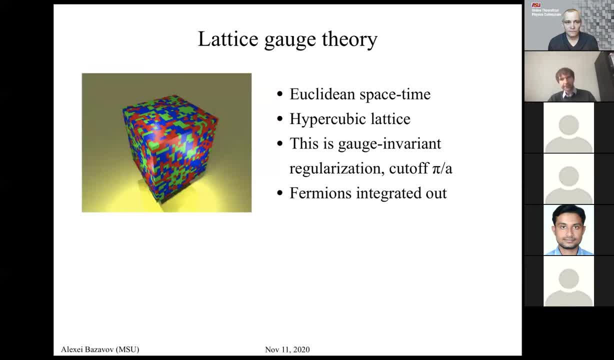 I wouldn't view it as an approximation to QCD, So rather a regularization of QCD, which is more or less on the same footing with any other schemes. It's just done in a specific way And we also take advantage of it numerically. 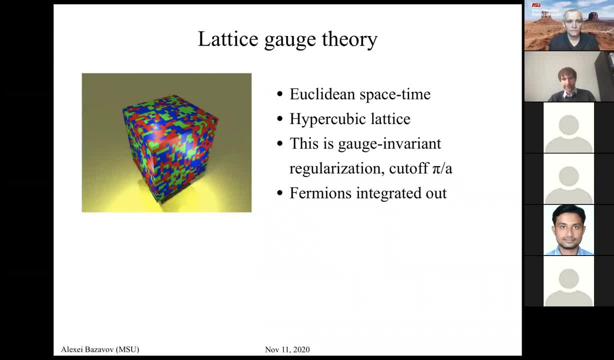 However, perturbative calculations could be done as well. They are less convenient than in the continuum, but it's the main idea. It's not an approximation, It's a regularization scheme. Now, fermions are represented in this formalism by: 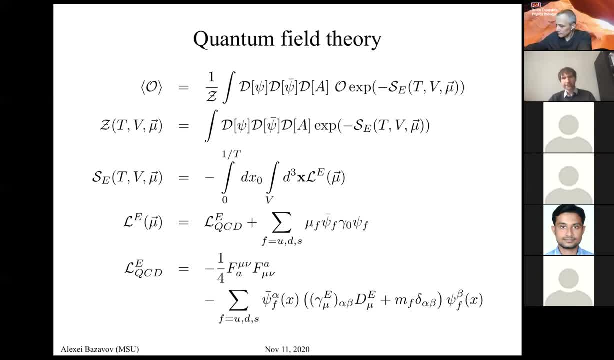 not by usual numbers but by anti-commuting numbers, which are not easy to deal on on a computer And they're not easy to deal with. and they're not easy to deal with. and they're not easy for many reasons. 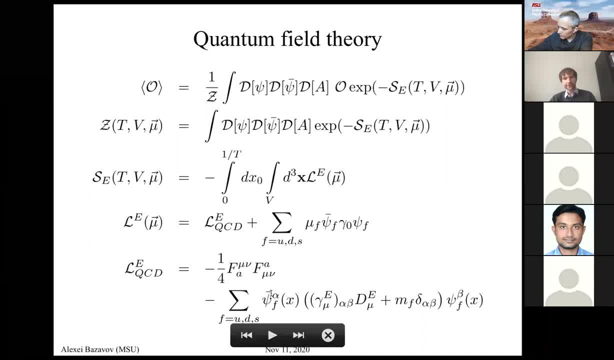 However, typically in the theories we want to study they enter bilinearly. So as a Gaussian type of integral they can be integrated out. It doesn't mean that we omit them, but we just rewrite the partition function only through the gauge degrees of freedom. 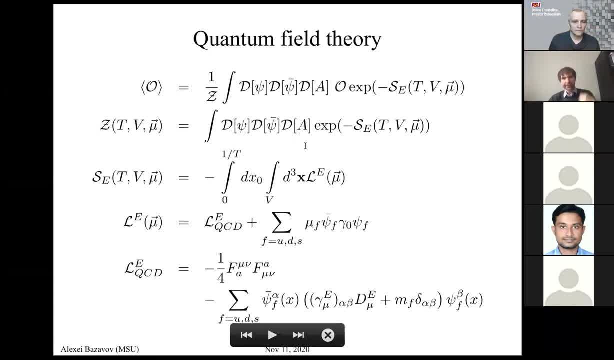 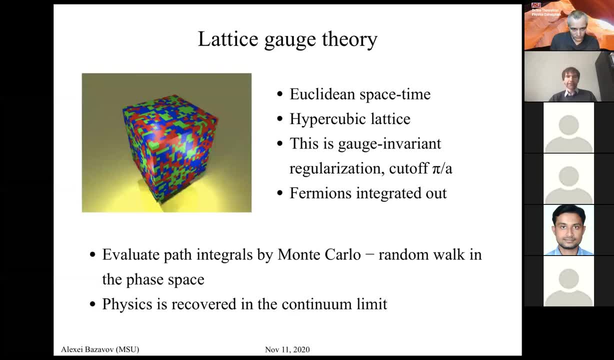 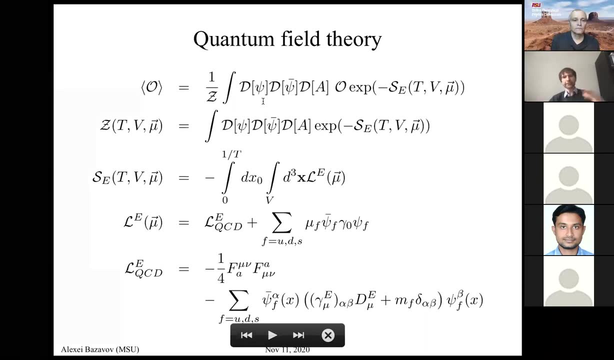 All the fermion dynamics is still in there, but the actual degrees of freedom that we have on the lattice are just the gauge fields. Now, those are integrals of very high dimension. right, Because I need to so, for instance, if I have a finite box. 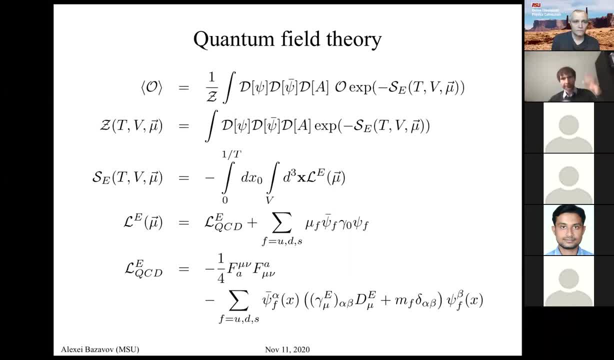 and I take 10 points in each direction, including time. so I have 10 to the four sides of the lattice. So I have 10 to the four points where roughly my fields live And so I need to integrate over 10 to the four degrees. 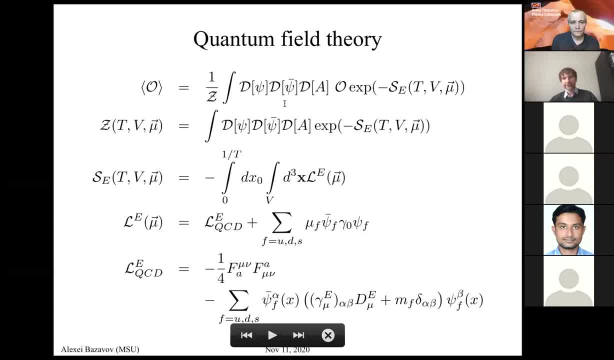 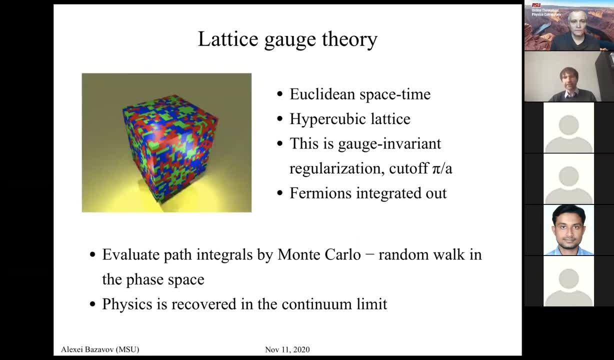 of freedom over whole possible values of them. So there are such vast integrals that it wouldn't be possible deterministically And it would be some sort of NP hard problem because the effort would scale exponentially with a number of degrees of freedom. However, the way out is a realization. 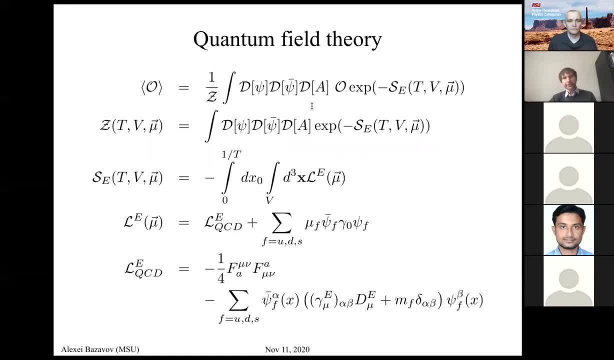 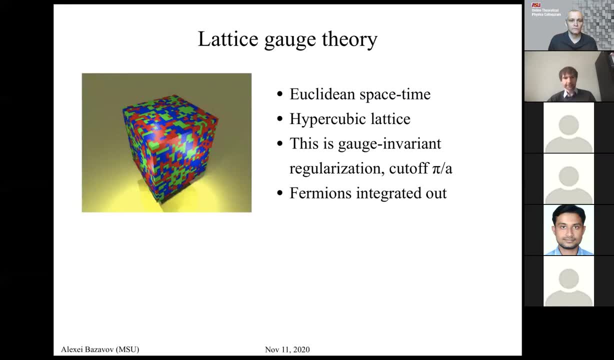 as in statistical physics, that the main contribution to this path integral comes from a tiny region of this gigantic phase space. And that's where, if possible, Monte Carlo methods typically win and provide polynomial scaling with a number of degrees of freedom. So, as long as we can make Monte Carlo work, 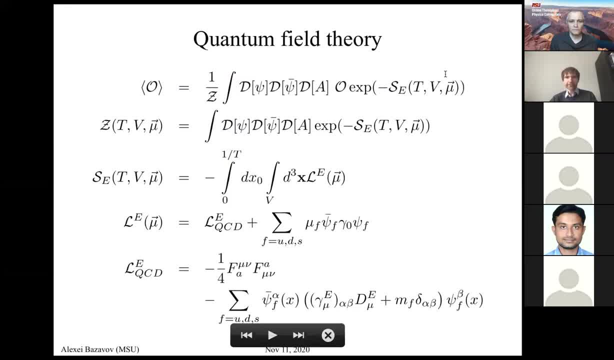 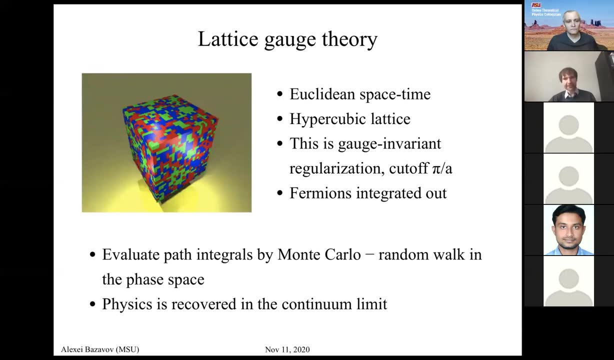 which requires being able to interpret this exponential of the action as probability, which means at the end, the action has to be real. So, for all the problems whether it's not real, like finite density, we have a big problem And that's one of the technical reasons. 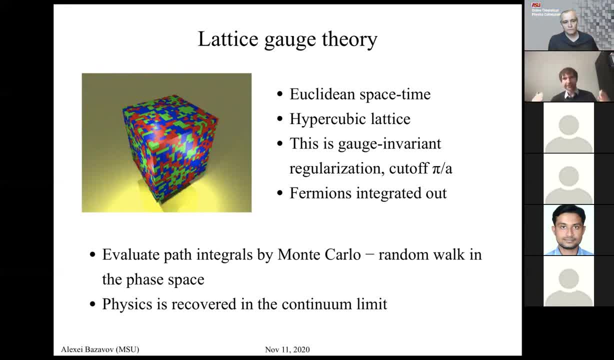 why it's not easy to access full phase diagram of QCD At non-zero variant chemical potential. But as long as we have real action and Monte Carlo works, we can randomly sample the most important configurations of the fields and numerically estimate these averages. 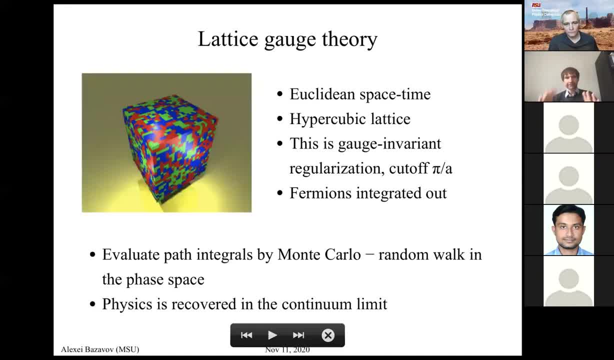 that we want. So that's a rough on one slide, the idea of lattice QCD. What's important, though, is that to really connect to the real world we need the same way as in perturbance in the normative calculation. 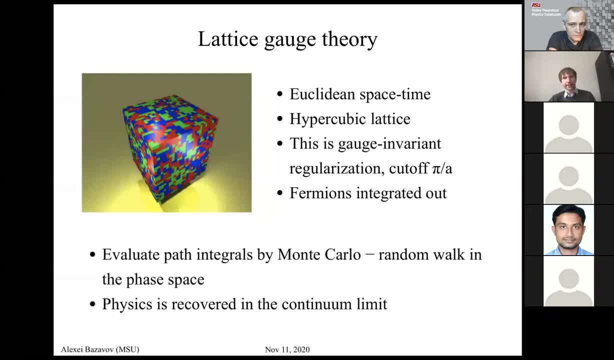 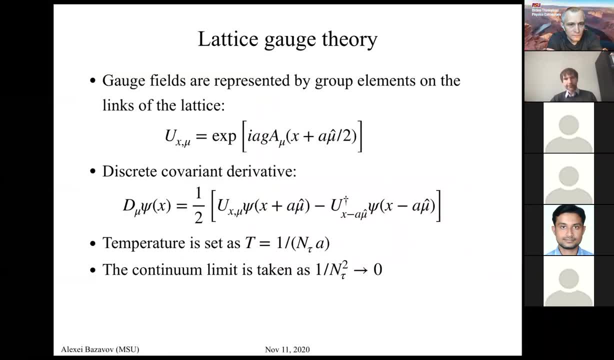 we need to remove the cutoff of the theory or in our case, dial the lattice spacing to zero, And that's important for our calculation. So now, the gauge fields now will have to be represented differently compared to how they're represented in the continuum. 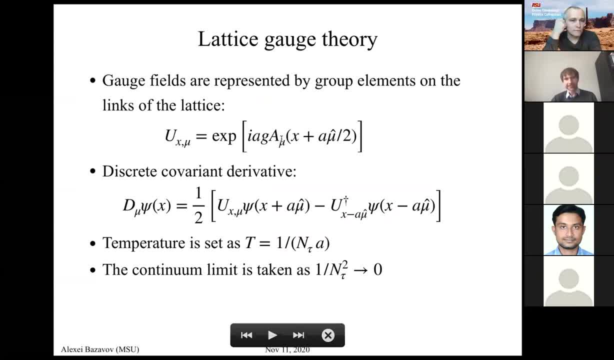 So we're switching from this, say four, vector potential, a, mu to elements of the group. So I will not go into details, but I loosely refer to the number of points in the temporal direction as a cutoff, Because the way we take the continuum limit 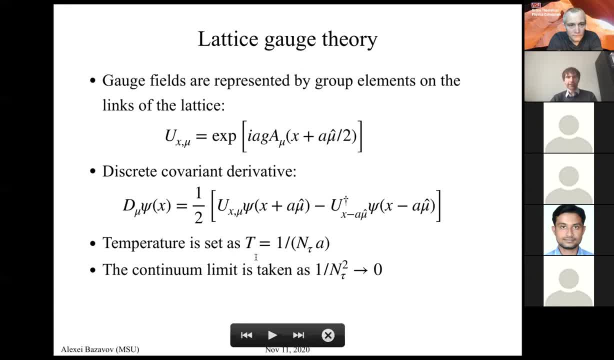 in finite temperature calculations is typically the following: Because the temperature is inverse size of the temporal dimension, We typically change the lattice spacing to cover different temperatures And then the continuum limit we take by increasing the number of points in the temporal direction. What it does, it means. 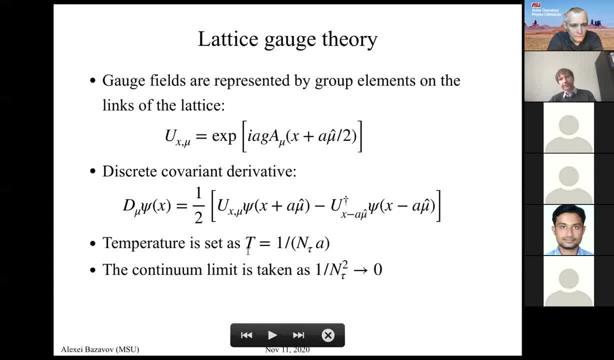 if I go to large N taus, I cover the same temperature range with finer and finer, smaller lattice spacing lattices, And that's what dials the system to the continuum limit. So I will skip that. That was a slide to convince you. 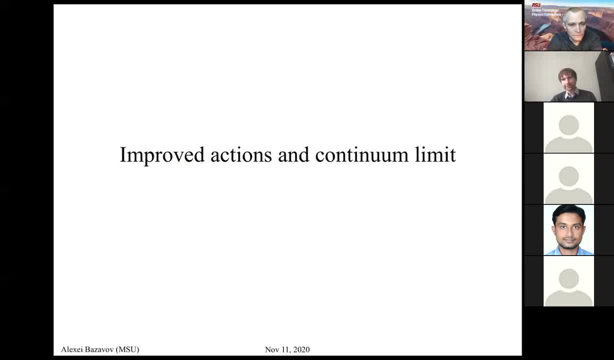 that all this numerical stuff, which has been developed roughly over the last 40 years, works correctly, reproduces a spectrum of QCD and many observables that we can match to experiments. Now what are the technical things that were needed in particular? 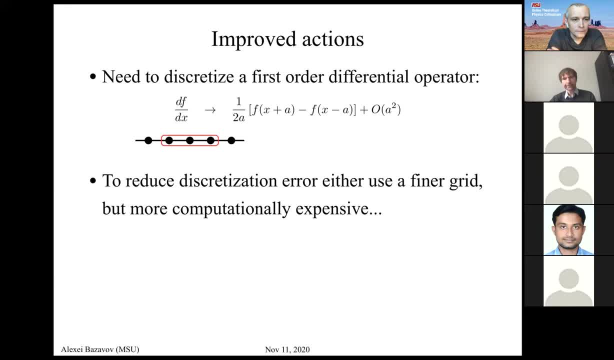 for the program of calculations that I'm describing here. Let me go through this quickly, just to give you some idea. We're doing not exactly this, but something very similar in spirit to this. So if I want to do calculations- say solve ordinary differential equations on a computer- 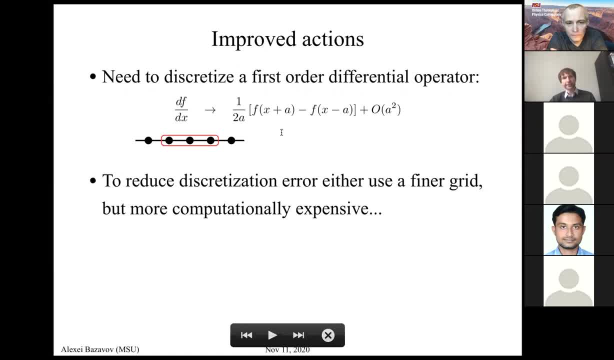 I need to discretize all these derivative operators So I could take some finite differences. but then this means I'm making inevitably some error. And if I take this type of finite difference it would be order of spacing square. So either I need to go to final lattices, 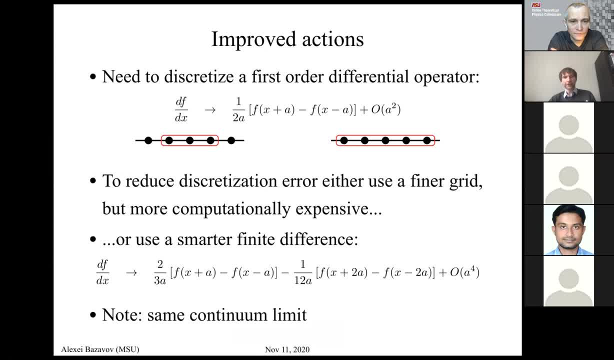 or I have to work with more sophisticated finite difference. So if I modify now discretization of this derivative, I could achieve higher suppression of this error by not so much extra effort. right? Because for instance here, if I stay with this sort of simplest scheme, 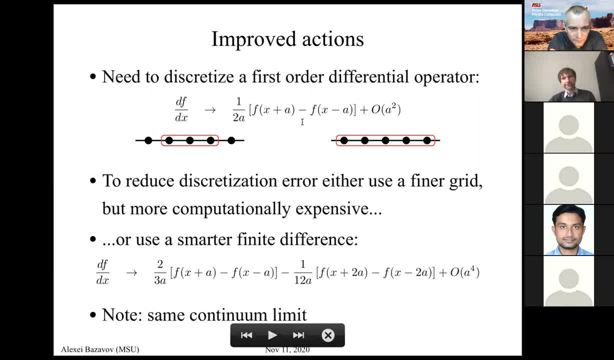 to achieve certain level of error, I have to half the lattice spacing, or maybe take one quarter, and so on. So this means I will have to do many more computational steps on the computer, While here it's a marginal additional effort, but it suppresses the error a lot. 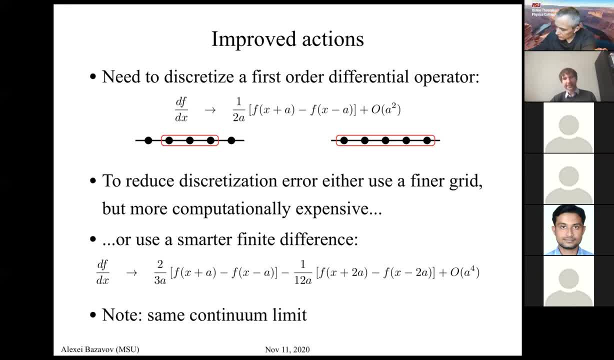 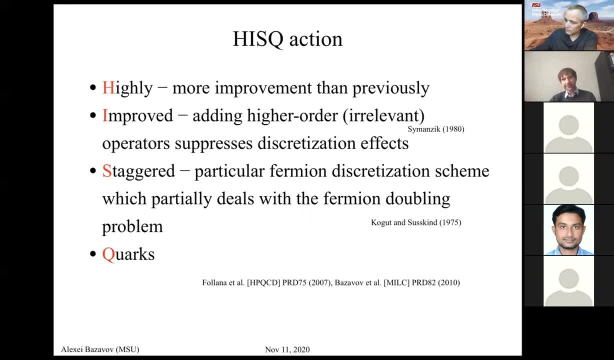 And, what's most important, in both cases I have the same continuum limit. That's important to recover all the physics correctly. So one of the building blocks of this whole program is what we call highly improved, staggered quarks action. So basically, choice of the action. 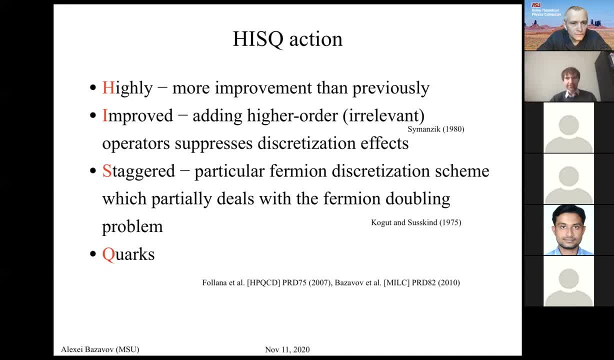 relying on the fact that at finite lattice spacing I could modify. I have one and only QCD Lagrangian in the continuum and one and only action. but I could develop different discretization schemes which would still give me the same continuum limit. 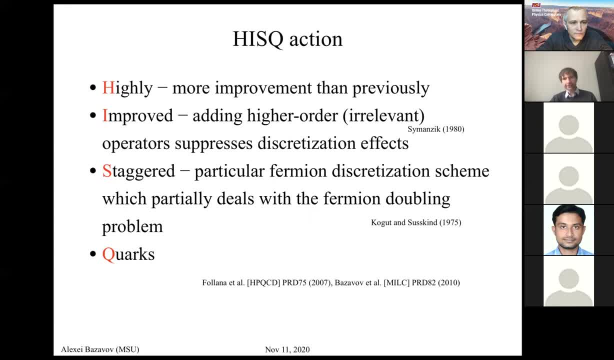 And that can be used as an advantage. And so effort was put into in late 90s, early 2000, into developing better discretization schemes. So we call it highly improved because it's like a second level sort of action compared to what's invented before. 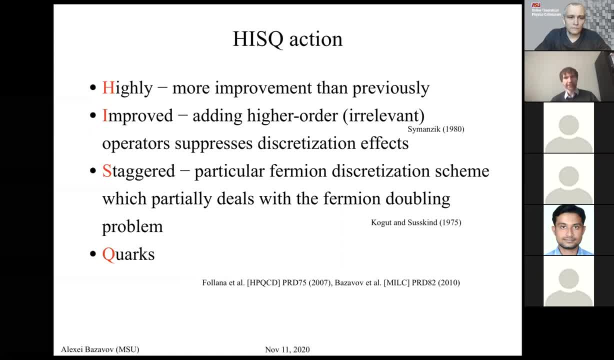 Improved means we modify the action in such a way which does not alter the continuum limit. Staggered is a particular fermion scheme which I'm not covering at all. It's a very technical subject. but fermions overall present many problems in discrete space time. 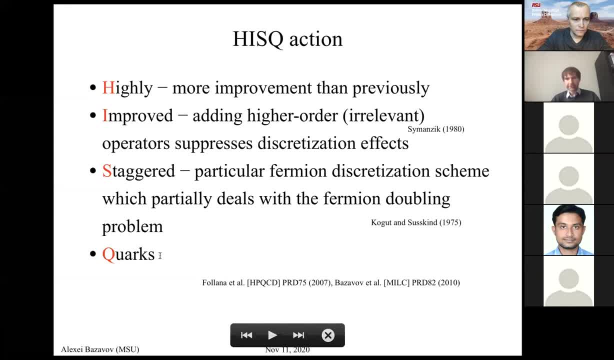 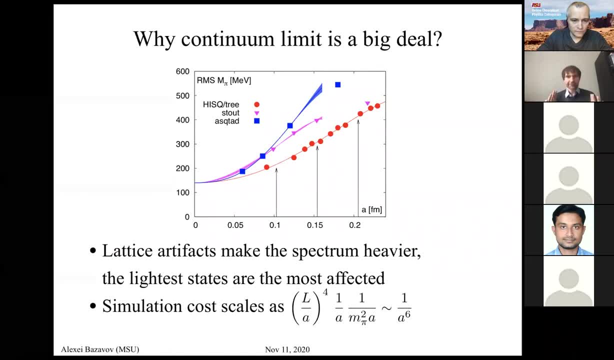 And quarks. of course we need the action for fermions here. So why is the continuum limit is a big deal. So I hope I can illustrate everything as in very condensed way of just a single plot. So remember we discussed at the beginning: 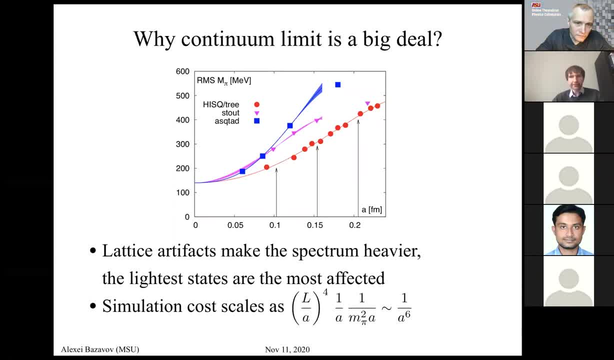 that typical energy scales are on the order of 100 Ne or so and it's a lightest quarks which determine the dynamics in that, in that area, And this is the same thing in the case of low energy scales. So I could ask the following question: 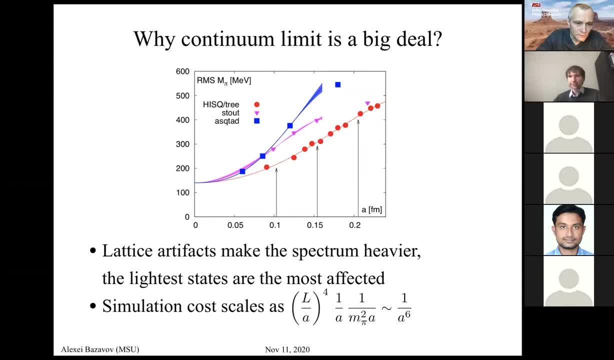 Okay, I'm simulating my, you know, regularized QCD on the lattice. So I'm making some error which is proportional to lattice spacing squared or such. How bad things may be. Now, what I would worry most are the lightest degrees of freedom. 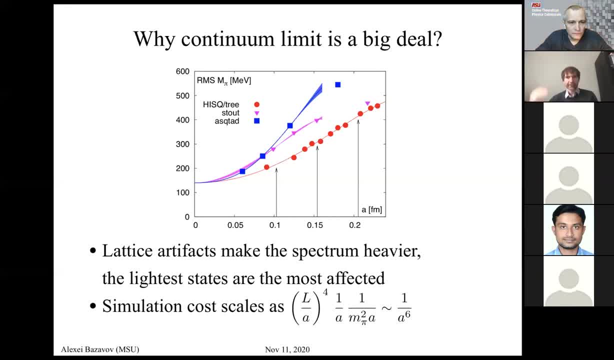 because they may be affected the most. If something is heavy, maybe layering, that is not that relevant. So I can look at what is called here. root mean squared pion mass and the pion is a lowest QCD composite state. 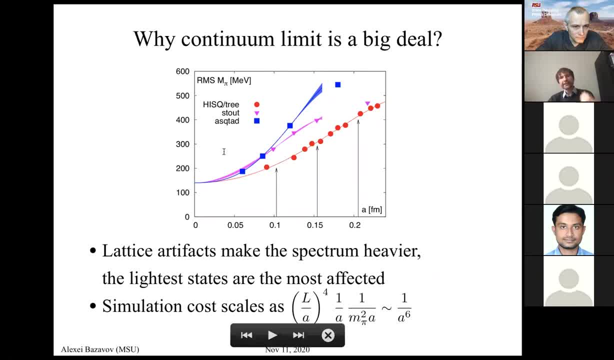 So now in any simulation I have to tune the input parameters, which are bare quark masses, so that I could have some pion mass. And let's say I tune them in such a way that I have 140 MeV pion. 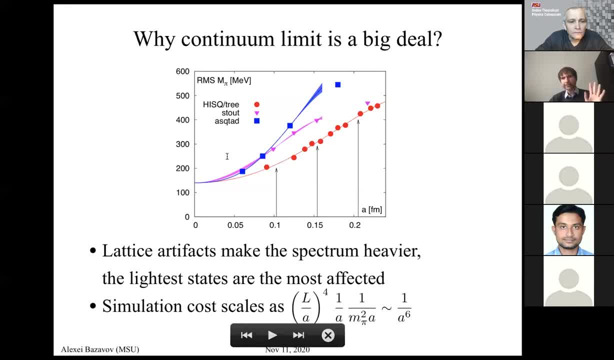 the physical pion and the continuum. Now I'm not here worried about electromagnetic effects, about difference between unique quark masses, So we take it as two degenerate light quarks at some average mass. What's important is sort of being close to those things here. 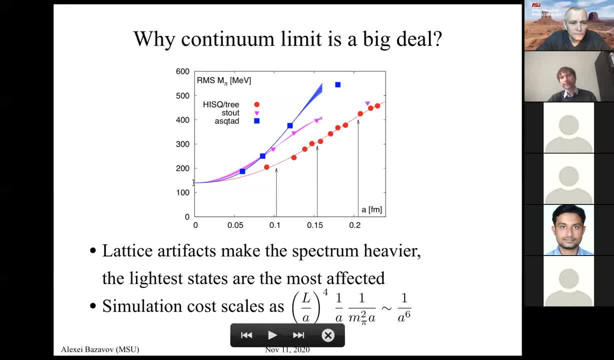 So then I could measure what pion mass I actually have at the given lattice spacing. So the X axis is a lattice spacing in Fermi And these arrows show a typical lattice spacing range that we can computationally measure And I can actually afford. 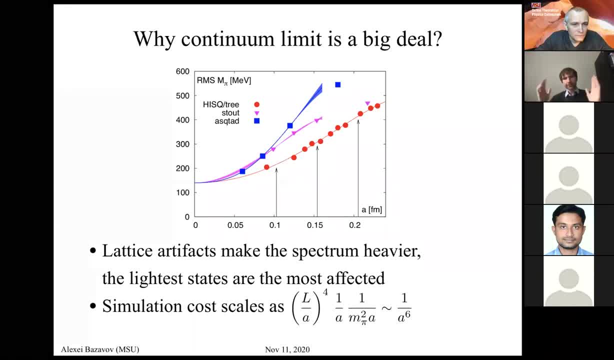 because I have to keep the physical size of the box when I'm doing lattice simulation fixed on the order of two Fermi or more, So I could really accommodate the physics that I want to study. If it's too small, it will distort it. 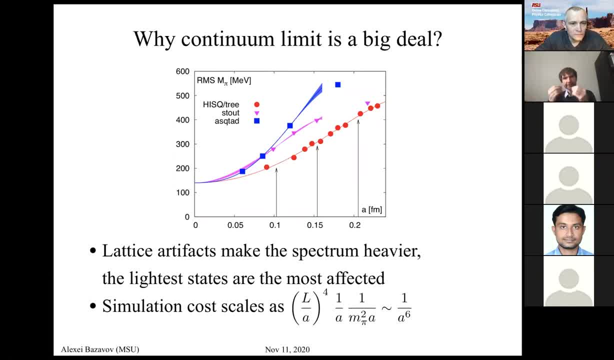 So if I'm going to lattices with smaller lattice spacing, this means there would be more lattice points in the same physical size box, which means more computational effort. So in ideal world I could just go to arbitrarily small lattice spacing and do the computations there. 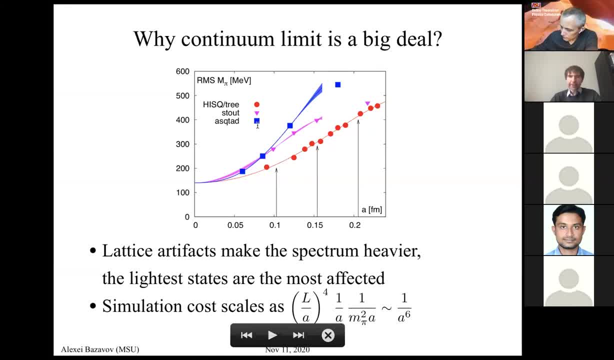 but it's not feasible, And so the effort was put into improving the actions as I described before, And what this plot shows is what root mean squared pion mass I would get with three types of improved actions, So what is called HaStat. here is something developed. 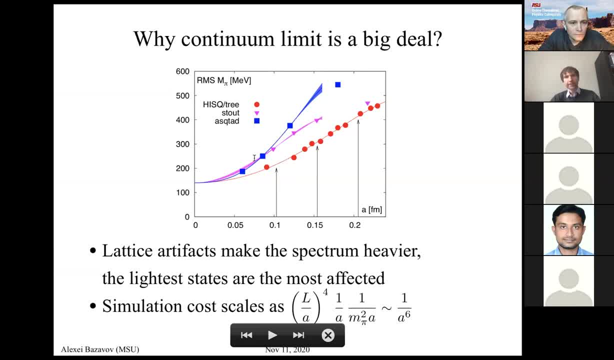 in the late 90s and was used very successfully. But here on this plot it shows that that's the one with the largest cutoff effects. So pion the root mean squared pion that my simulation has is actually very heavy on the scale of lattice spacing. 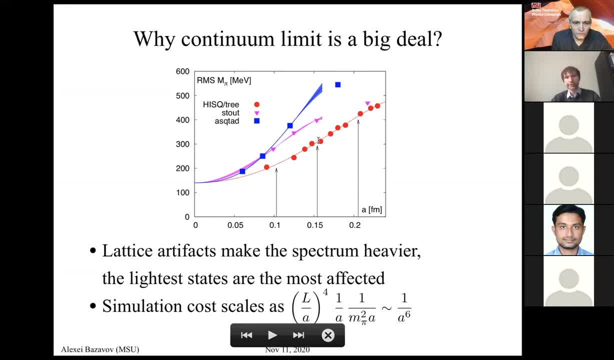 that I can afford to work. So, for instance, at 0.15 Fermi lattice- spacing lattice, it's half a GeV mass. So this means the spectrum of this regularized QCD is very distorted. The details depend on the action that I'm choosing. 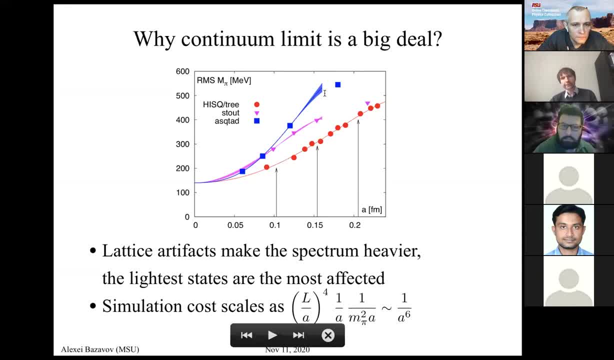 but it's not 140 MeV pion that I want. So certainly it would affect the dynamics if it's governed by the slight degrees of freedom. Now LEN1 has a choice: either very fine lattices but computationally prohibitive. 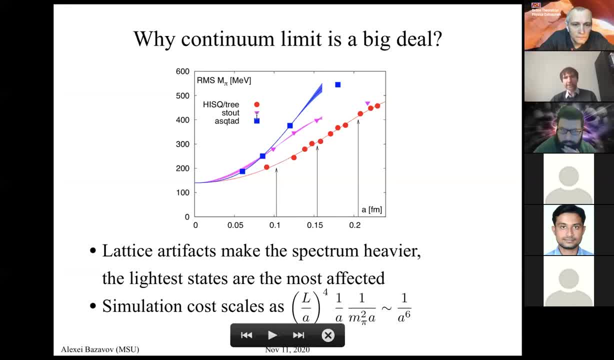 or smarter discretization schemes. So the next stout action used by other collaboration, Wuppertal, provides better cutoff effects, less cutoff effects, And then what we are using, highly improved, staggered in this red line, And so it's one of the best choices. 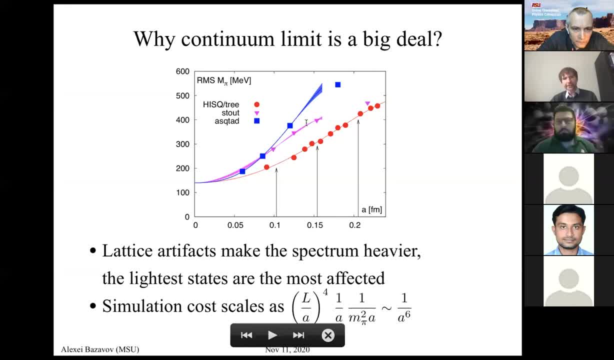 Stout has various variants. It can be improved further. So there could be variants of stout action which behave comparably to this red line. But the main message here: it's a big deal to do this improvement, to be able to do this calculation. 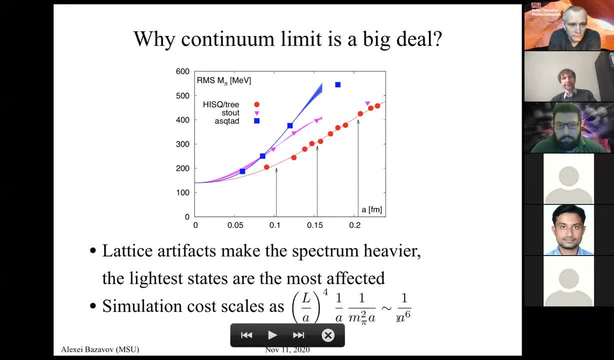 because the simulation cost typically scales at least as one over lattice spacing to power six. So it's very costly And for some quantities, like equation of state, it's something on the order of one, on the order of one, over lattice spacing to power 10.. 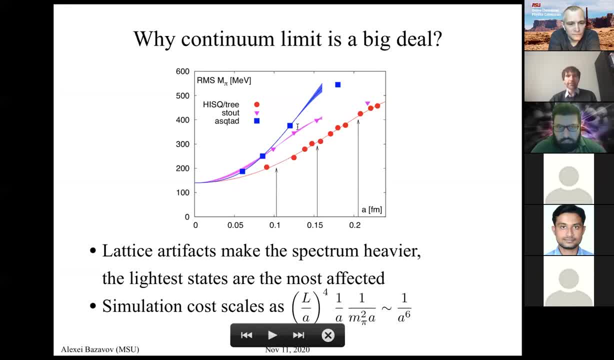 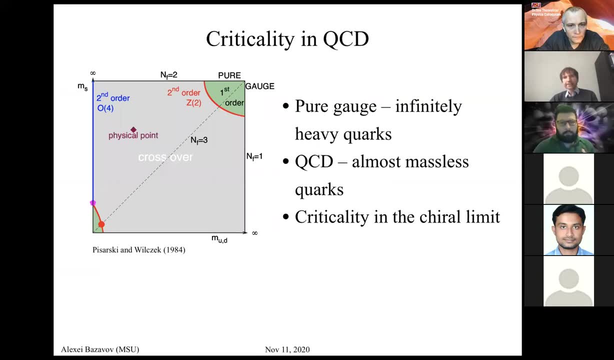 So it's very costly to go to the left on this plot, but it's much less costly but requires some theoretical effort to bring these curves down. So hopefully that illustrates a point Now what we can expect in QCD in terms of the critical behavior. 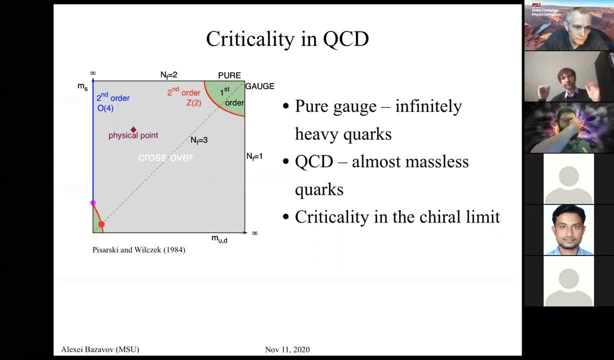 So the real world phase diagram, how phases in QCD behave as a function of temperature and chemical potential in real world, meaning with all the constituents of their physical masses. that what we have seen before. However, theoretically, we can ask another question is: 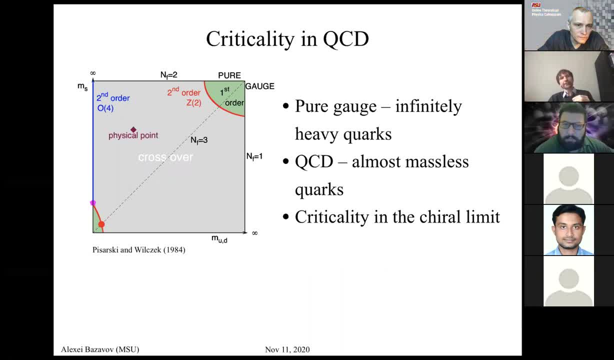 how critical behavior in QCD changes if we change the quark masses. So there is one and only physical point where masses of light quarks which are on the horizontal axis, Again at this scales we take UND quarks which are as degenerate. 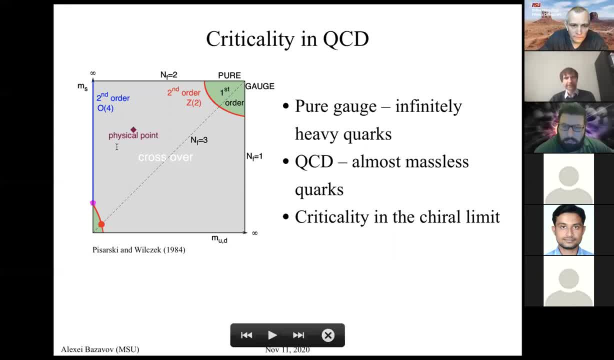 We neglect all the isospin breaking and stuff like that, And then we have the strange quark, which is somewhat heavier, So it's on the vertical axis, And then we have that phase space on what would be the order of finite temperature transition in QCD. 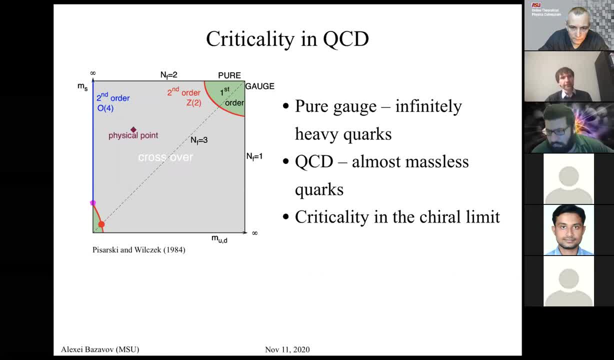 at zero bearing chemical potential as function of the masses of the constituents, So what we call pure gauge, which was historically studied a lot because it's much computationally cheaper. So this means infinitely heavy quarks. Questions from junior audience. So infinitely heavy quarks. 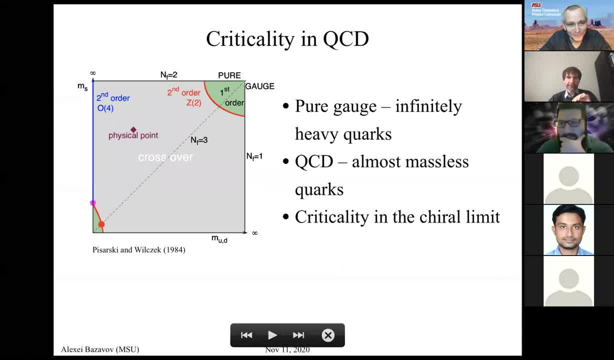 what was shown in lattice calculations in the 80s- 90s is that it's a region where we expect first order real phase transition, And theoretical arguments were given that we also expect first order phase transition when all the three masses are dialed to zero. 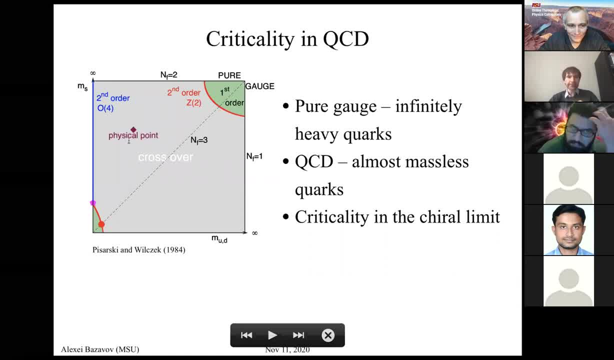 in the other corner And then somewhere in between, including the physical point, we expect a crossover region. That's what we observe on the lattice And the contrast here. it's all not to scale, but the idea here is that we have very well studied pure gauge regime. 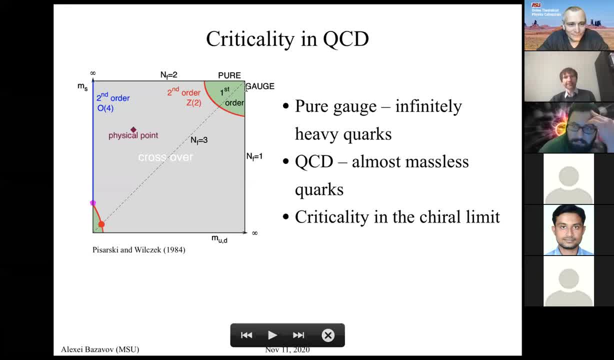 where quarks are essentially infinitely massive, But the real world regime is dealing with almost massless quarks. So this point is sort of close in some quantifiable sense to the vertical axis And we expect that if we go along so we keep the strange quark at the physical point. 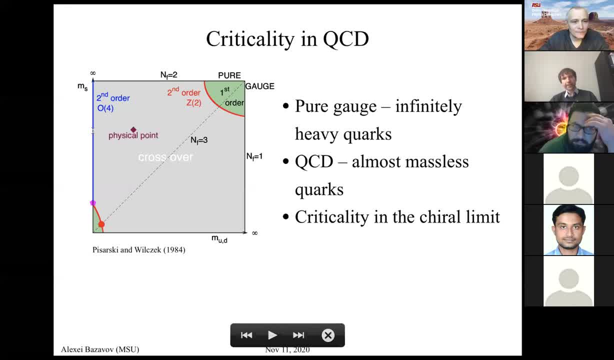 and we dial the light masses to zero, we enter the real phase transition regime. So in other words, in what we call two-flavor chiral limit, when UND masses are zero, we expect real phase transition, real critical behavior. So the chiral condensate. 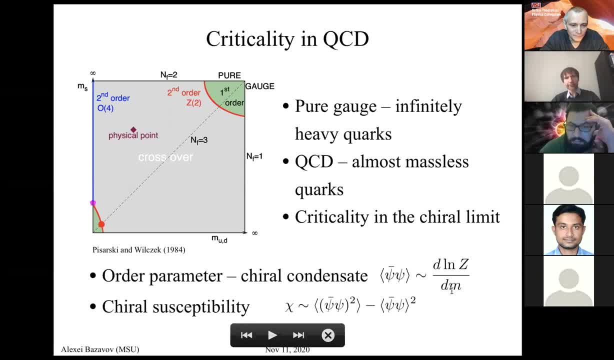 the derivative of the free energy with respect to the quark mass can serve as an other parameter for probing this. breaking of the chiral symmetry in the hydronic low temperature phase and restoration in the high temperature phase, very much like magnetization in spin systems. 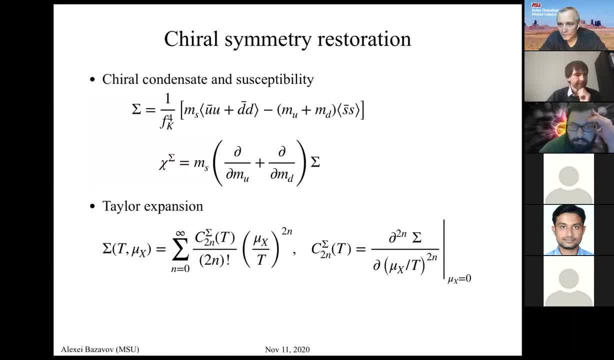 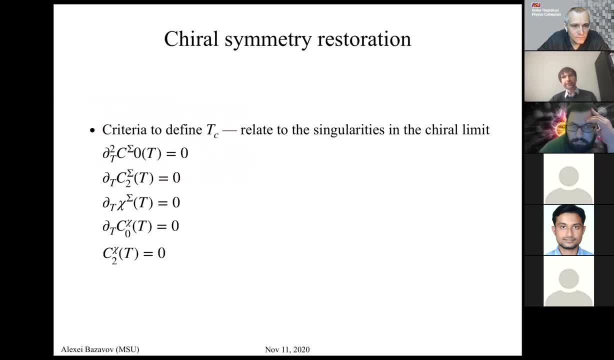 So this is a technical part. Maybe I would skip it for the interest of time. So just take my word for it that we can construct various quantities which behave as some sort of order parameter or its derivative, which is like a susceptibility, And by studying these quantities, 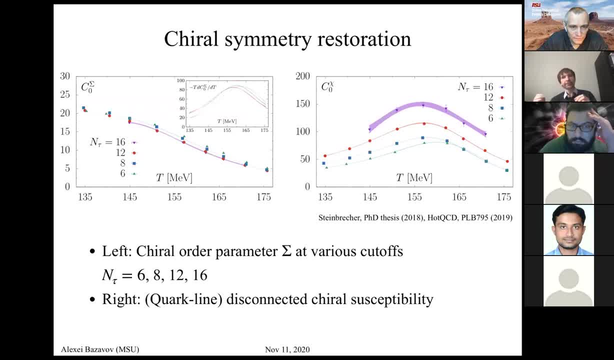 we can define what we call chiral crossover temperature from the consideration that, although at the real world, quark masses, there is no true phase transition, there are no singularities, We have a quantity which at least will develop a singularity in the chiral limit. 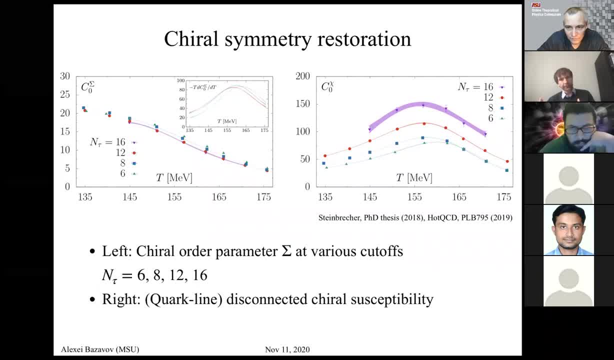 And since the light quark masses are small, we can argue that this is the right quantity to define the chiral crossover temperature form. So if we look at the condensate itself, the analog of magnetization, then it acquires some non-zero value. 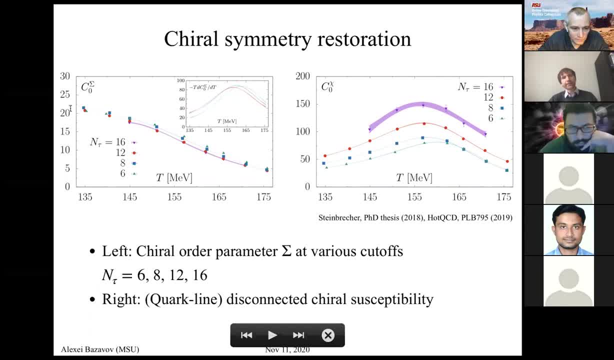 There is arbitrary normalization here. in a way, There is a non-zero value in the confined phase And then with increasing the temperature it starts to melt and goes to zero. And here, as I mentioned earlier, I treat n tau the number of points. 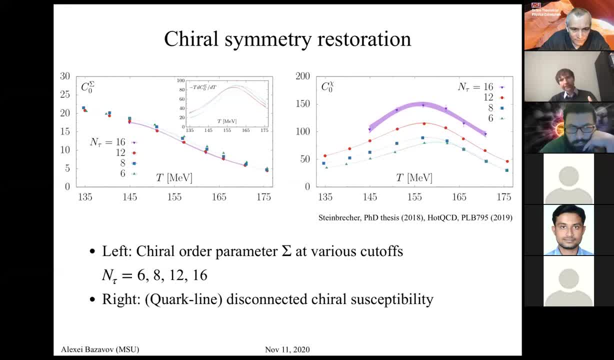 as a cutoff. So the larger the n tau, the closer things are to the continuum limit, And so what this plot is showing is basically calculation at various cutoffs, and then we do the continuum extrapolation and extract the results out of that. So now, here we see, the behavior of the order parameter. 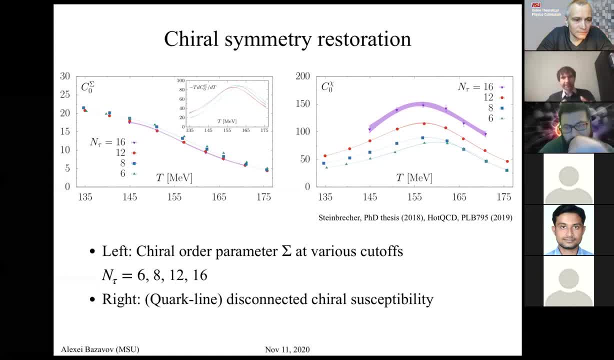 or would-be order parameter in the chiral limit, Because remember, here at the real world quark masses there is no phase transition. So would-be order parameter in the chiral limit, But then it's easier to look at its derivative with temperature or mass. 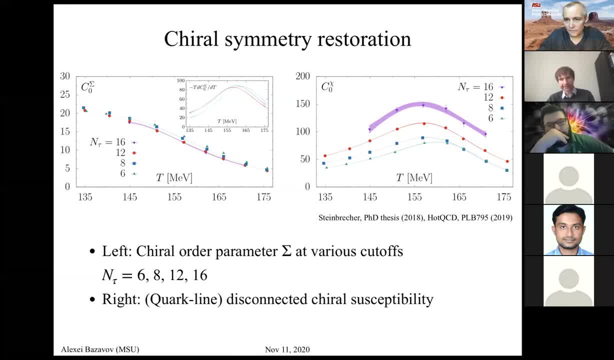 or with chemical potential. There are different mixed susceptibilities one can construct, So one of them is chiral susceptibility itself. So this is a quantity which develops the peak with this cutoff And it would diverge if we take the chiral limit. 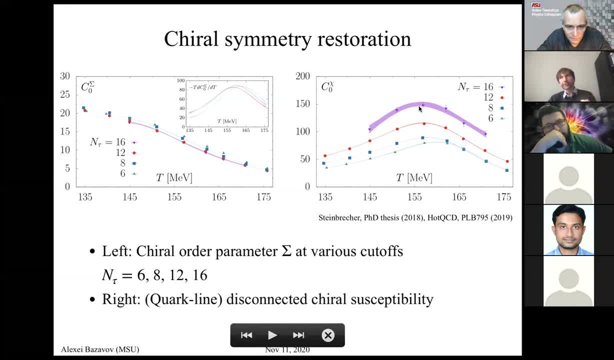 And so this is something that we started calculations with Hisk in early 2000.. And I think I actually visited Arizona State in 2013 when there were fresh results on the chiral crossover. So the temperature and stuff. But then lately it has been updated. 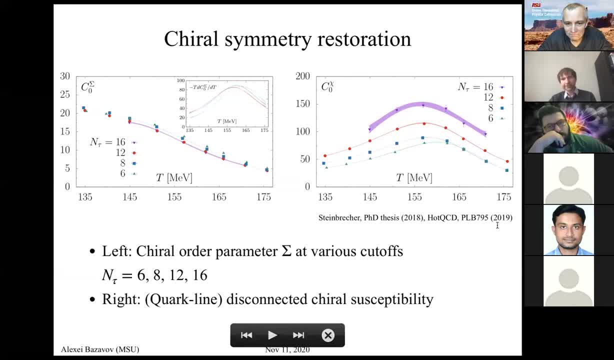 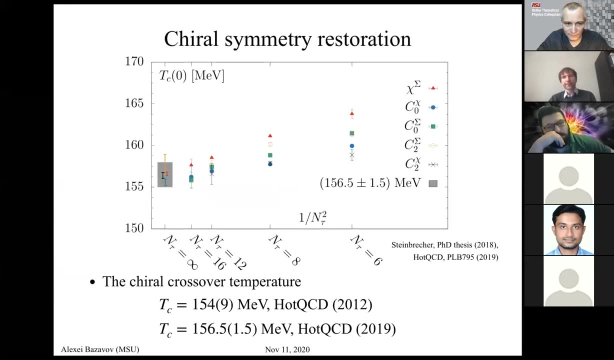 So these are plots and results from 2019 hot QCD paper, And the vital role was played by Patrick Steinbrecher, a PhD student in Bielefeld at the time, And so the end result is that, by looking at those various susceptibilities, 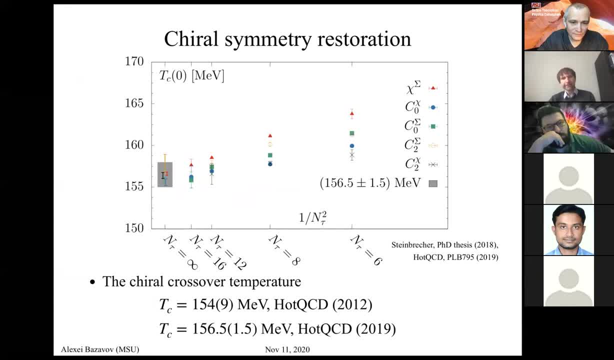 one could sort of observe that they, even though we're not dealing with a genuine phase transition where all these quantities have to diverge, at the same point we're dealing with a crossover where they potentially may be scattered in some range. Nevertheless, at the end they're all compatible. 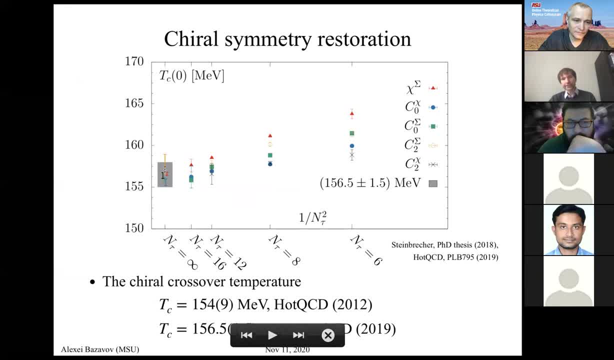 and we can take the average as a value for the chiral crossover temperature. And so our now old result from hot QCD. I have this box here which is on the way Well, and it's not movable for some reason. It's okay. 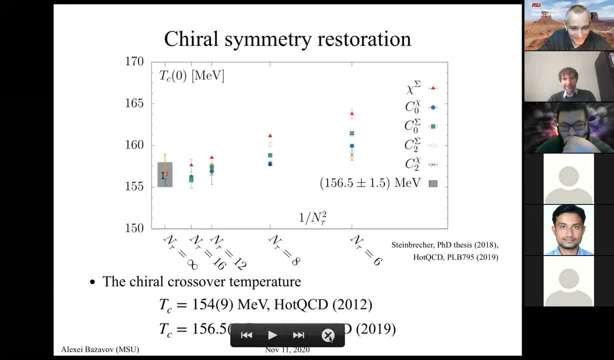 So, and if I press this it will just switch off the slideshow regime. So, in any case, our old result is 154 plus minus nine MeV, with large error, And then it was updated to 156.. So 156.5 plus minus 1.5. 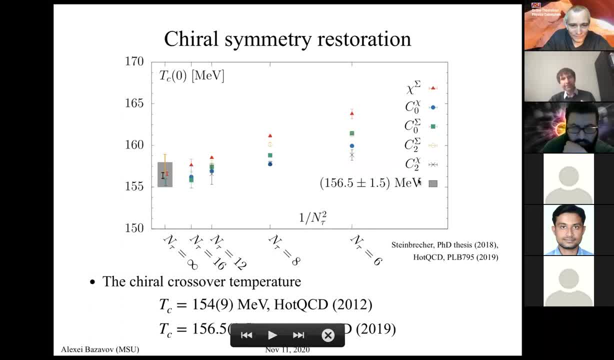 And it's not just updating the precision, It's many more quantities related to this transition region which are much better understood. We're really have robust control of the continuum limit here and things like that. So well, if I don't touch it. 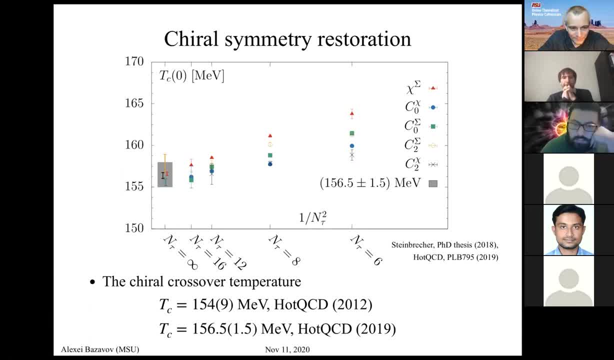 maybe it will disappear. So any questions? by the way, is there? As I say, I'd be happy to be interrupted. I don't want to- So far, there were no questions from the audience. I do have some sort of smaller questions. 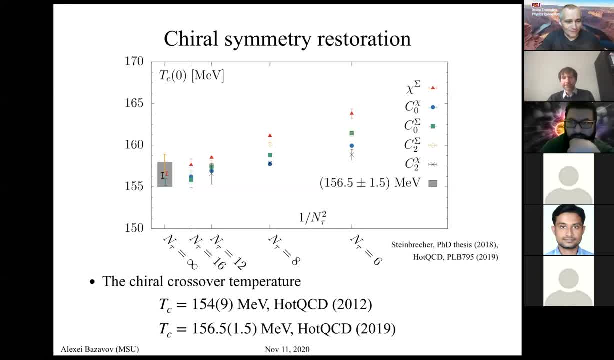 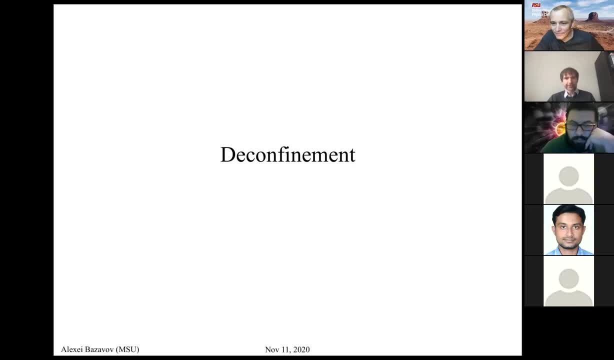 but I would rather keep them until the end. Okay, very good. So LAN deconfinement: Okay, we discussed that. we have the confined phase at low temperatures and we expect deconfined phase with almost free eventually- quarks and gluons. 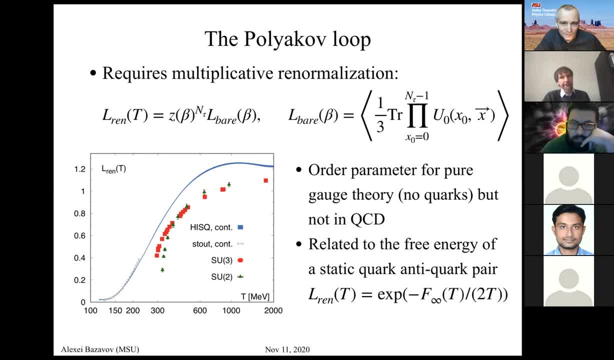 at very high temperature, How we can look at this phenomena from this thermodynamics perspective, So in pure gauge theories, the Polyakov loop, which is a world line of a static quark. So if we have a medium where we insert a static probe charge, 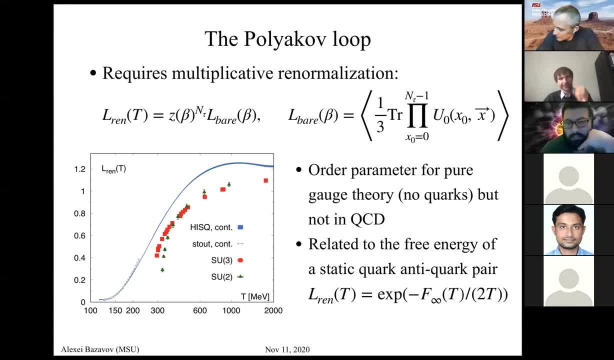 cannot equilibrate with a medium and we just study its free energy basically, or the Polyakov loop itself, which is the exponential of the free energy. Then, in pure gauge theories, at infinite quark masses, we expect genuine phase transition, And that's what's shown on this plot. 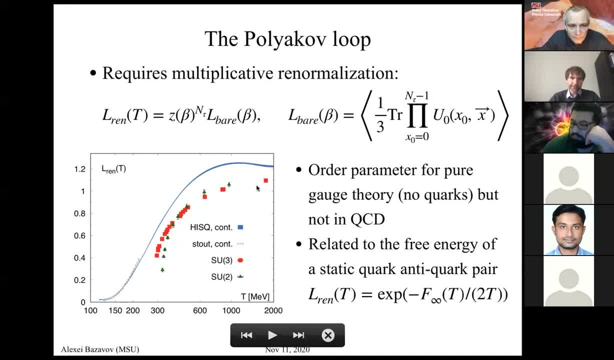 There are many points which are not plotted, but the idea is that if we look at SU case, we expect second order, so continuous transition. So I would sort of connect this dark green points to zero, So the Polyakov loop. the order parameter is zero in the confined phase. 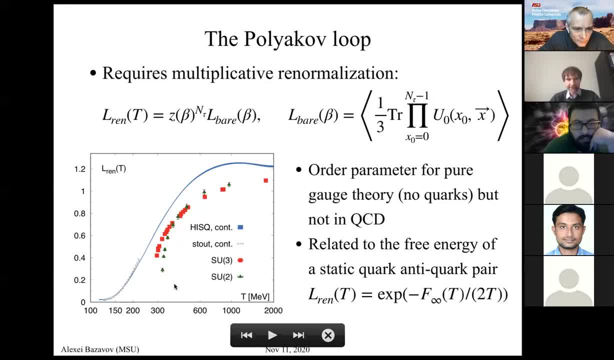 And then it's non-zero in the de-confined phase. So it's also similar to magnetization, serves as an order parameter and such. Then in SU there is a first order, So it's discontinuous. So I could imagine okay. 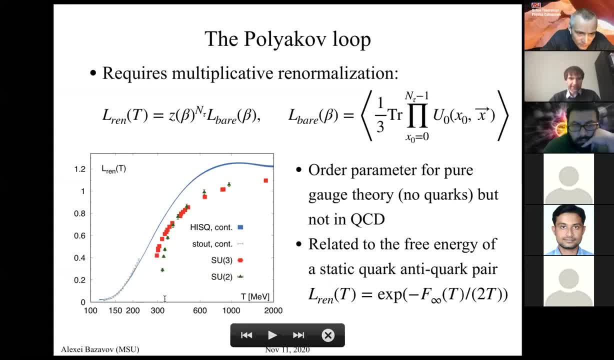 I have these points at high temperatures and there is a gap and it's zero in the low temperature phase, But in QCD it's relatively smooth. Now, the precise shape of this curve is controlled by renormalization conditions, because this property, this quantity, is a 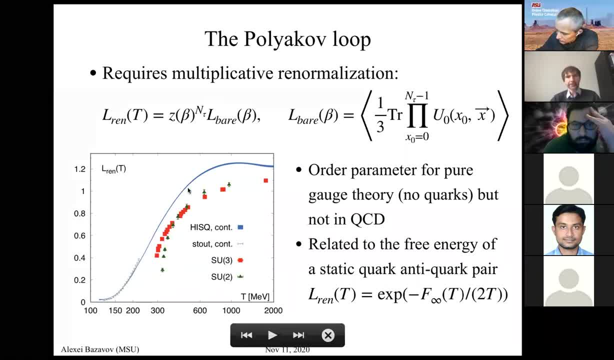 Polyakov loop has to be renormalized and that actually alters how exactly this curve will look. But at the end we see, okay, there are still some region of relatively rapid change in this quantity And, in a way, one of the questions one may ask. 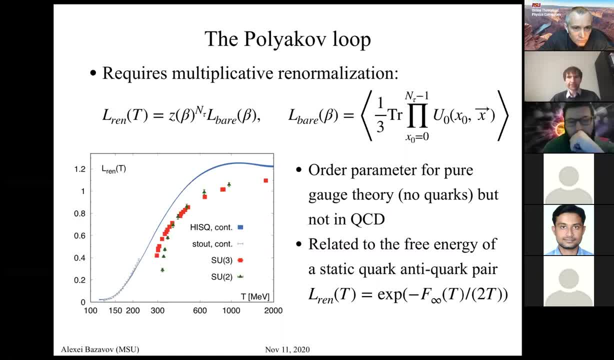 okay, can I? can I really define some de-confinement sort of temperature out of this? I discussed how we can define the chiral crossover temperature based on the consideration of real singularities in the chiral limit. Here the situation is a bit more obscure. 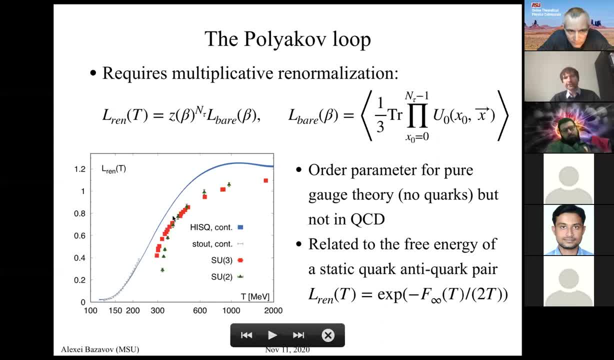 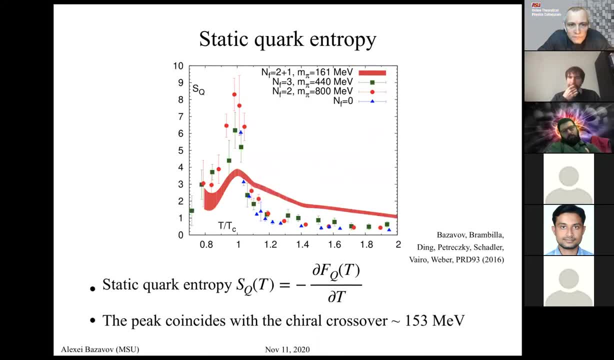 It's a purely gluonic quantity. in a way It's not immediately related to singularities in the chiral limit. However, one can look at the difference in entropy between the equilibrated medium and the medium with inserted static quark in it. 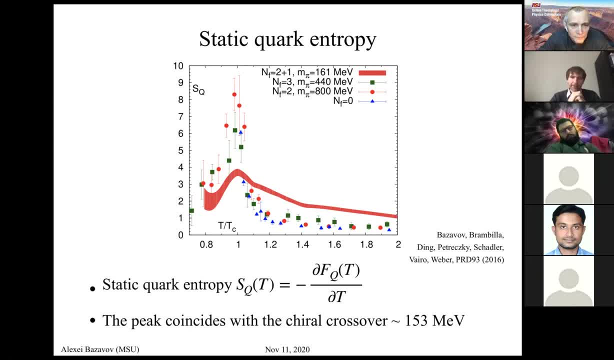 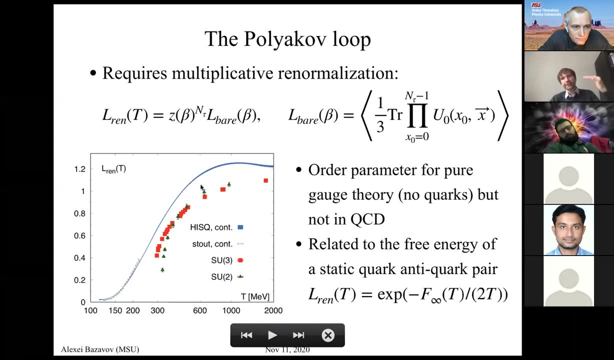 So static quark entropy, And then this quantity, because it's a derivative of the free energy for static quark. it eliminates this dependence on the renormalization scheme because essentially this dependence is basically manifestation of the fact that free energy is defined up to a shift. 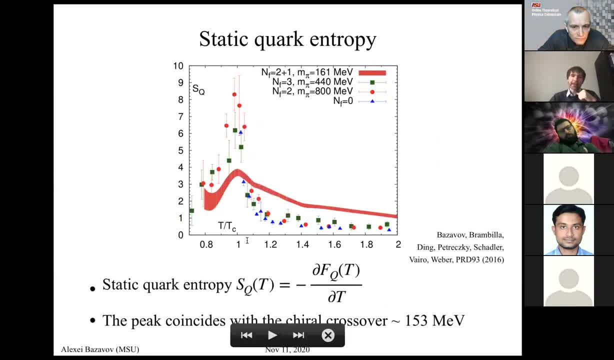 So here it's eliminated, And one could look at the peak of this quantity. Now, what this plot shows is calculations at, you know, different quark masses with slightly different particle content And, for the case of pure gauge theory, no fermions at all. 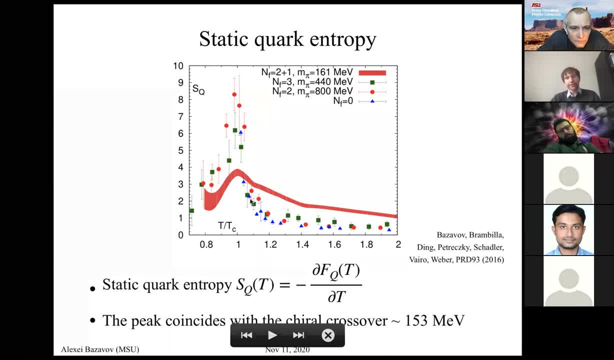 where there are real singularities and stuff. So what was observed? this is a work not done by what GCD, but by collaboration center in Munich. So the vital role here was played by Johannes Weber, who worked with me as a postdoc. 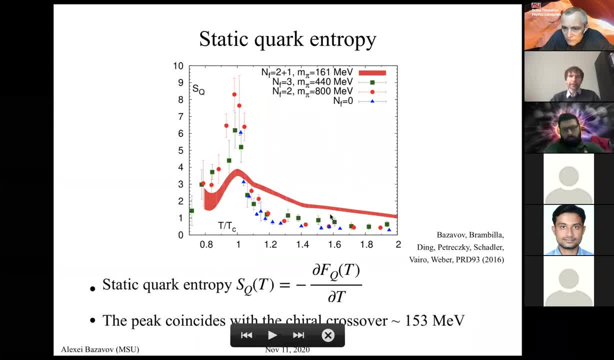 and move on to other position. So recently, So surprisingly somewhat, the peak of the static entropy, which we can take as another definition of some sort of crossover temperature, happens very close to the chiral crossover. There is no immediate relation. 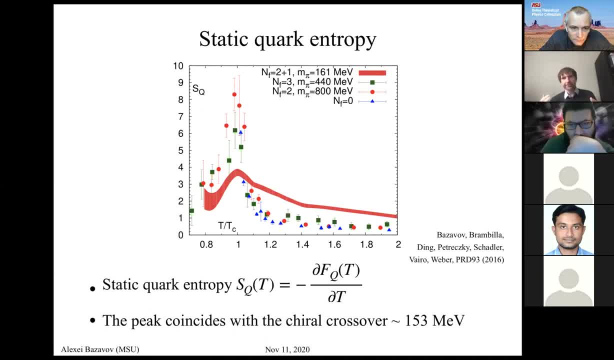 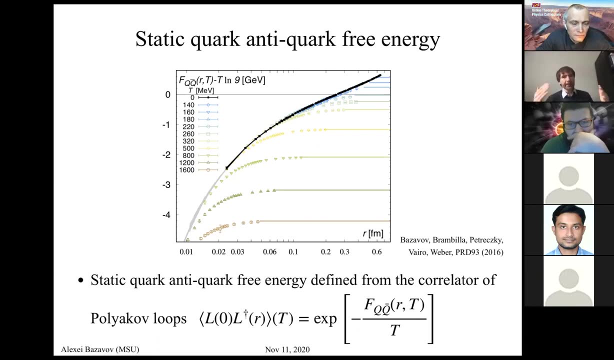 between those quantities. However, there is, you know, certain intuition that something happens around 150 MeV on the order of pi mass. So also very briefly, I will sketch the, if we now look at the pair, not just a single quark- and its word line. 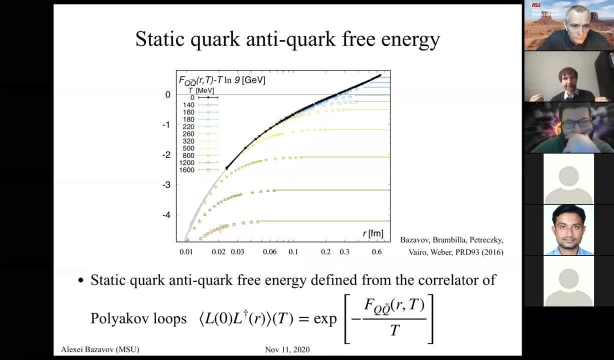 but pair of static quark and anti-quark, something that I started with as we look at the zero temperature static work potential, which has Coulomb behavior at short distances, but then in QCD has this confining linear part. This is something we can extract from a correlator. 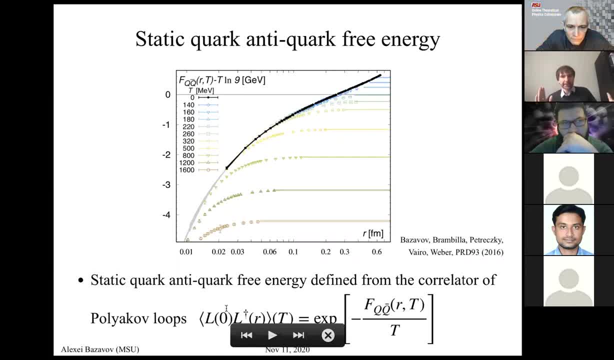 of the Polyakov loops, separated by distance, r, And what we expect by analogy with electromagnetic plasmas is that they are in QCD. we have a long range, basically infinite range interaction, but medium at finite temperature would screen it. 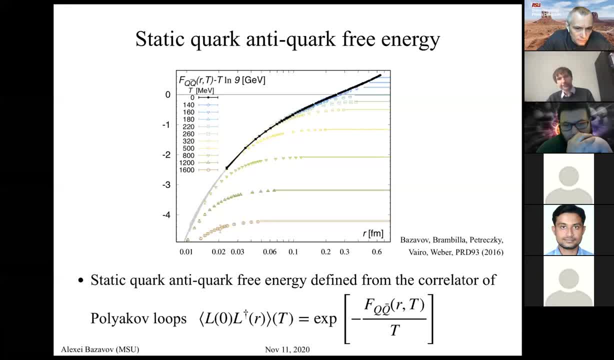 And so the potential becomes finite range. very similar effects happening in QCD, And so if we'll start with zero temperature static potential and then start dialing the temperature up, we will see the screening effects which flatten it off. 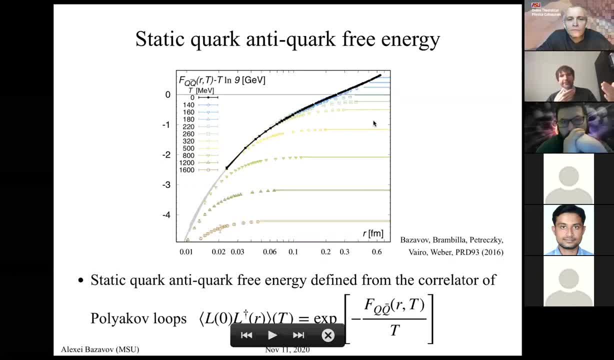 meaning that at some distance, these constituents no longer see each other and interact, and at higher and higher temperature, this screening happens at shorter and shorter distance. Again, there's much more to this phenomenon, but it's one of the ways to look at. 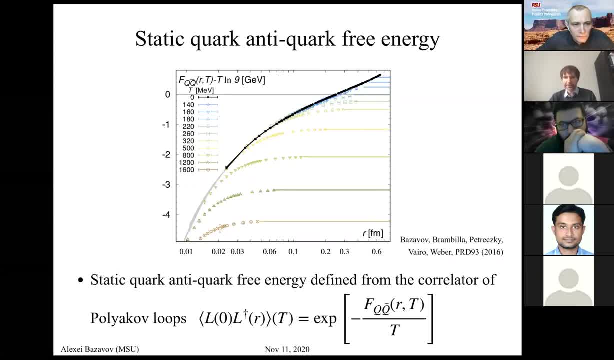 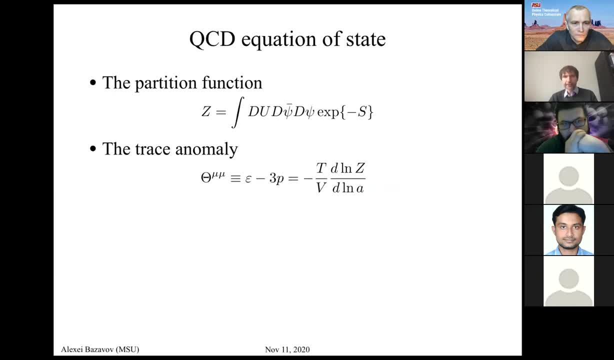 at deconfinement happening at finite temperature. Now let me skip the fluctuations, because I would really like to discuss the equation of state and some new developments there. So we talked about certain signatures of deconfinement and chirosymmetry restoration. 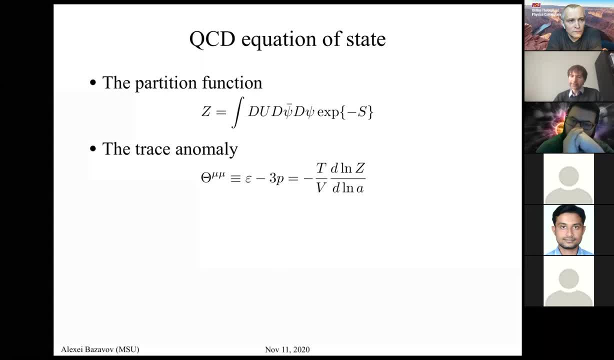 when going from confined to deconfined phase. Another interesting observable and something to describe QCD thermodynamics is the equation of state. So we have the partition function now. it's written in shorthand notation, but basically same as before. 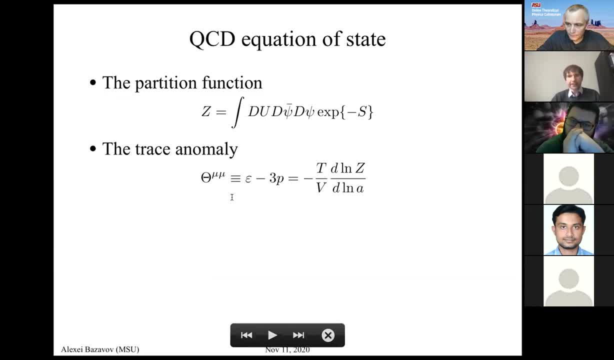 and the quantity that we typically start with in lattice calculations is the trace of the energy momentum tensor, which in this language can be rewritten as a derivative of free energy, with a lattice spacing which naturally gives us the. let me have a better slide. 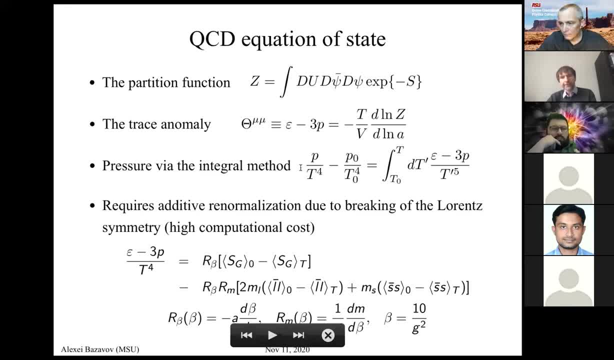 maybe I'll show everything at once Where this quantity we can directly extract from the operators, which are easy to calculate on the lattice. However, it requires renormalization due to additive divergence. So what it means in practice is that to 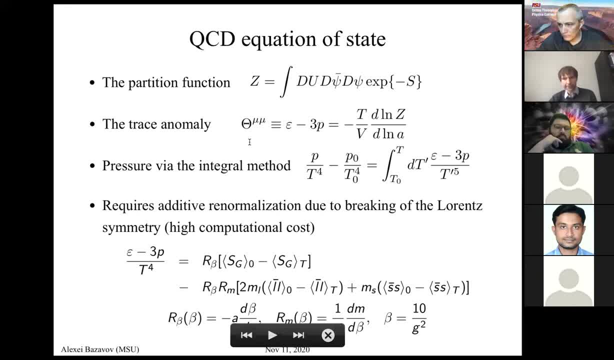 it's one of the most expensive things to calculate on the lattice, at least the way we're doing it. There are some alternatives being recently developed. We'll see how those things go, But so far the most robust method is directly subtracting the divergences. 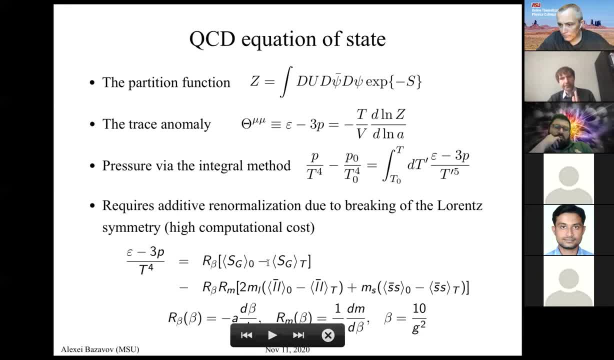 by performing the same calculation, meaning with the same bare parameters, same quark masses, same bare gauge, coupling at zero temperature lattices and finite temperature lattices Because, remember, temperature enters in a way through the geometry, It's a compacted temporal dimension. 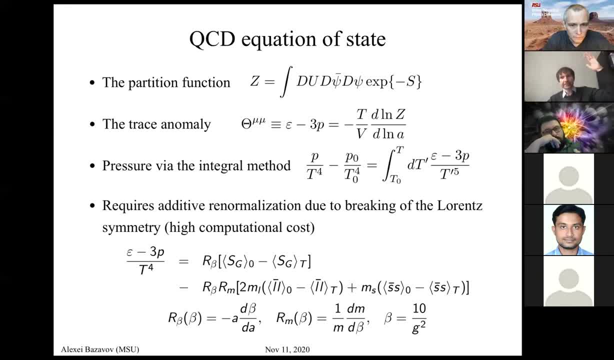 while zero temperature, we're saying, okay, it's large enough to be considered infinite, And so this means we calculate the, the gauge part of the action, at zero and finite temperature. We calculate this Fermi on condensates. It's the same as what's called slightly differently. 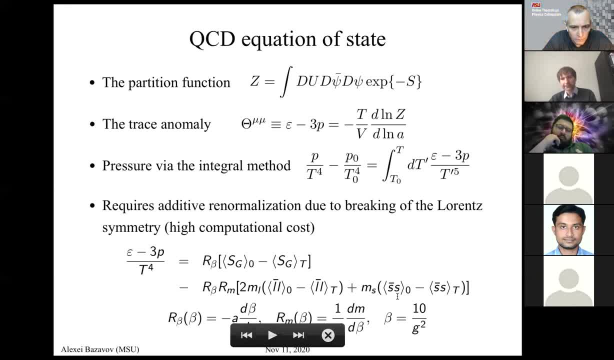 but basically this would be all the parameter for chiral symmetry and chiral limit and so on. Then they're multiplied by various beta functions- And this is a part of the problem- where the effort scales as one over lattice spacing to power zero, So we can get 10,. 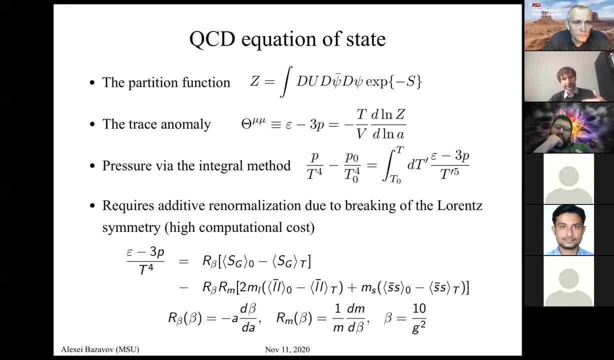 but again we need different sets of of lattices that finer, smaller and smaller lattice spacing So we could have some robust continuum limit. So the end result of this: when we extract the trace anomaly, we can calculate the pressure by integrating it with temperature. 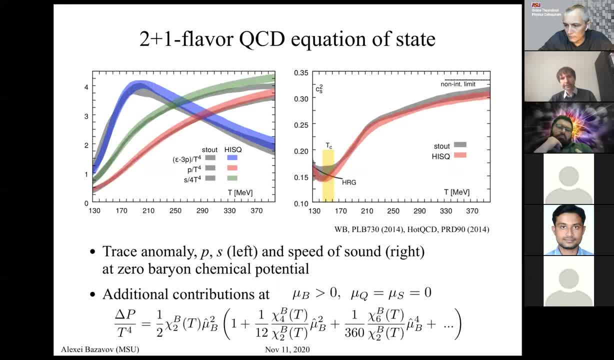 So this requires many, many points to cover the temperature region. So here I'm just showing the final result from 2014. paper was calculated with a Wuppertal Budapest and hot QCD around the same time, So one can get the trace anomaly. 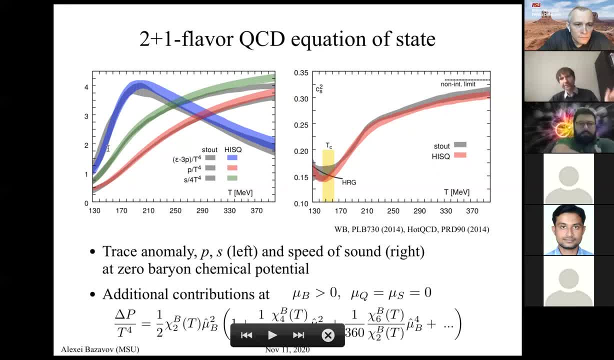 Now it's, it's a already. what is shown is a continuum result after final analysis, with all this statistical, systematic errors, everything folded together in the continuum limit, And then out of this quantity, by integration, one can extract the pressure, entropy, energy density and other things. 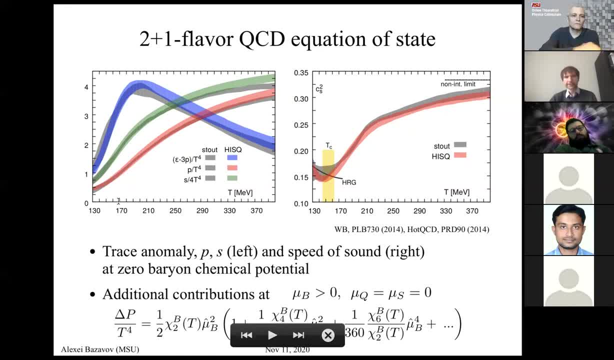 So this is another look at the deconfinement, because this rapid rise in the pressure in the transition region tells us about increasing the number of degrees of freedom. So I have say this variance in this nuclei in heavy ion collision, where all the quarks are confined. 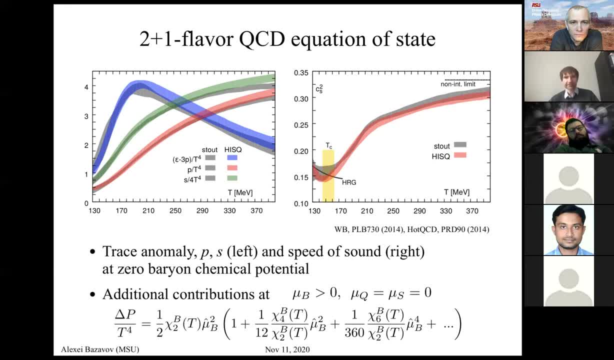 but then in quart long plasma face they're sort of liberated, move around and give rise to the pressure And then this is all at zero chemical potential. but using this as a baseline, by using the method of Taylor expansion in the chemical potential, 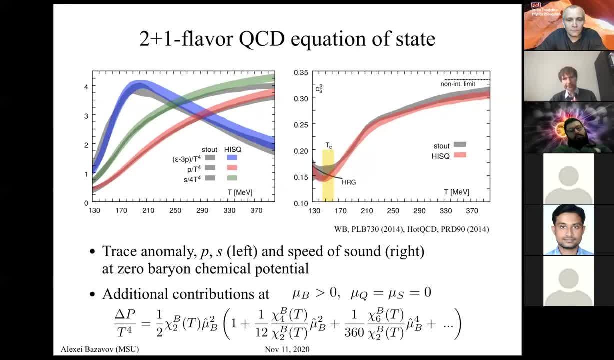 because, as I mentioned before, we cannot directly do lattice simulation when the chemical potential is non-zero, because it immediately breaks down all the Monte Carlo. So the backbone method for all this just simply doesn't work there. However, close to the temperature: vertical axis on the QCD phase diagram. 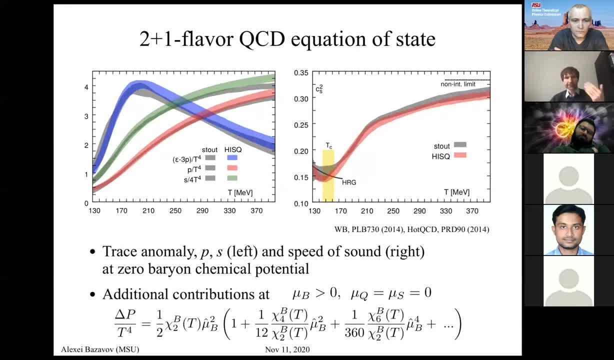 because still do an expansion in quantities like new over T treated as a small problem. So this is a very important parameter. It requires calculation of many, many operators in this for the expansion at high orders. but the end result: one can calculate all those quantities. 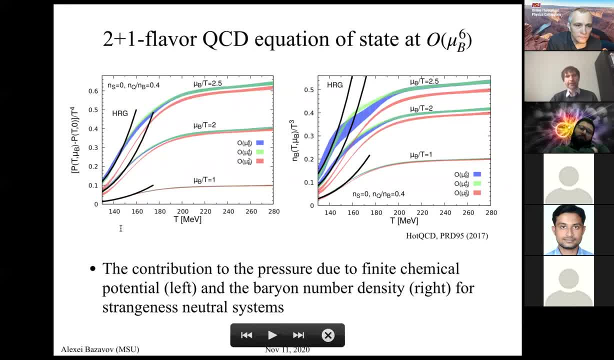 I'll I'll skip through quickly the end result that we can calculate the additional contribution into the pressure. So this is a difference between pressure at some finite bearing chemical potential and zero bearing chemical potential. So it's again, it's a difference between the temperature. 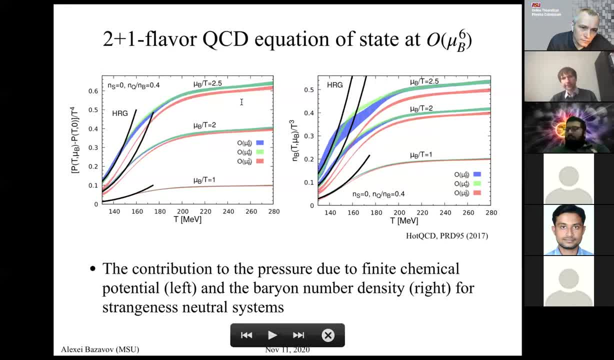 but now you can sort of look at snapshots at different bearing chemical potential layer And so combined it provides the equation of state at finite temperature and finite density and let what can be used as as one of the inputs for hydrodynamic modeling for this realistic heavy ion. 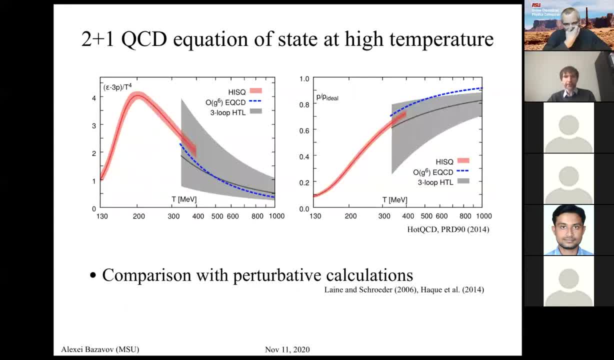 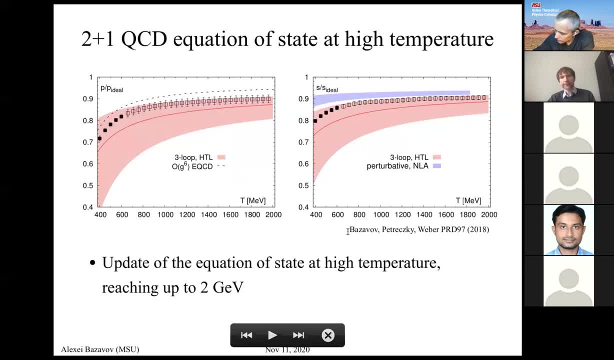 collision problem. So Len recently- again, I'm skipping some parts- but another work was done outside of what QCD and Johannes Weber played crucial role in. there is extending the hot QCD result to much higher temperatures, up to two GV, And the reason to do that is mostly theoretical because this is a two. 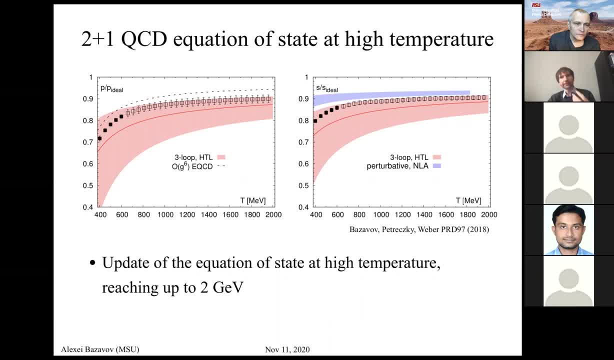 plus one flavor equation of state, meaning that we're not discussing dynamical charm work in here yet. So in the real world there will be contributions from left. at this temperature, However, it's very important to understand theoretically where lattice can be. 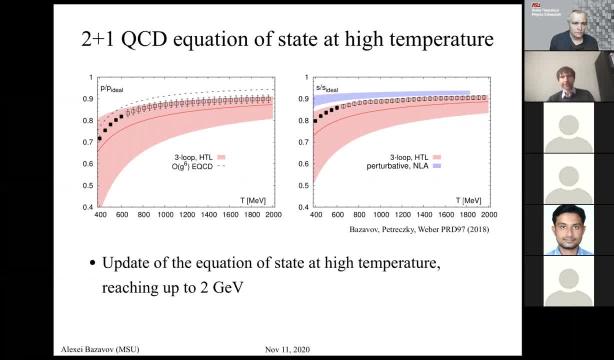 connected to weak coupling expansions, because this quantity, due to the renormalization, is extremely expensive to calculate on the lattice And it's becoming more and more expensive towards high temperatures due to subtraction of these divergences that I mentioned. So this means the lattice calculation is first principle. 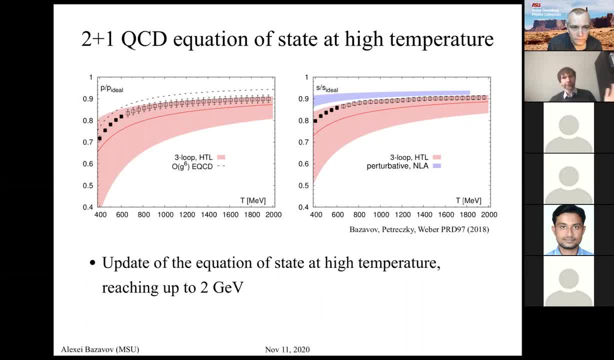 everything is nice, but it cannot be pushed too far. So this is already something that we don't have full control over the continuum limit. So we rather call it a continuum estimate, where we don't have all the cutoffs available to really do the extrapolation. 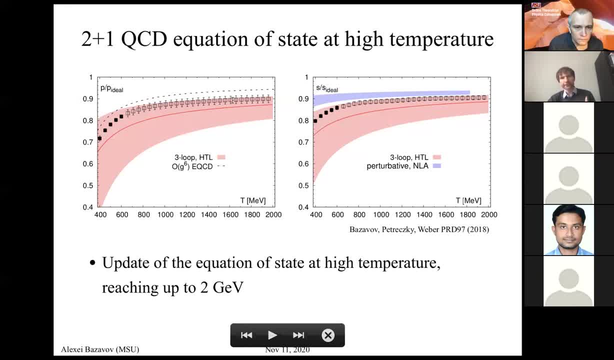 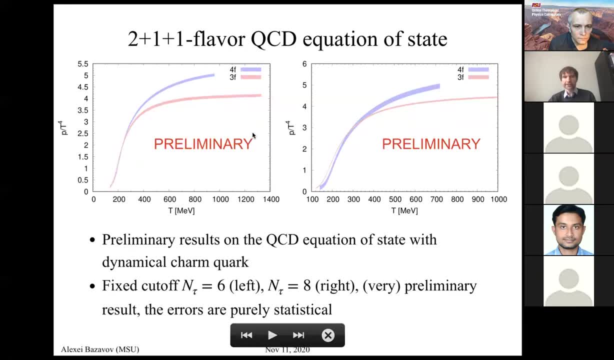 but we have some reasonable idea what the cutoff effects are, So we can assign some systematic error to this quantity. So now what is new for us Is a calculation of the two plus one plus one flavor equation of state. That's a project has been ongoing for a while now. 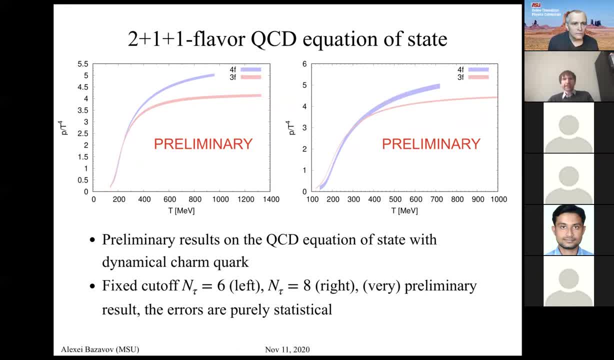 but hopefully entering completion phase is a contribution of the dynamical charm which becomes important at temperatures on the order of 300 MeV or so. So, although its mass is around 1.4 GeV, so it's on one hand, very heavy. 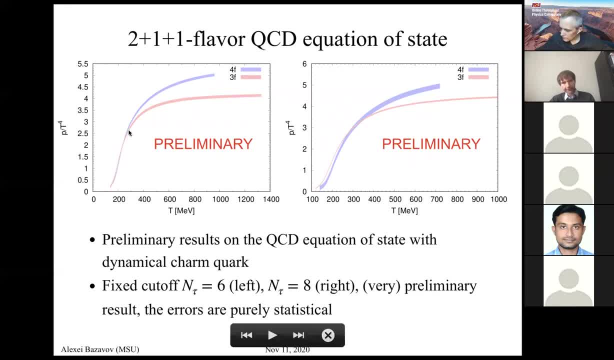 However, it starts to contribute to the equation of state. but it's only one. Now. this is not going to be the first calculation. It has already been done by by Wuppertal, Budapest collaboration, So- but it's the only one for now. 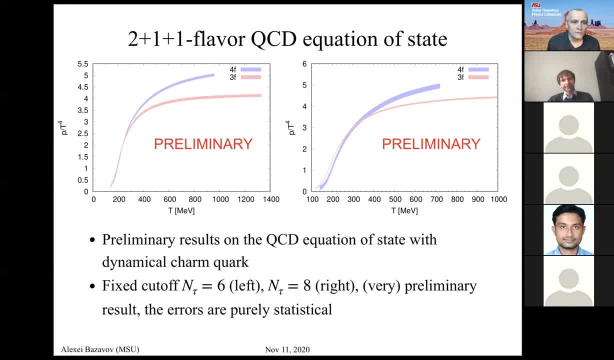 We want to be able to cross check, compare and have our own. So what I'm showing here is just the results at very coarse cutoffs. So that's the smallest lattices that we have in tau six and eight, So this means they're very coarse. 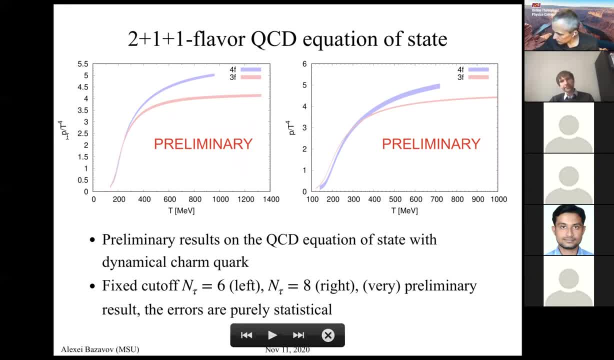 And what's compared here? this pressure not in the continuum limit but at that fixed cutoff between the three flavor results that I showed before, which we fully control, understand now- and the four flavor result. So these are purely statistical errors. 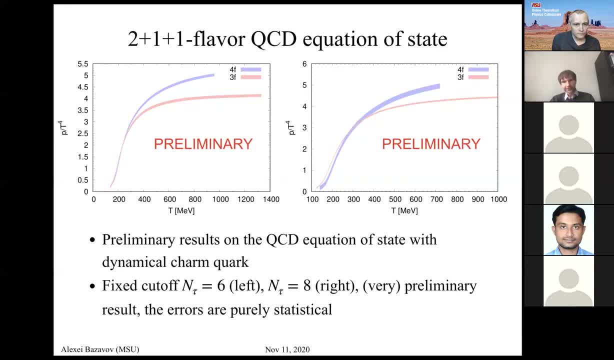 There are a lot of systematics that will need to be considered and folded. in the final analysis, We need lattices with with large and tau so we can really control the continuum limit. but it's shaping up. That's exciting for me. 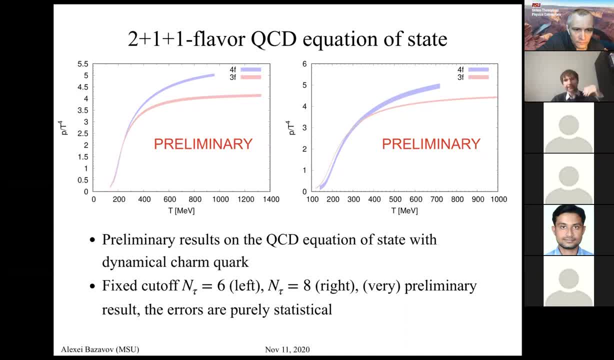 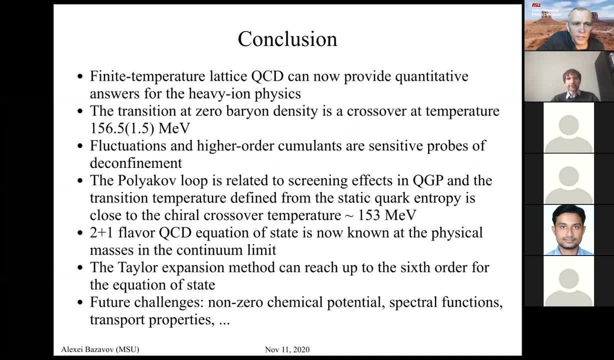 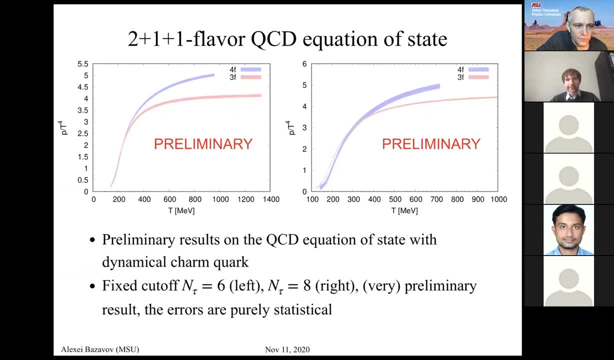 That's, the project is entering completion state and we can have the full real world equation of state with with a charm core contribution. So let me let me conclude Quickly- Yes, Quickly, about the two figures. What was the difference between them? 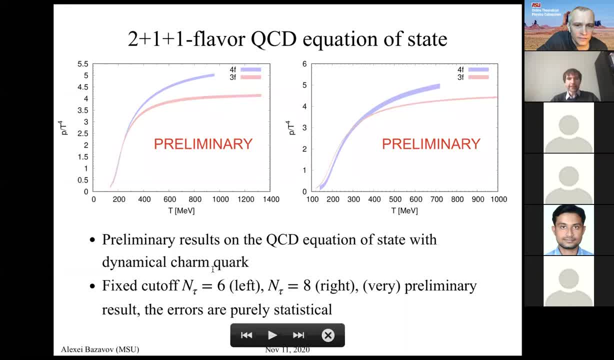 Both pressure, Both pressure, but at different lattice cutoffs. So in other words, the left hand side, it's coarse lattices that cover the same term Temperature range And the right hand side is finer set of lattices. 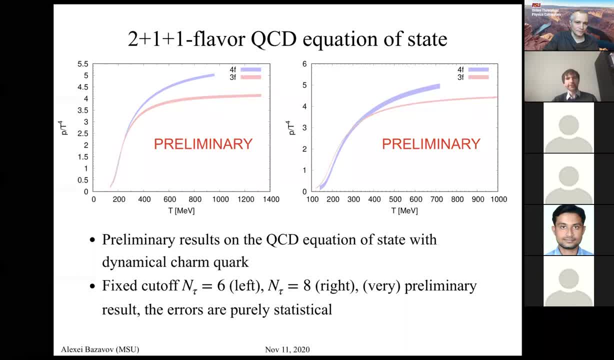 which cover the same temperature range. What we will need to do when we have two more- like in tau 10 and 12, we will need to extrapolate at fixed temperature to the continuum limit. So we could imagine like there are four curves here and I'll six. 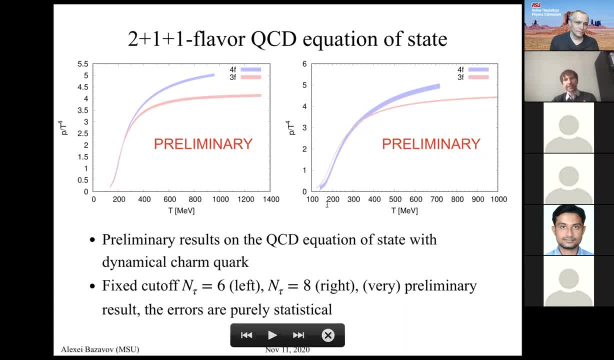 eight, 10,, 12,, and then we take an extrapolation where one over and tau squared goes to zero and tau to infinity, And that would eventually provide some continuum curve. Okay, So that's why it's. it's a very 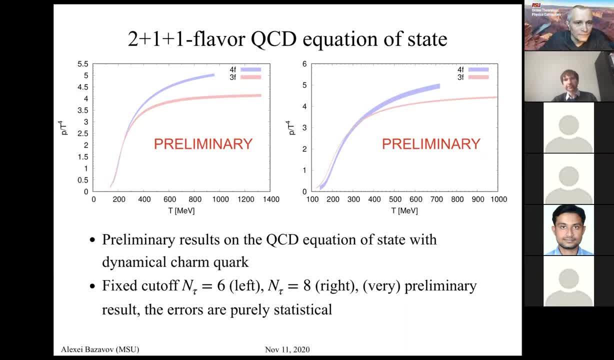 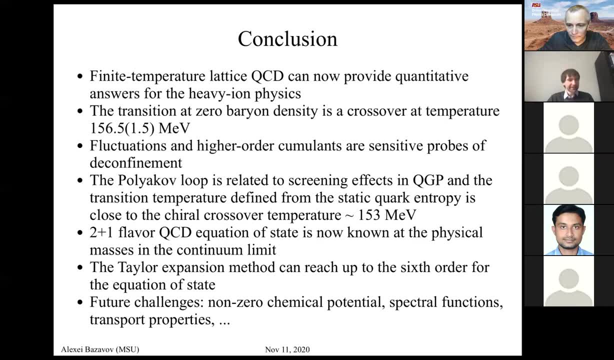 very preliminary threshold. You know the press, So I'm out of time quite a bit. So, as I said at the beginning, do not want to test your patients in in this new zoom world. So let me conclude. There are many things which 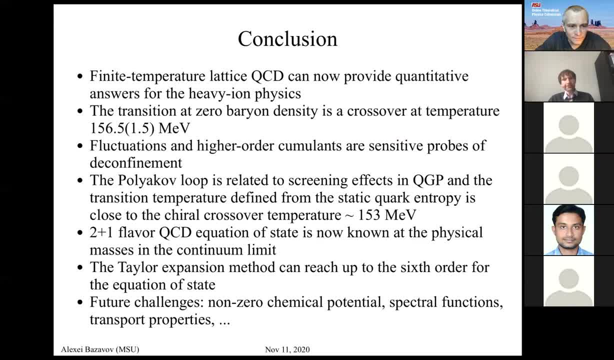 Now at the stage where lattice QCD at finite temperature can provide really Quantum, But- and I I want to go back to So, basically, This is a very, very quantitative description. That was not the case 10 years ago. 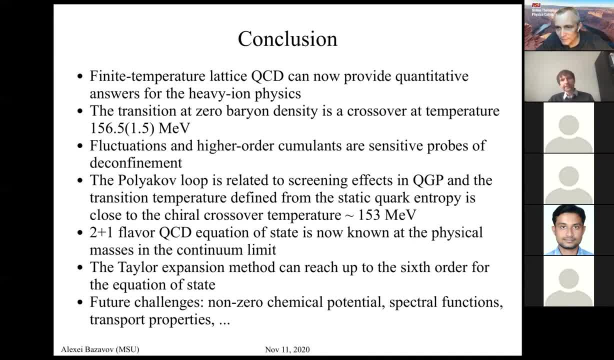 So it improved due to using these improved actions. How great it is. A lot of theoretical and computational improvement then Brought us to this point. We had a recent update of the chiral cross: lower temperature with much more control over the continuum limit. 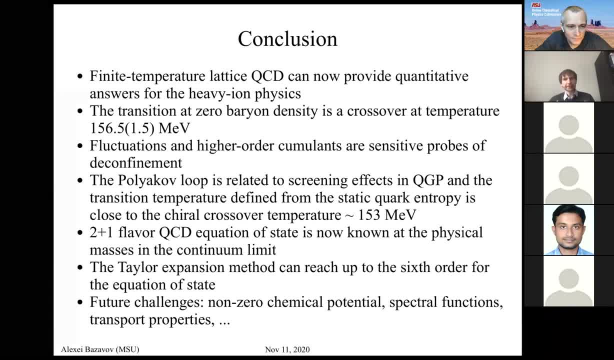 With this expansion, said finite density, which provides a text or observables, and whoopered out previous results. Everything's consistent. that's great. Now there have been, and still ongoing work on fluctuations and high order cumulants which probe the confinement. 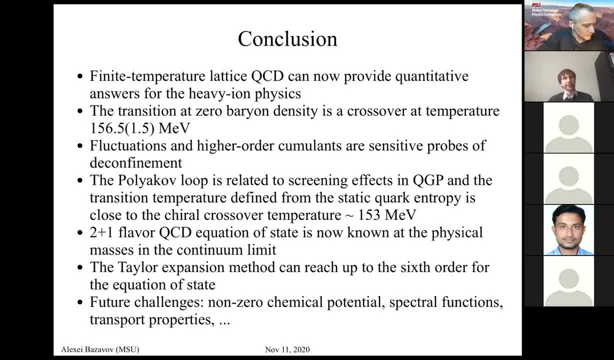 I didn't, I skipped that part, but they can be related to the observables which are extracted from heavy ion collision experiments. So that's also extremely important to provide these results and compare them with what's actually measured in heavy ion collisions. Now the Polyakov loop itself. 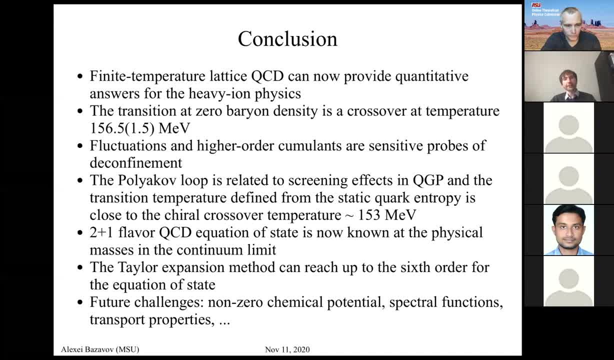 I discussed a little bit as a feature, as a quantity describing the confinement. It's not a measurable quantity but it's related to screening effects in the plasma And if we look at the pair of static work and a quark, we can look at the free energy or entropy. 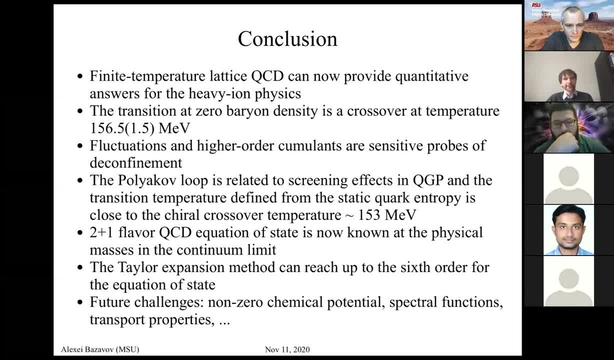 We can also extract the sort of a little bit alternative definition of crossover temperature from this deconfinement related observable and it matches what we observed from chiral condensate and related quantities. The two plus one flavor, QCD, equation of state. 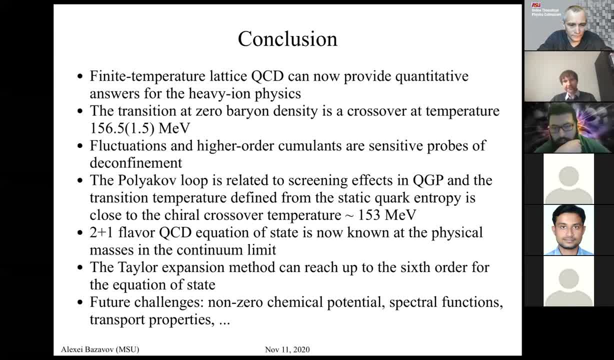 meaning two light plus strange. no, dynamical charm is well-known: full control, physical quark, mass continuum limit. The fourth flavor is upcoming And non-zero chemical potential. origin of the phase diagram is very hard to probe. There is a Taylor expansion method. 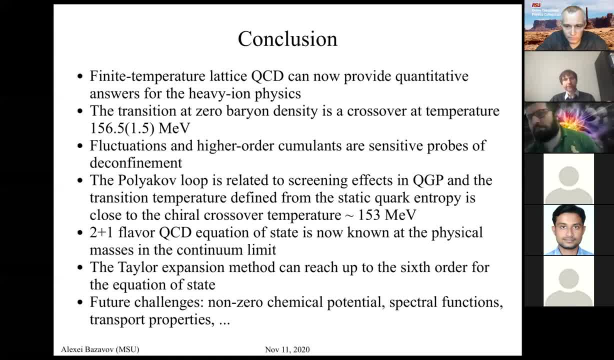 there is alternative method, like used by Wuppertal Budapest. collaboration is imaginary chemical potential calculation. setting the chemical potential imaginary makes the action real. So all the Monte Carlo works again. So it's a very, very nice way of doing that. 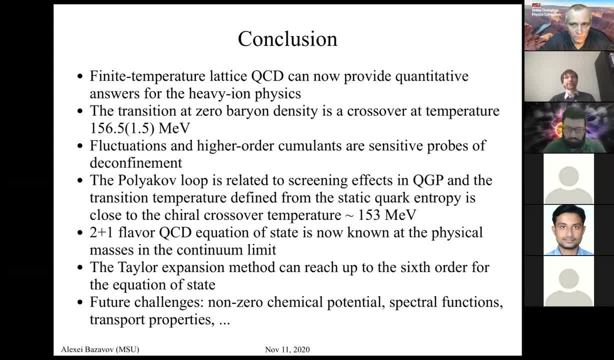 But then the problem is basically shifted to another corner, because then one needs analytic continuation from imaginary to real. So the question is: what is the real chemical potential? That's where the hard part is there, but it's also very robust and reliable method. 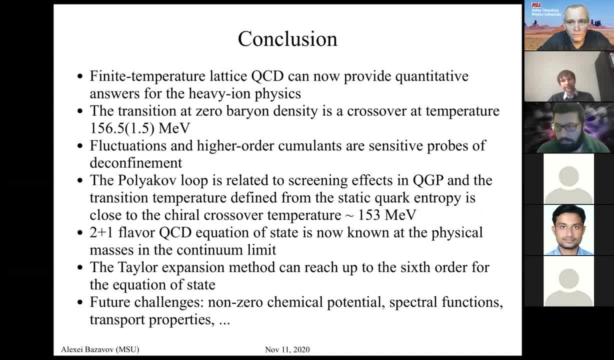 And, in a way, combination of these two, can probably provide the best method, And that remains a challenge: basically finding the critical point on the phase diagram theoretically, or at least showing where it may be or the region where it's not. It's still a challenge, then. 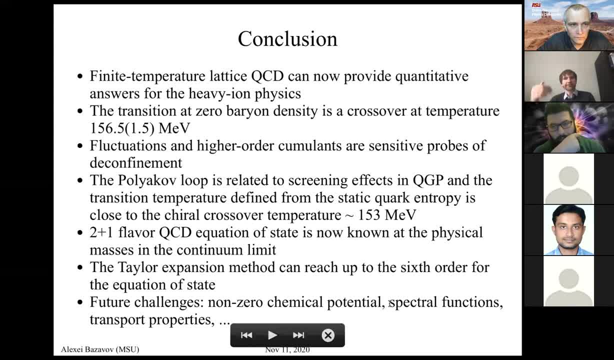 I have not discussed this at all- but the next stages of this finite temperature calculation program. they're related to experiments like S-Phoenix, which is dedicated to study of heavy quarks, And this is also very hard problem, somewhat related in spirit to this non-zero chemical potential. 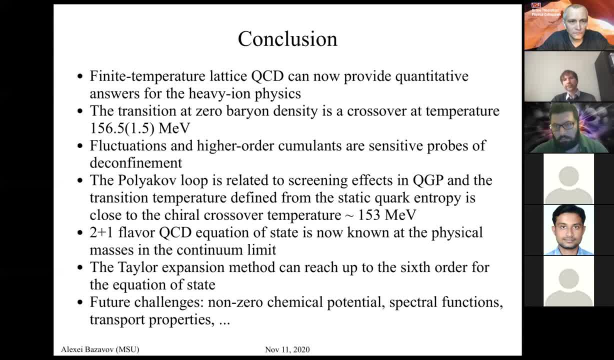 is basically extracting something related to real time Because, remember all this lattice, Monte Carlo relies on being in Euclidean space time. So real time, the quantities are very hard to access but they are very relevant for the experimental program. So on that, thank you for your attention and that's all. 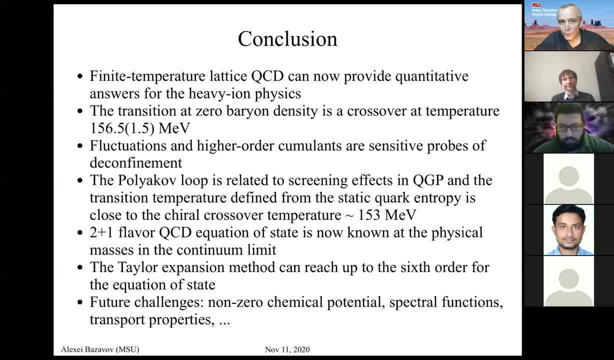 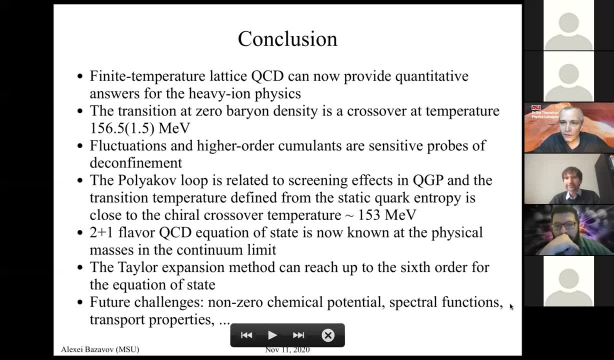 Thank you. Thank you very much for a very nice presentation. Now we have time to go to questions. Are there any questions from the audience? I don't see immediately any. Yes, I do see now. So, Hong Chao, I hope I pronounced that correctly. 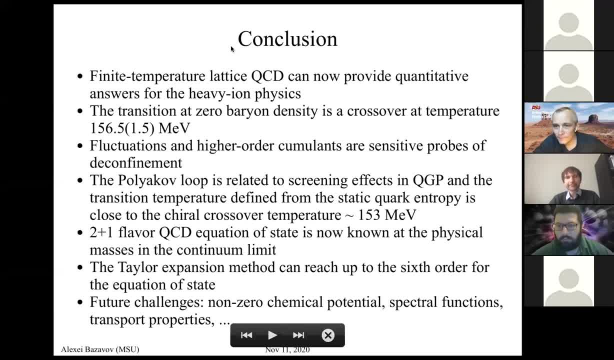 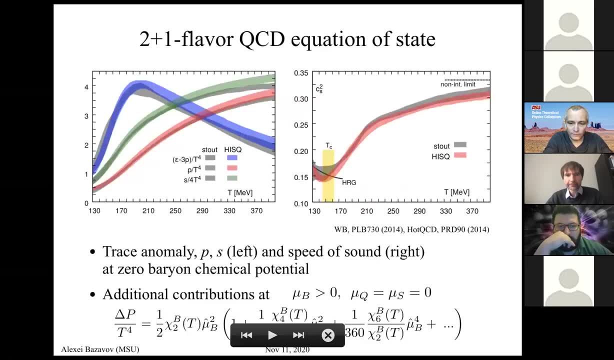 Go ahead, You go first, I think Okay, thank you, Hi. so thanks for the nice presentation. Can you go back to the slides where you showed this entropy, where you get the entropy from the static quark, This one. 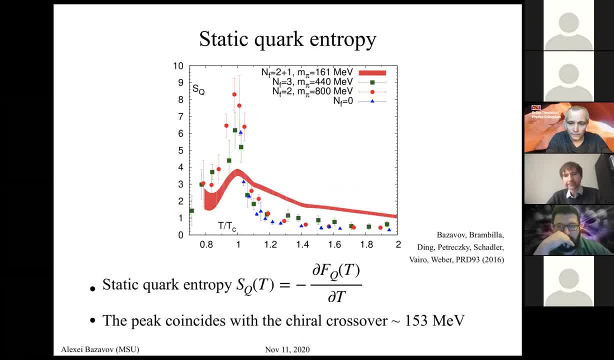 Yeah, yeah, exactly Yeah. so I just wonder so: why does the error grow so much when you're close to the critical temperature? Is it because of the way that you compute the S, which comes from the finite difference, or 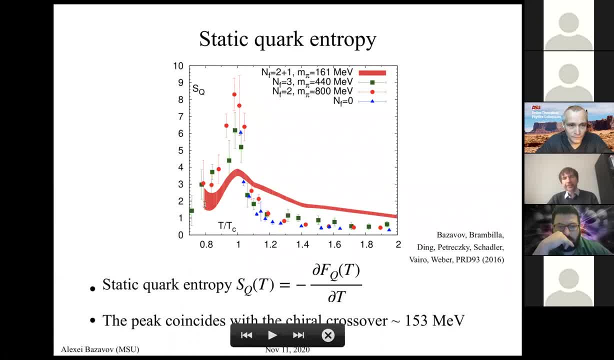 Well, it's more like it's. you know, it's not easy to do the simulations at low temperatures. in a way, There is a lot of statistical noise in these quantities, And so that's manifestation of that. This error folds together two things. 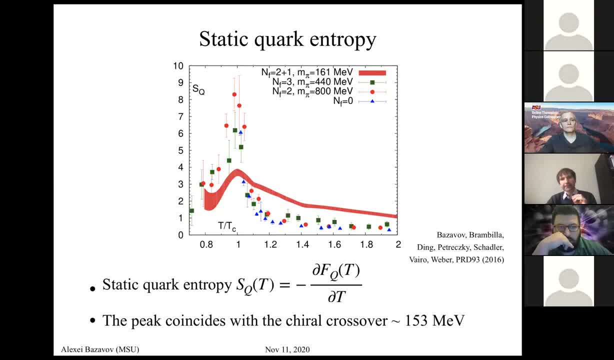 There is statistical error from the fact that you know we're doing Monte Carlo, So this can be beaten by running longer. but essentially you know you have some finite amount of computational resources and you end up with some statistical error And then you have systematic error. 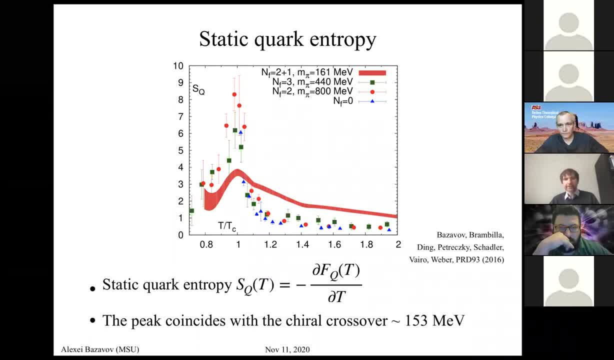 from extrapolating to the continuum limit And so here there is a lot of noise. So what happens at high temperatures you typically have? you know the fields, these gauge fields that we're simulating. they're smoother. there is less statistical noise in quantities. 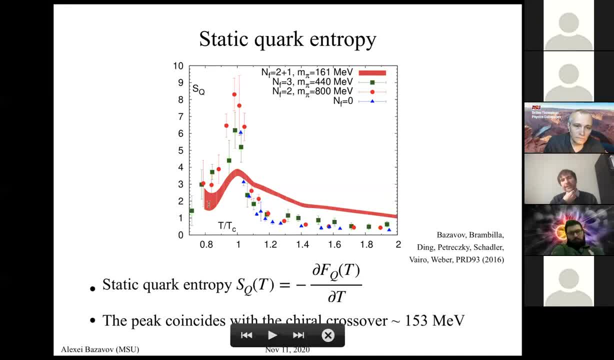 So that's a lot of statistical noise plus systematics of the extrapolation. Okay, so this is not a feature of the fact that we are close to critical temperature, but this just when we go to colder environments, it just happens. Yeah, it's purely technical. I would say. 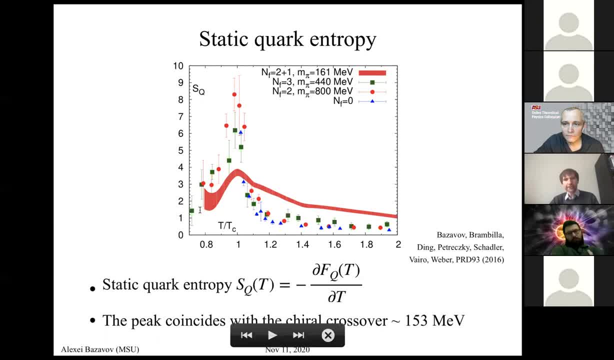 So, in other words, with an infinite amount of computing time, this bend can be shrunk to zero width, right It just. it's not a physical feature, It's just, you know finite amount of resources that we can afford. 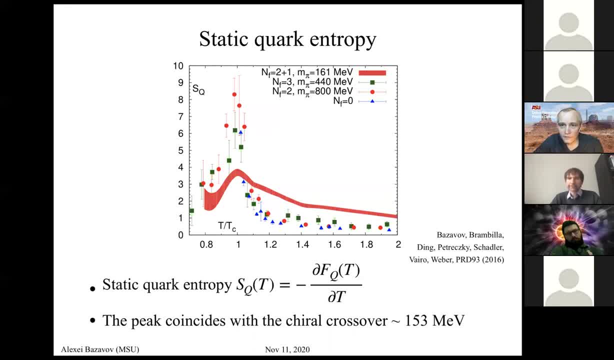 Oh, okay, thank you. Okay, next question, Claudia Ratti. Hi, Alexei, thanks a lot for this very nice talk. I had a question about your second to last slide, just quickly, Where you show the charm result. 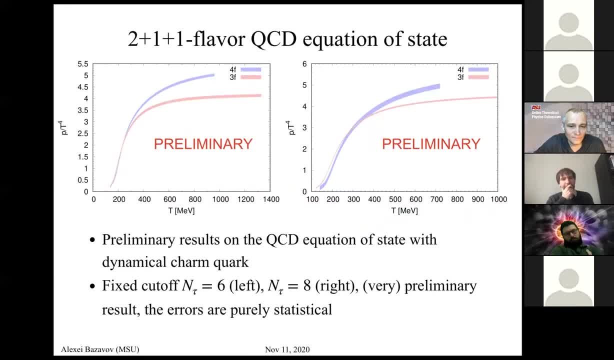 I know you said it's preliminary and it's at finite lattice spacing, but I noticed that on the NT equal six at low temperature you have agreement between three flavor and four, and then at the NT equal eight, the new data seem to be below the previous ones. 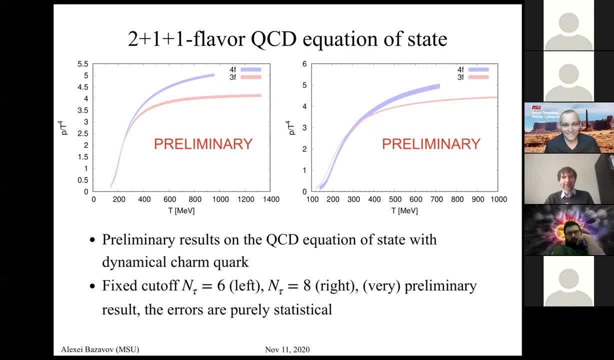 Is that- Very good expert question. Okay, there are a lot of things which are technical going on, but that's interesting to discuss. So, yeah, Because it's expensive to calculate, we are taking a little bit of a shortcut here because we are confident in the three flavor equation of state. 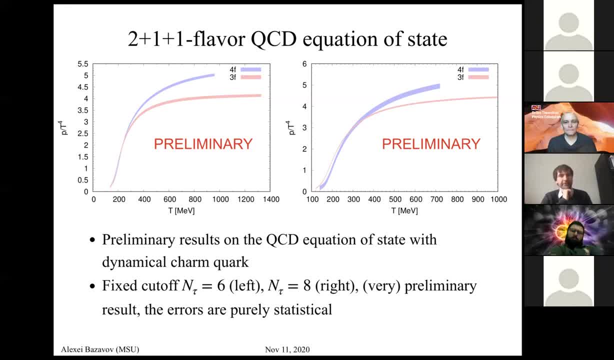 Now we have full continuum limit. So this program is going on the following way: We are actually doing the four flavor calculation and the pion is tuned to be 300 MeV in the continuum limit. So in other words, this is data. 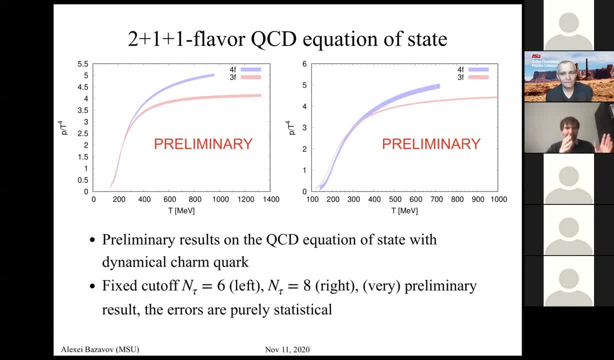 which would correspond to something which is almost like QCD, but with all the spectrum shifted up. And what we intend to do: once we have fully controlled continuum limit, we will stitch it together with a three flavor result at temperatures around 300 MeV. 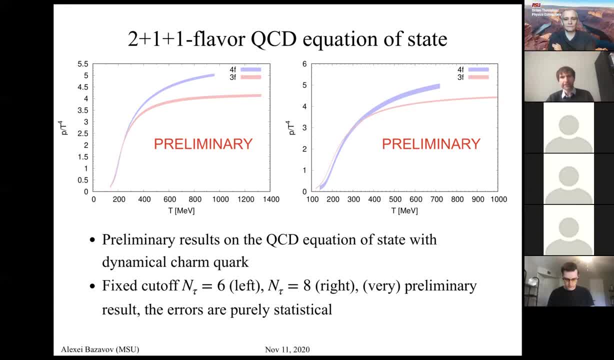 Because at 300 MeV, as we know quite well now, the light work mass doesn't play a role anymore. I mean in a reasonable range. So having 300 MeV pi is not a problem anymore And the charm quark is not yet contributing. 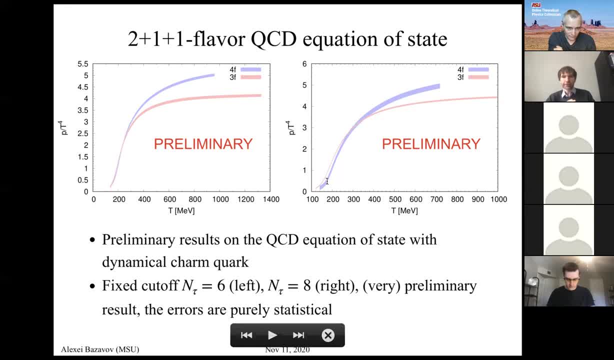 So the difference here is for two reasons. One is it's a heavier pion And as we know from this hadron resonance gas kind of quick consideration, that if you shift the spectrum higher then all the thermodynamics kind of observables will go down. 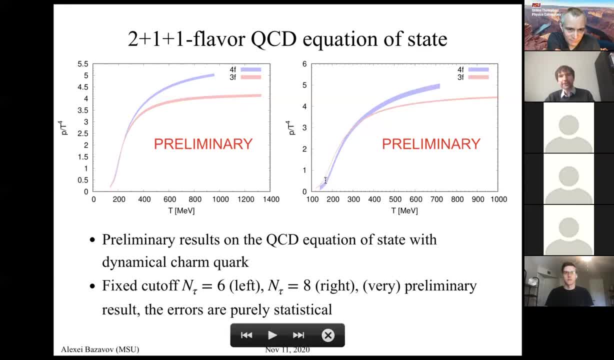 And we still need to understand the cutoff effects which affect both vertical and horizontal axis, Because the temperature scale, as we set it, it also has cutoff effects And we fully understand them in the three flavor case, but we understand them much less still in the four flavor case. 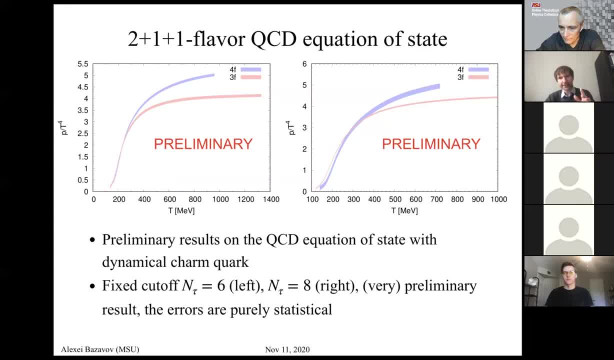 because it's a very different set of simulations, It has a slightly different action also, and so on. So there is a possibility of a systematic error, also in the horizontal direction. So my quick sort of understanding this, it's at least these two effects. 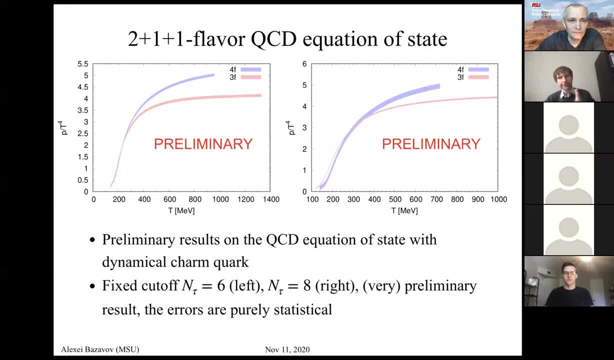 are playing a role here: Heavier pion and uncertainty of the temperature scale itself. Okay, very interesting, Because on the left you don't have it. So I was wondering It's more accidental. I mean, such a coarse lattice is that many things like? 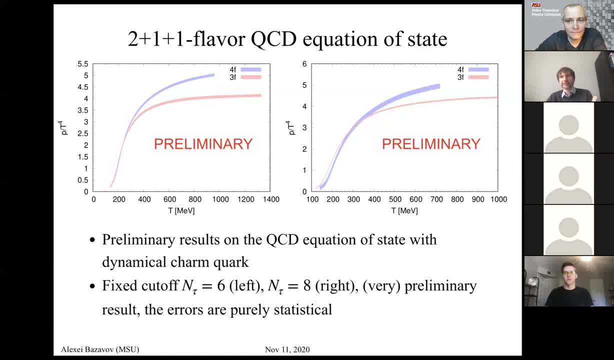 that's one of the things that's, of course you and our collaboration observed over the years that sometimes you know you have coarse data and things work out well. Now you get better data and things break down suddenly because there are, you know, certain accidental cancellations anymore. 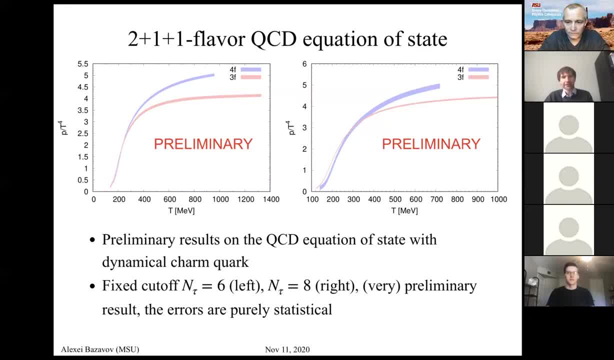 And some things. he didn't previously start to show up, So this is an accidental effect. for now, Thanks a lot. Okay, next question is Kirill. Kirill Boislavsky, did you want to ask? Yes, yes, hello. 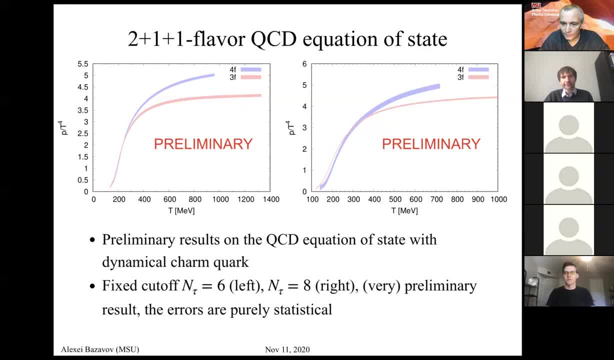 So thank you a lot for the great talk And I have actually kind of general question more or less. So it's actually it's become very usual and very natural that the deconfinement phase transition and the Kirill phase transition are at the same. 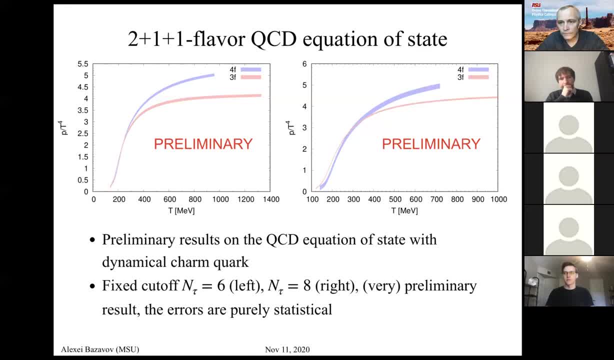 the crossovers are at the same temperature. What happens when you crank up the chemical potential, And especially since there has been already some tail expansion in the chemical potential? has there been any difference in the temperature between the deconfinement phase transition? 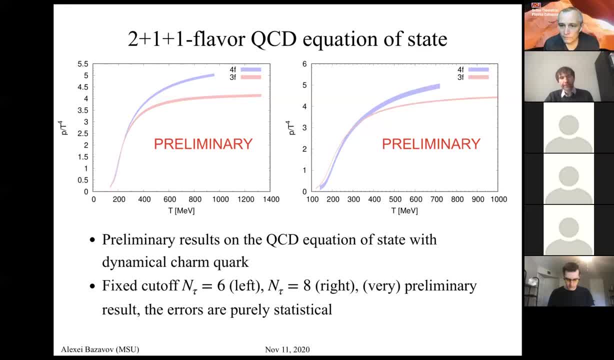 or crossover, and the chemical, the Kirill one. Well, this is something that's being studied. I'm sure I'm not involved on that part. I mean I could talk a little bit about what happens with the Kirill crossover temperature. 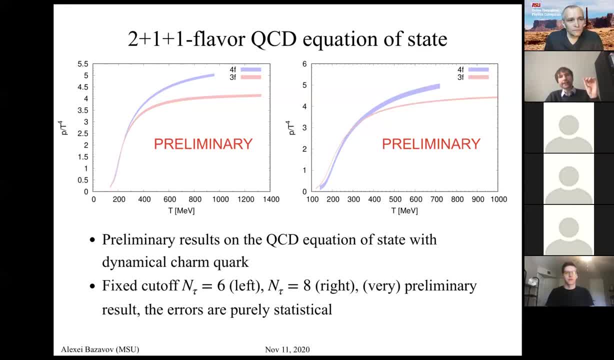 So one could study how the Kirill crossover temperature changes with the chemical potential. And we've done this within hot QCD where you basically can define some curvature coefficients and it goes down as you expect from that phase diagram. Let me read them there maybe. 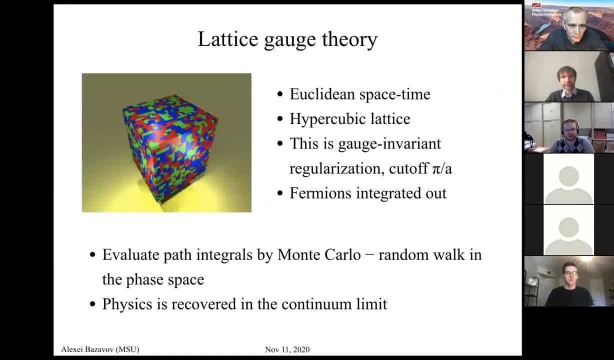 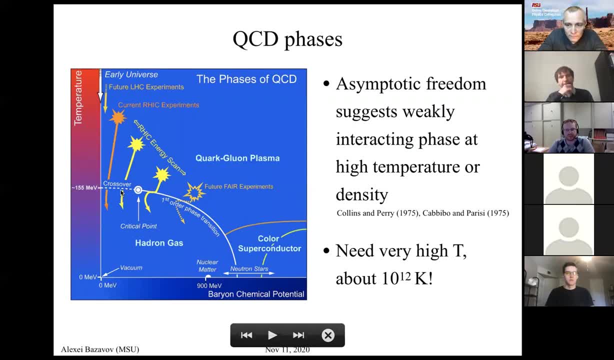 So the question is: what does Polyakov loop do in that regime and how things may be compared? So maybe Claudia can comment if Uppertal looked into those things. So this is an interesting question. It's just not something that I looked into. 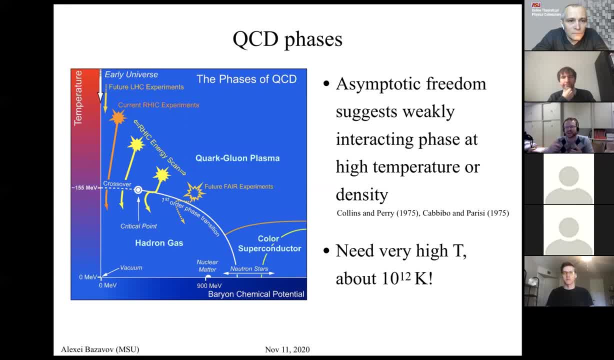 Sorry, I thought because you were talking about tail expansion, So kind of in both observables this has been done. Well, it has not been done for the Polyakov loop And it's one of the sub projects that were sort of at the back of my mind, but it's not the highest priority. 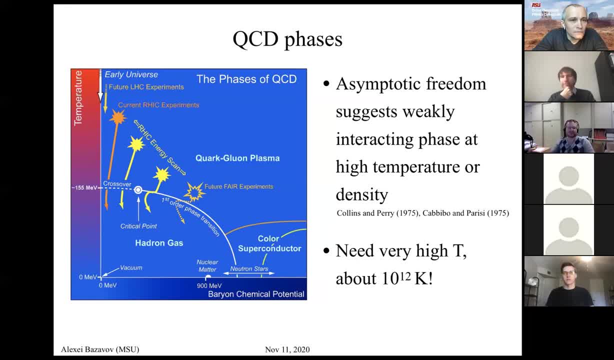 But in a way this is actually something. it's a project which require less computational resources but more human resources to actually do that work Because, as you very rightfully point out, in a way all the data is in there, So one just needs to really do the analysis. 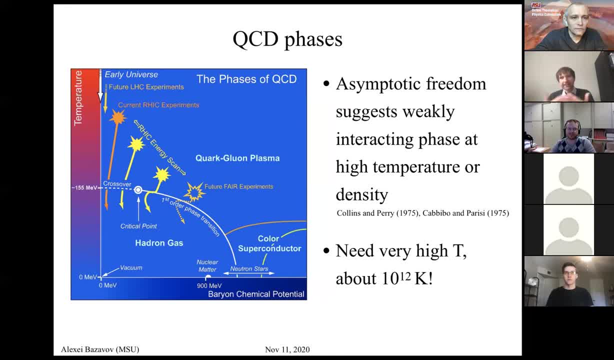 because we have the Polyakov loop, we have the Taylor expansion and then you basically fold things together in that expansion and study that stuff. Okay, thank you. Okay, next question from Jean-François Paquet. I'm hoping I'm pronouncing it correctly. 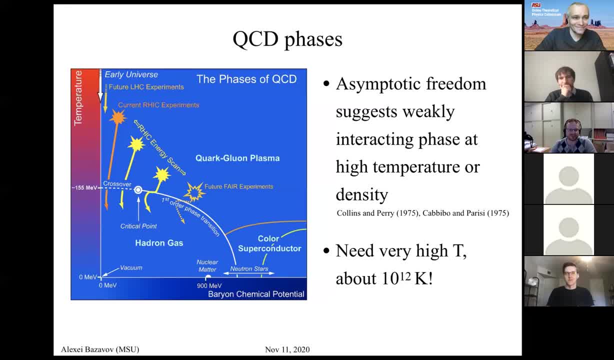 It's leading order. Thank you, Thank you. So often in heavy end collisions we need to know how to transition from a fluid description to a hydrogen as gas. So the problem that we have is not so much that we don't know the equation of state. 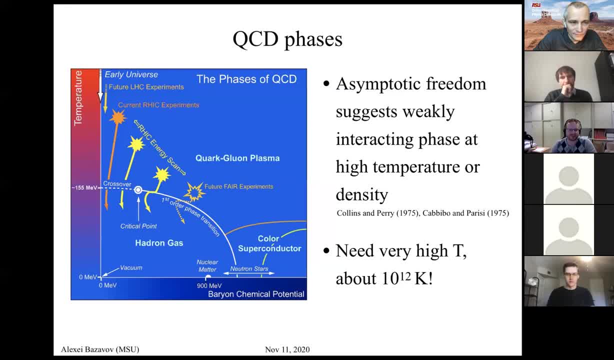 but that we don't know exactly how to do this matching between the lattice calculation and the hydrogen as gas, And I get the feeling that often improvements are mainly trying to improve the hydrogen as gas until you can match the lattice. But I'm wondering if there's any insight from the lattice. 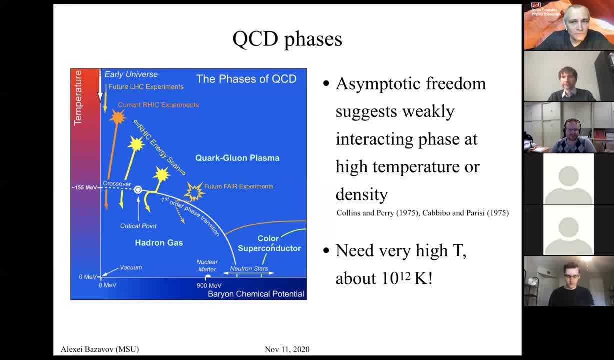 that can be used to better understand the hydronic thermodynamics, If there's some way to- I don't know some way- to better understand this matching. Do you understand my question? I understand your question And I could say I'm certainly. 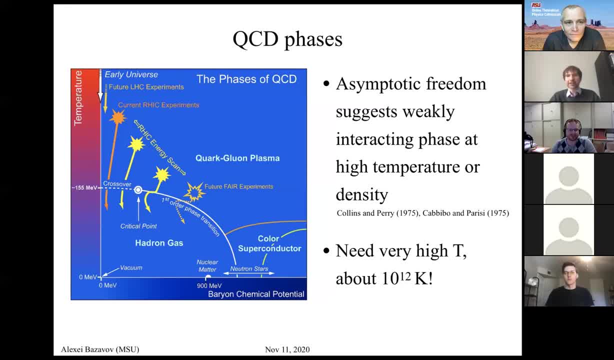 not an expert in this part, because that's why one of my disclaimers is that all I showed to you is basically infinite amount of matter in thermodynamic limit, in equilibrium right And- Even in that case. even in that case. 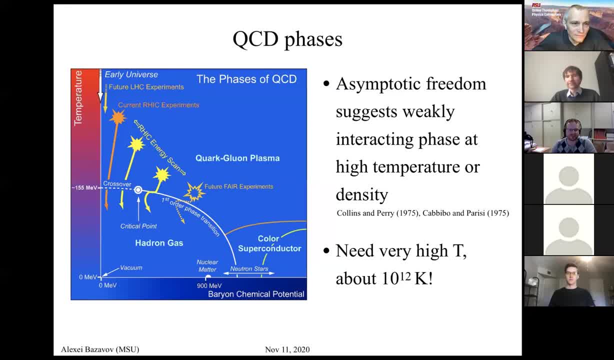 technically we don't. I don't know if we know how to exactly match the hydrogen as gas to the lattice calculation, even if you're in this infinite thermodynamic limit. There's a continuous attempt, I think, to improve this matching. OK, I was just wondering if you had any insights. 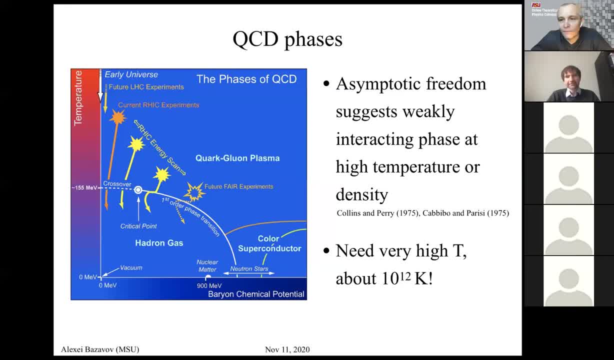 I personally no. OK, Maybe I can say something to that. So I think for the thermodynamics the matching is pretty good. I think the continuous attempt to improve from the other resonance guys side of things comes when you go and do look at more differential observables. 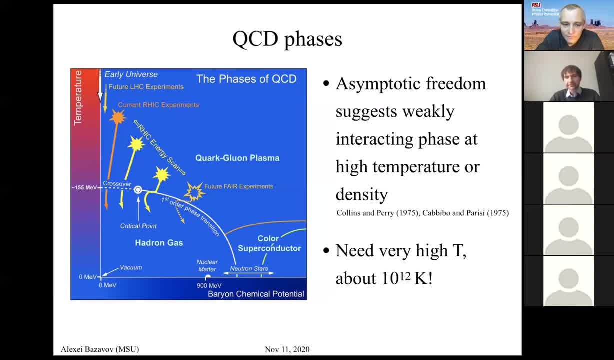 like higher order susceptibilities and off-diagonal susceptibilities. There you really see that maybe just the standard HRG model with a spectrum which is just the PDG observed spectrum is not really enough to really match all of the observables, But for the equation of state alone, 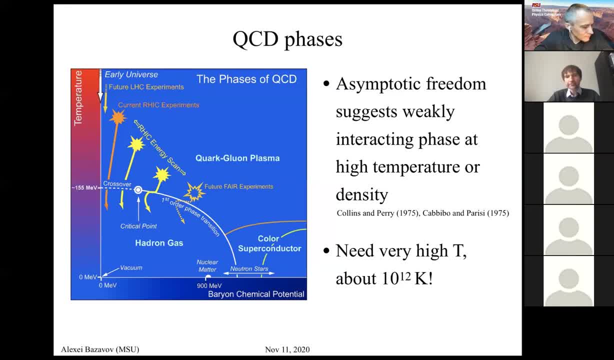 that's. I've never seen any problem in matching the two. I mean it's pretty good. I mean, as a hydro practitioner it's pretty good. But even if it's a 5% discrepancy, which in a sense 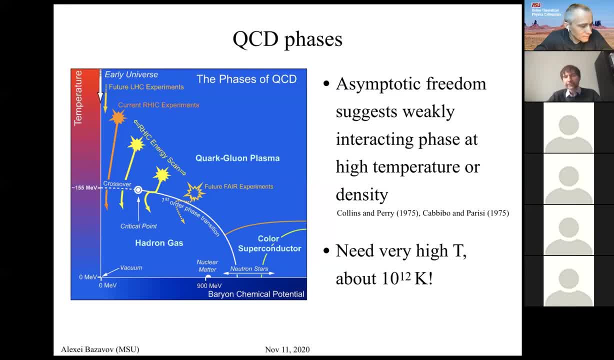 is excellent agreement between the two. it's unclear if the effect that we have in our hydro simulation is that small. Somehow you need to force your equation, your hydrogen resonance gas, on your lattice equation of state. OK, I was just wondering. I don't want to harp on too much. 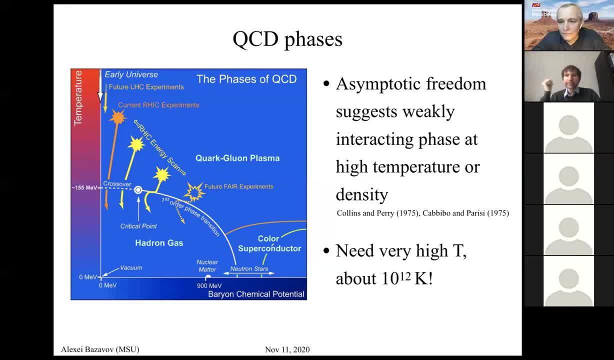 Thank you, Claudia, for the update. Thanks, Claudia, Maybe a quick comment. I mean, if you're interested, of course, in some bulk observables like equation of state and so on, then we could see where it matches resonance gas and so on. 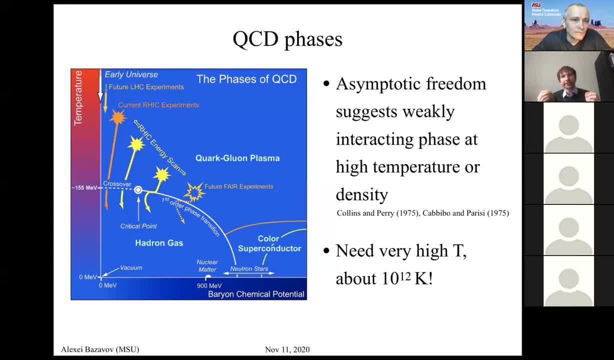 But I was under the impression you need more than that, right? Because you have this fluid and then you have this surface where it starts breaking up. You partition it into cells And then you have to decide how to turn this fluid into particles and stuff, right? 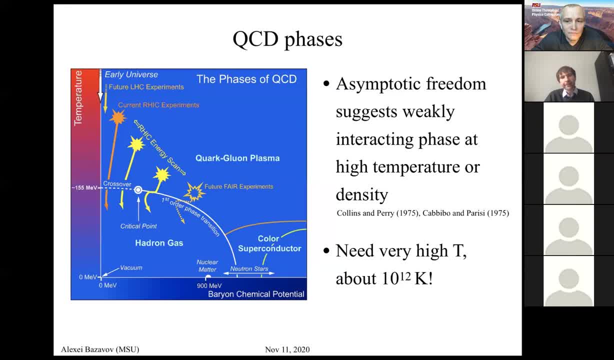 I mean technically speaking, we have both problems. I mean, the one you're describing is arguably much worse: trying to find exactly how to transition from a fluid to hadering degrees of freedom, But even at the level of the equation of state. 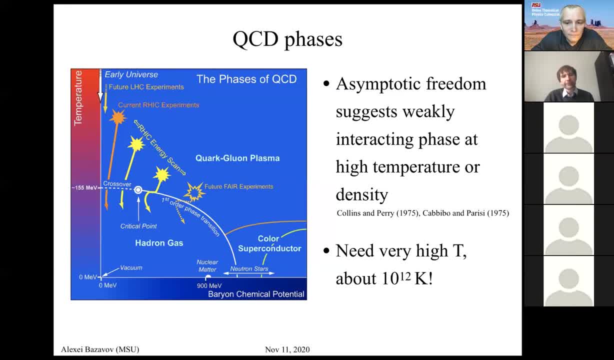 we keep having this pesky problem that we can match it. It's pretty close, But you often end up having to force, for example, the speed of sound of your hydrogen resonance gas, the speed of sound of your lattice calculation. It's not big, but some people think it's enough that. 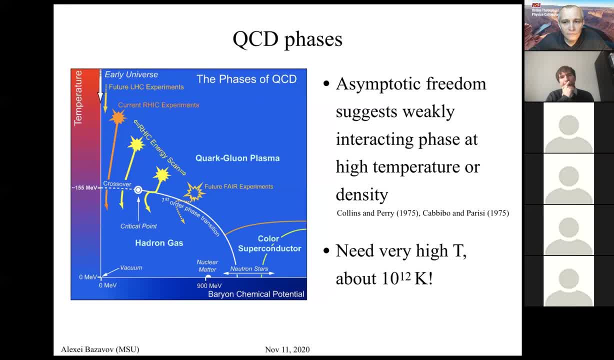 it affects more description of data actually. So I was just wondering. Yeah, thank you. OK, I don't see any other questions from the audience. I had some sort of several naive questions on my own. One of them was actually related to this mention. 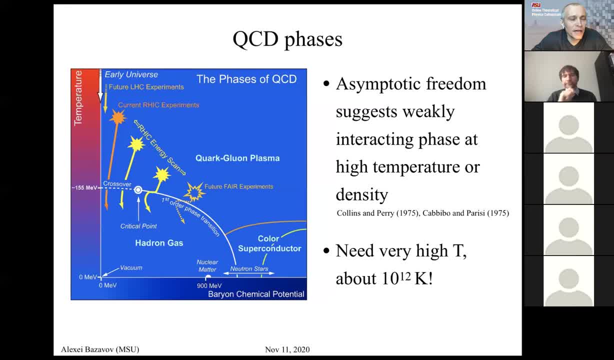 how you approach the continuum limit and the light pion mass. If you try to approach the light pion mass of order, let's say 140 to 100 MeV, then basically the corresponding de Broglie wavelength of that is essentially of order, just slightly more. 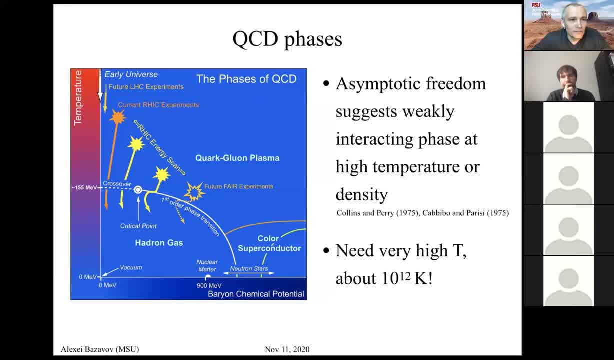 than 1 Fermi, or maybe like 1 and 1 half, maybe even well, yeah, 1 and 1 half is about for 140.. Now, if you are going to consider the physical lattice of the size of only 2 Fermi, it seems to be that barely. 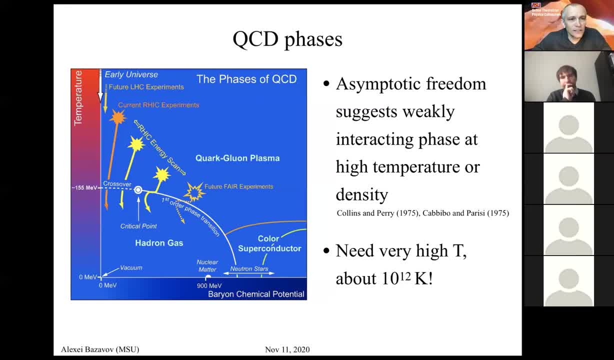 any de Broglie wavelength of a pion fits there. Isn't that some sort of big problem in there? Well, in a way, I mean, what we want is typically that m? pi times l is something like 4,, 4, 5.. 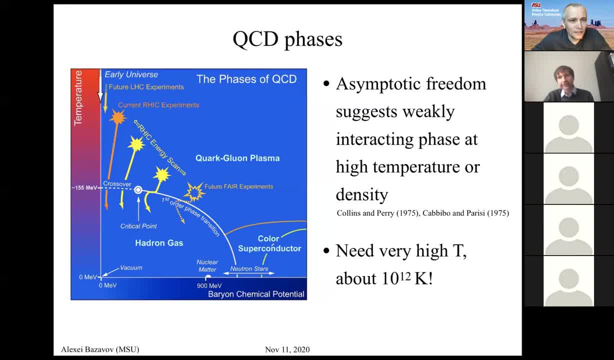 I don't seem to get that right. Right, If you take l, you said 2 Fermi, You're taking more than that. I'm sorry, Maybe I'm missing something. Well, it depends. That's why we have different boxes. 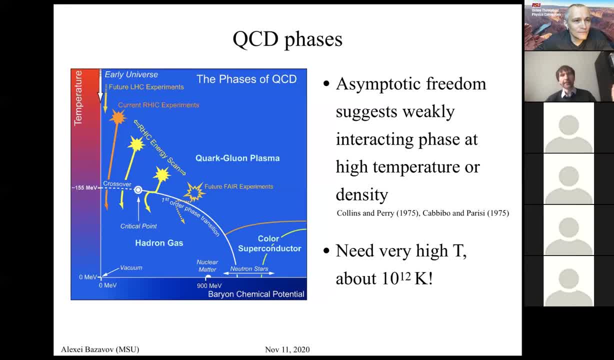 depending on what pion masses we're trying to simulate. But what is typically argued is that when we have these boxes with spatial periodic boundary conditions, then finite size effects enter as e to power minus m, pi, l or so, And so we want them to be suppressed. obviously. 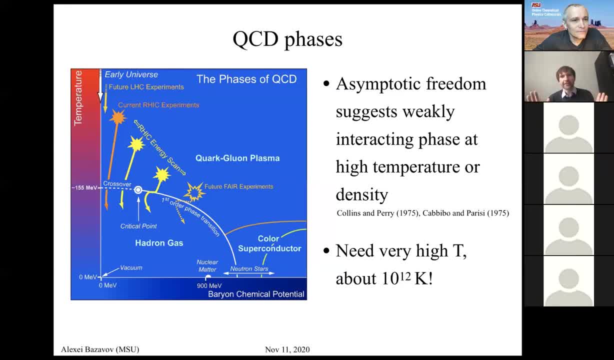 But then OK, we cannot afford to, It's too large. So the typical sort of common wisdom is that we take m pi? l around 4, and that's good enough, Because, in a way, one thing here is that we have many, many sources of systematic error. 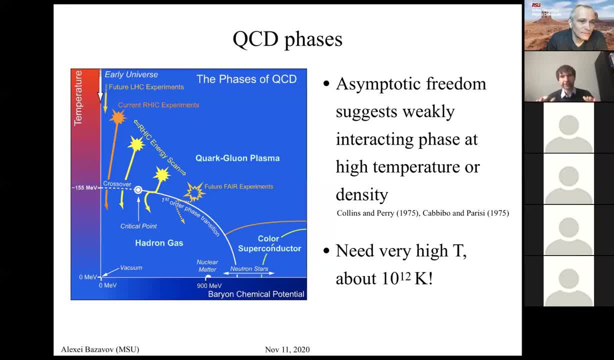 and statistical errors on top. So typically you want them all to be comparable because you don't want to improve something too much and put a lot of effort, but then it wouldn't be seen because of all the other errors, And so that's typical boxes that we have. 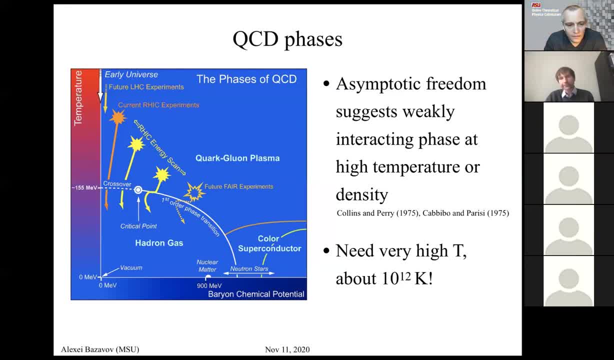 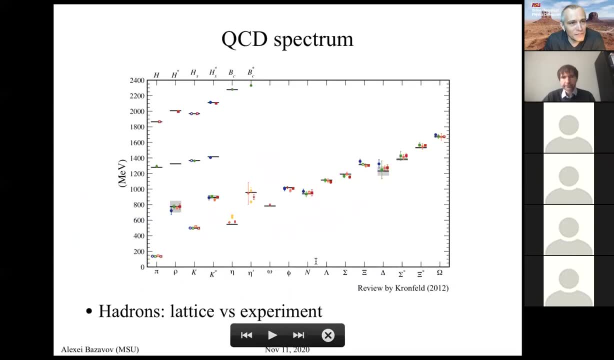 So m pi? l on the order of 4.. OK, and the other thing was kind of related to one of the statements that you made on, I believe, on the last conclusion page, saying about potential exploration of time dynamics processes, So in real time. I thought that was like a taboo. 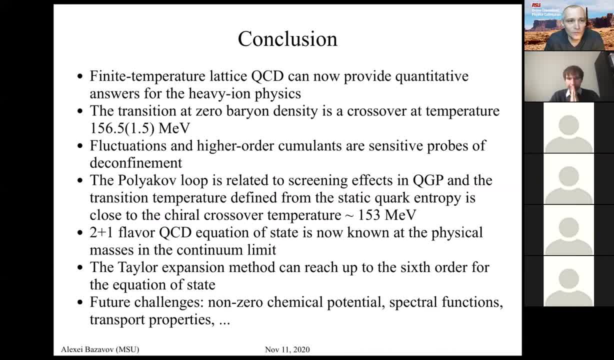 You cannot go there at all. Is there some new ideas that might help you to understand some dynamics, actual time? Well, I would say the sort of more accurate statement is not really the dynamics, but rather some quantities which are really sort of like real time quantities. 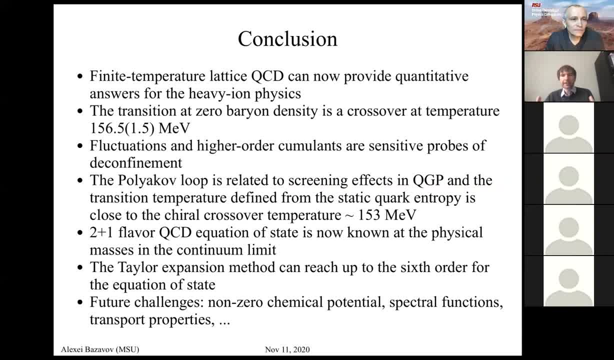 Because, for instance, why we're interested in the spectral functions for heavy quark-1 and so on. So we could sort of have it, We could have a description of how those things change with temperature And we could make some sort of quantitative statements. 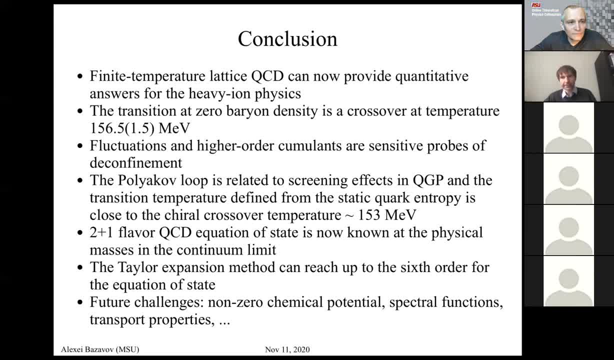 which states are still present at different temperatures for this S-Phoenix kind of program and so on, And those are essentially Fourier transforms of the correlation functions in real time. However, in Euclidean spacetime we have only this Euclidean correlation function. 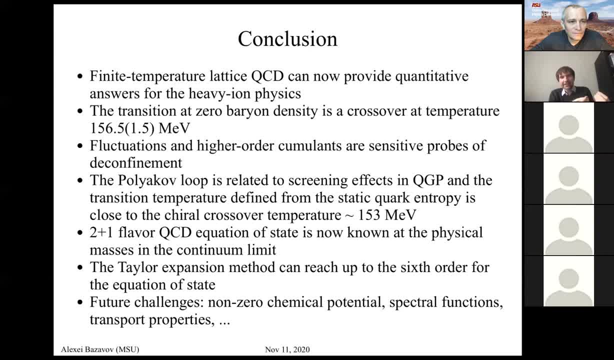 So then this means the spectral functions. it's really something which I consider a real time thing because it's very differently related to correlation functions. in Euclidean spacetime We have some sort of Laplace transform and so on. So, in principle, all the information is there. 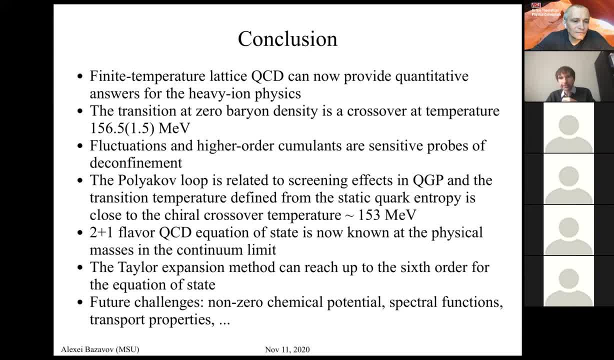 but it's just becomes such a hard inverse problem that it's almost impossible to solve in a way, And I mean some improvements can be made by, you know, having more data, more quality data. As you know, there is a lot of work related. 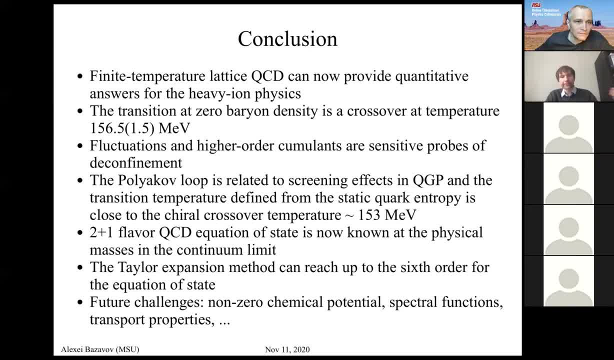 to spectral functions with this inverse problem, Bayesian methods, all kinds of things. So this is something that you know, new methods or not, but it has to be approached And so maybe with some incremental improvements, Similar inverse problem with the transport properties. 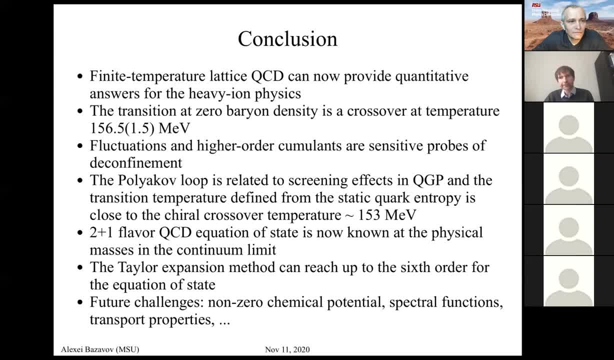 like this. It's even harder than this Clark-Koenig spectral functions because it involves gauge absorbers and those are much more noisy on the lattice. Those mean the statistics is horrible, and so on. So when I made this statement, it's basically: 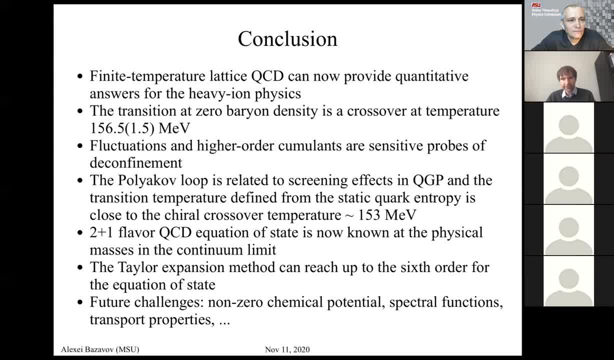 it's just the next steps that we have to be addressing anyway, And maybe with marginal improvements for now, Of course, if you noticed, I mean a lot of lattice community is interested in quantum computing now And typically the narrative is that it can address problems. 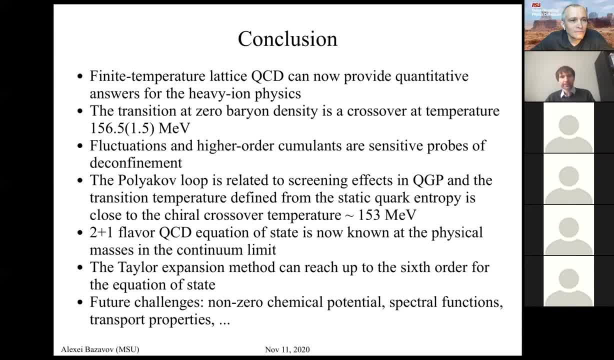 which are exponentially hard, because in principle we could work in Minkowski space time, but this means having that problem which complexity scales exponentially with a number of degrees of freedom. So we just give up in a way, right With the usual approach. but then maybe it was quantum.